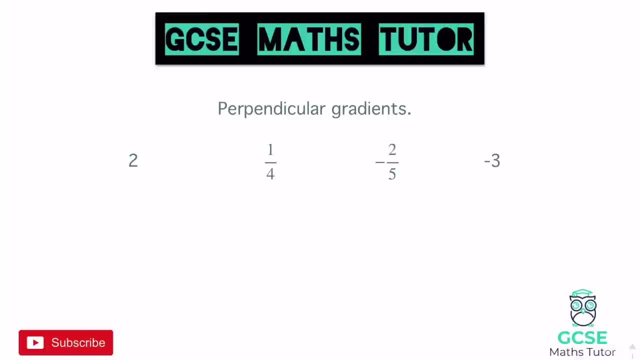 in this series looking at equations of lines. You're going to have to have a very good understanding of that. Again, the link for that is in the description, so check that one out first if you haven't already. but we're going to get started. So grab a piece of paper, grab a pen. 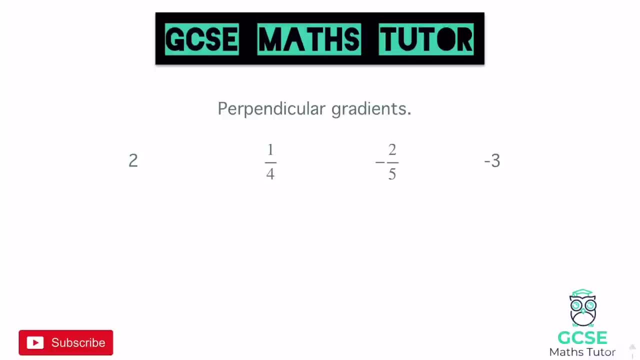 make some notes and we're going to start by looking at this question here, just looking at perpendicular gradients. So on the screen I've got four separate gradients. I'm going to have a look at creating the perpendicular gradient of these. So the first one that I'm going to have 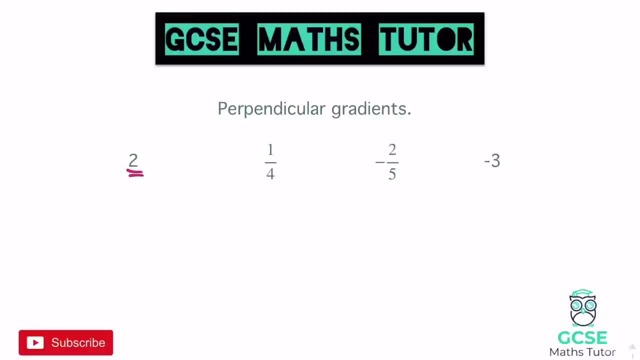 a look at over here is if we've got a gradient of two. So if we have a line with a gradient of two which, thinking about what that would look like, it would be sloping upwards, something like this: So let's imagine this line has a gradient of two. Now if we create a 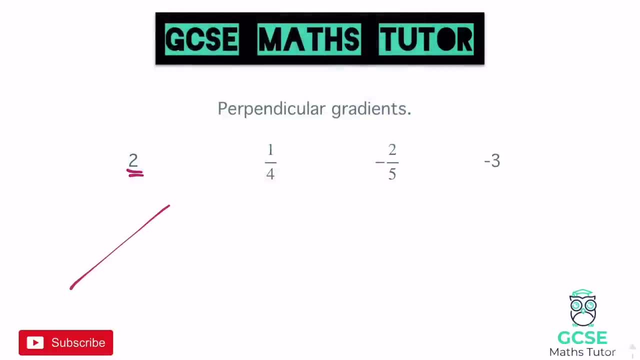 perpendicular line to this. it would be sloping, obviously at a 90 degree angle in the other direction, like this. Now it's quite easy to find the perpendicular gradient, but if we think about what a perpendicular gradient would kind of look like, this original line here would have a rise. 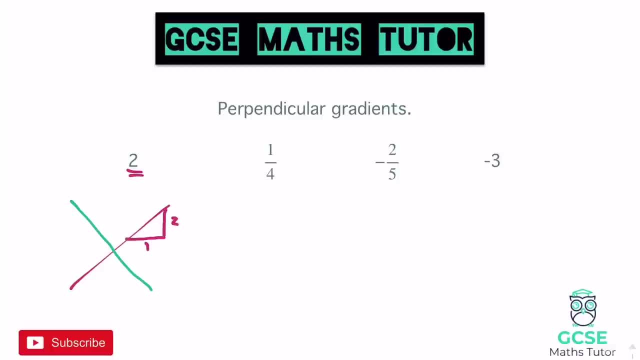 of two and a run of one, and that's what makes it have that perpendicular gradient, So that gradient of two there a rise of two and a run of one, or a change in y of two and a change in x of one. 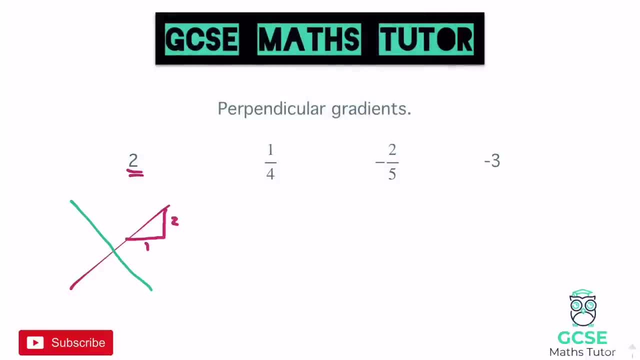 Now, if we were to rotate that 90 degrees to create this perpendicular line, which would look something like this: if you imagine now where those numbers would be, the two would be on the bottom there and the one would be on the side. Okay, so now our rise is one and our run is two. Okay, so over here. 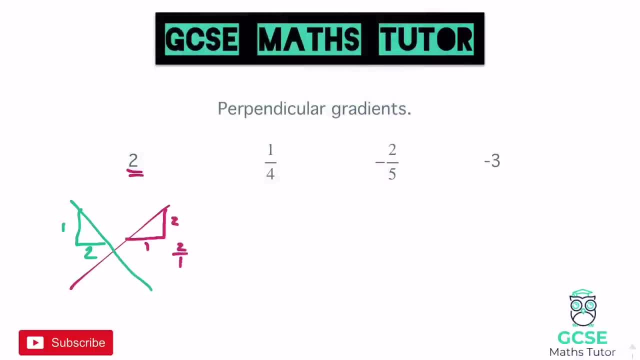 although we had. let's have a look- a rise over run would be two over one, which gives us a gradient of two. this one now gives us a rise of one and a run of two and is sloping downwards. so it would be. 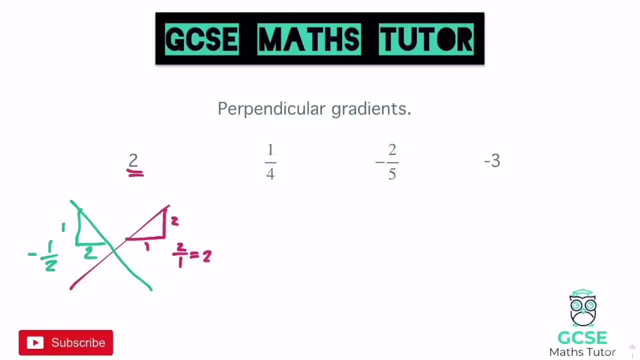 negative, so it would be negative a half. Okay, so just thinking visually about why we get the gradient that we do here, that's what it would actually look like there. So instead of having a rise of two and a run of one, it would have a rise of one and a run of two and would be sloping. 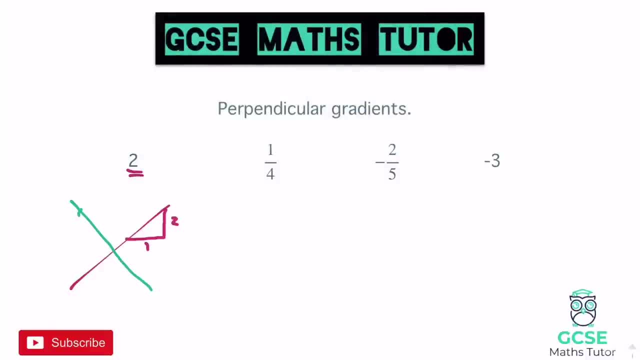 Now, if we were to rotate that 90 degrees to create this perpendicular line which would look something like this: if you imagine now where those numbers would be, the two would be on the bottom there and the one would be on the side. Okay, so now our rise is one and our run is two. Okay, so over. 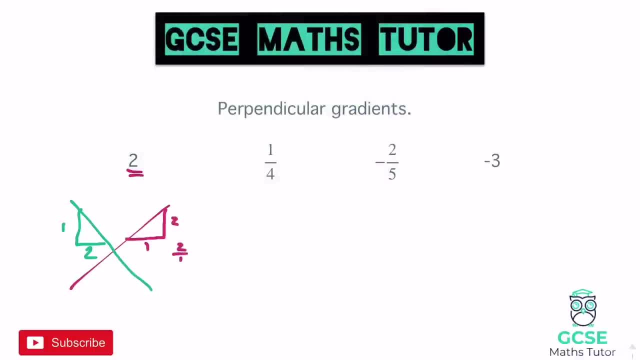 here, although we had- let's have a look- a rise over run would be two over one, which gives us a gradient of two. this one now gives us a rise of one and a run of two, and it's sloping downwards. so it'd be. 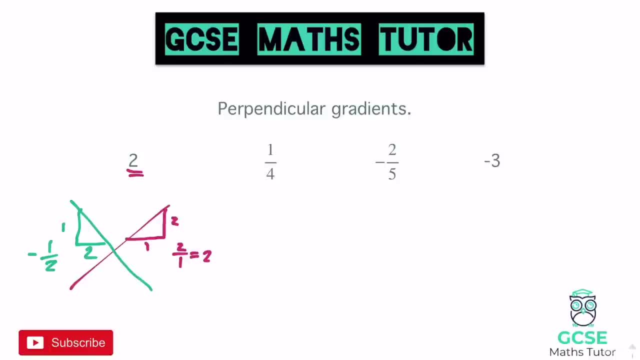 negative, so it'd be negative a half. Okay. so just thinking visually about why we get the gradient that we do here, that's what it would actually look like there. So instead of having a rise of two and a run of one, it'd have a rise of one and a run of two and would be sloping downwards or in. 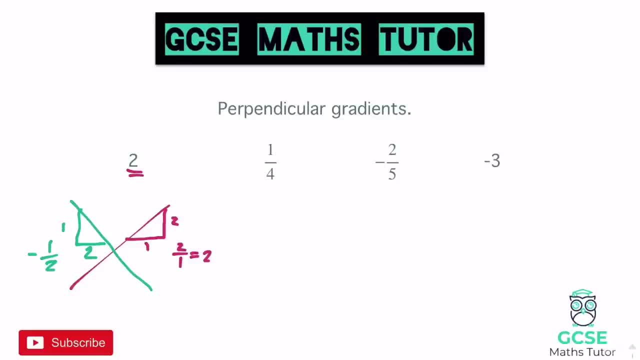 the opposite direction. Of course, if it was sloping downwards originally, it'd now be sloping upwards. Okay, so what actually happens here is something called the negative reciprocal, which is the name of this perpendicular gradient. so how do we get from two to negative a? 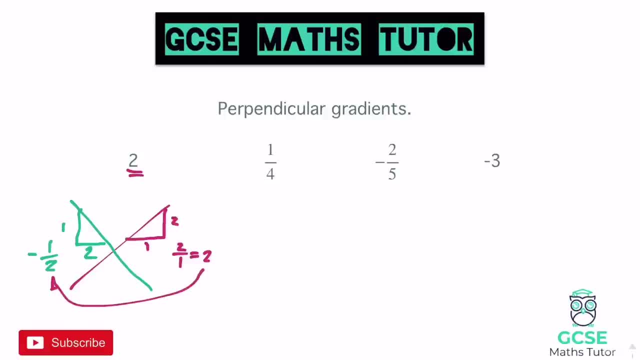 half just using the numbers, and that's what we're going to have a look at here. So I'm going to get rid of this and you're going to see why we get the negative a half here just using the numbers. 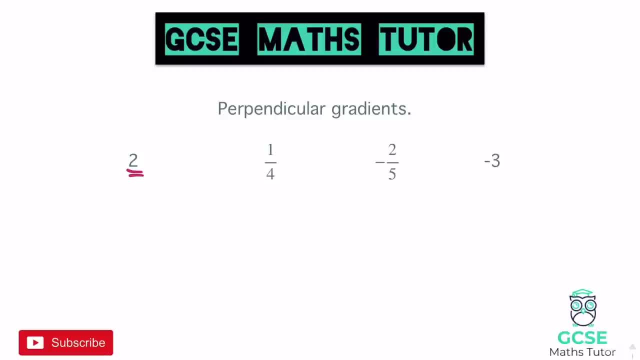 Let's get rid of that Right. so first things first, we're going to look at the two and we're going to imagine that it's a fraction. So if it was a fraction- which seems a bit strange- it would be two over one. Okay, so any number can be written as a fraction, just by putting it over one. Now to 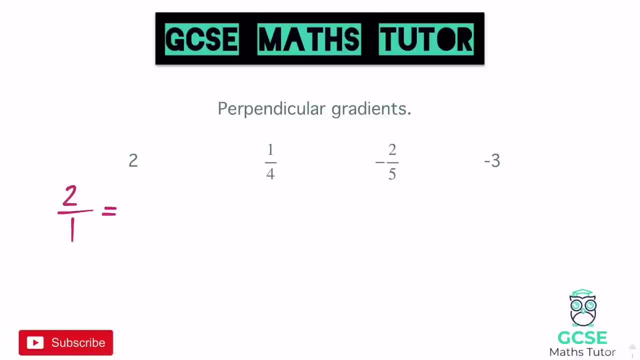 get the negative reciprocal. okay, negative just meaning that we swap the symbol. so currently it's positive, so it's definitely going to become negative Again. thinking about that visual idea that I drew there. if it was sloping upwards, it'll now be sloping downwards and the reciprocal just means to flip. 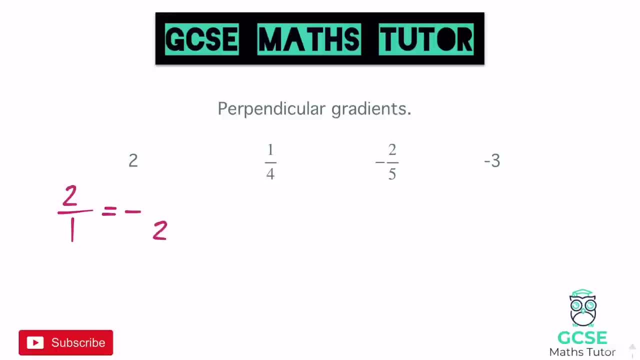 it over, essentially. So the two's going to go on the bottom, the one's going to go on the top and there's our gradient negative a half, and it's called doing the negative reciprocal. Okay, so what we're going to do in all of these circumstances here to get the perpendicular 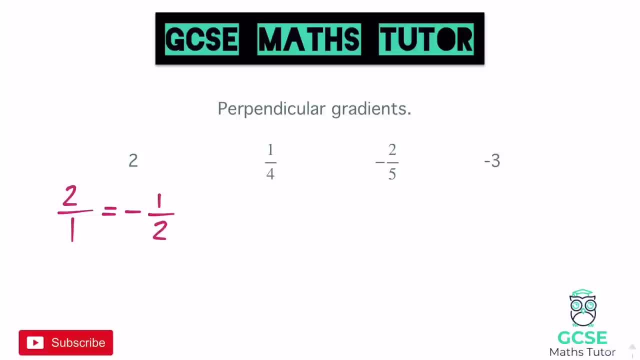 gradient is to flip it over, which is called the reciprocal, and to swap the symbol in front of it. so if it's positive, it'll become negative, and likewise, if it's negative it'll become positive. So for this next one, here one quarter. if we flip it over, we get. 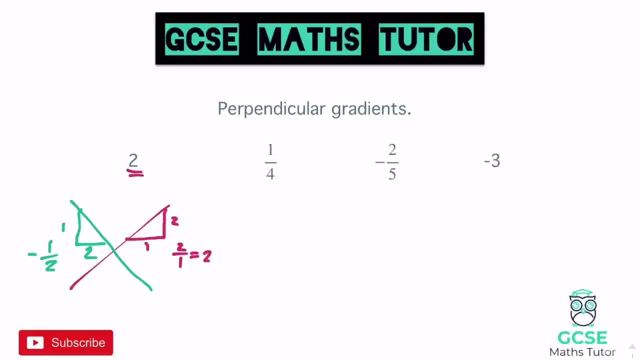 downwards or in the opposite direction. Of course, if it was sloping downwards originally, it would now be sloping upwards. Okay, so what actually happens here is something called the negative reciprocal, which is the name of this perpendicular gradient. So how do we get from two to negative a? 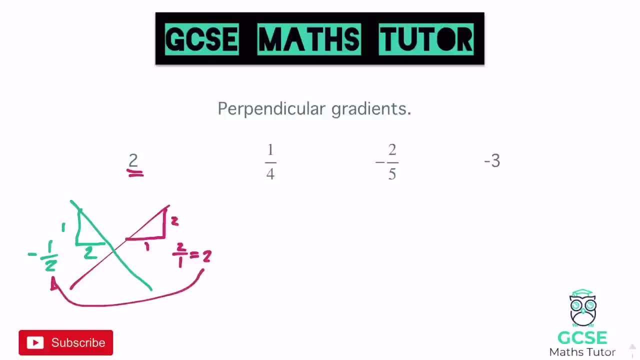 half Just using the numbers, and that's what we're going to have a look at here. So I'm going to get rid of this and you're going to see why we get the negative a half here just using the numbers. Let's get rid of that, Right. so first things first. we're going to look at the two and we're 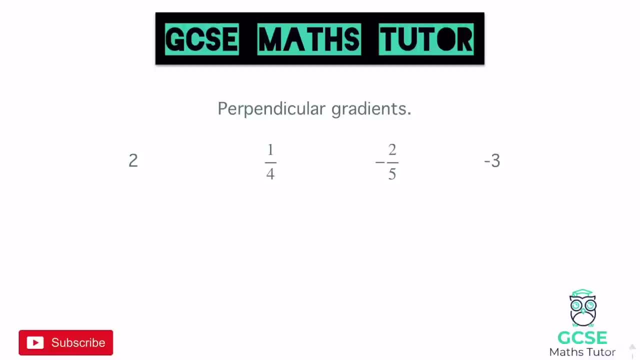 going to imagine that it's a fraction. So if it was a fraction- which seems a bit strange- it would be two over one. Okay, so any number can be written as a fraction, just by putting it over one. Now to reciprocal. okay, negative, just meaning that we swap the symbol. So currently it's positive. so 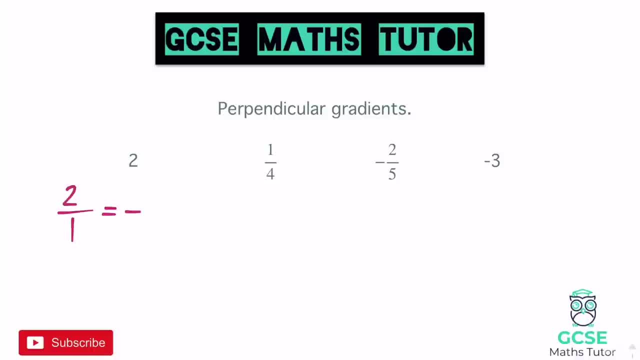 it's definitely going to become negative. Again, thinking about that visual idea that I drew there, if it was sloping upwards, it will now be sloping downwards And the reciprocal just means to flip it over. essentially, So the two is going to go on the bottom, the one's going to go on the top. 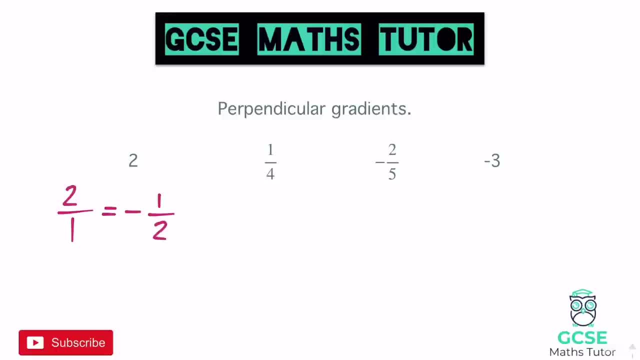 and there's our gradient, negative a half, and it's called doing the negative, reciprocal. Okay, so what we're going to do in all of these circumstances here to get the perpendicular gradient, is to flip it over and to swap the symbol in front of it. So if it's positive, it'll become negative, And 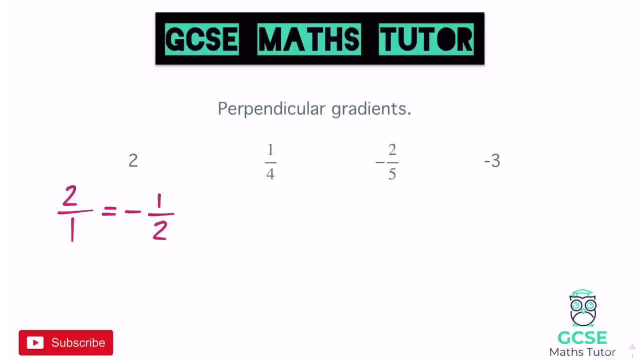 likewise, if it's negative it'll become positive. So for this next one here, one quarter. if we flip it over, we get four over one. It's currently positive, so it becomes negative, So it's negative four over one, And four over one is just four. So the answer or the perpendicular gradient in this: 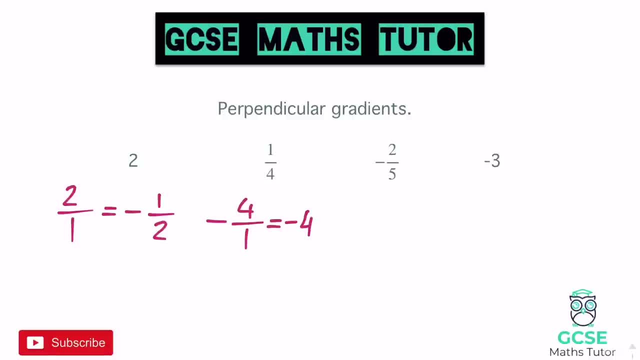 case would be negative four. And there's our perpendicular gradient. if we have a gradient of a quarter On to the next one, If we flip this over, so two fifths becomes five over two. just flipping those numbers over It's currently negative, So now it's positive. I don't have to. 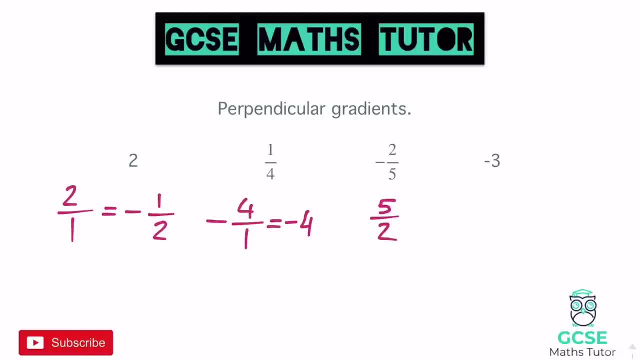 emphasise that it's positive there. I can just leave it as five over two. I could put a plus sign in front of it, but we don't have to. We'll assume it's positive if there's no negative symbol. So that would be five over two, which we could write as a decimal as well. We could write that: 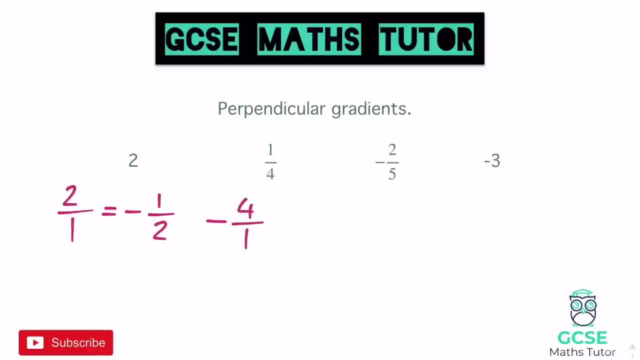 four over one. It's currently positive, so it becomes negative, so it's negative four over one, and four over one is just four. so the answer or the perpendicular gradient in this case would be negative four and there's our perpendicular gradient if we have a gradient of a quarter. 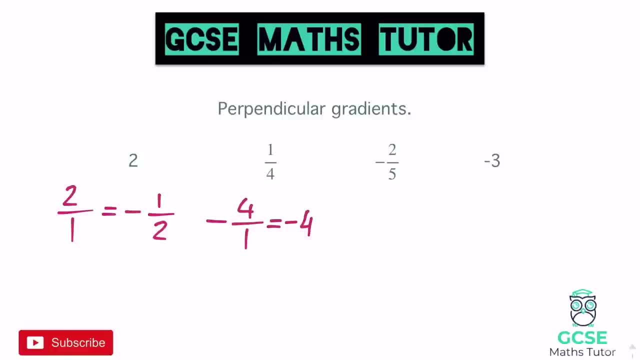 On to the next one. if we flip this over, so two fifths becomes two. just flipping those numbers over, it's currently negative, so now it's positive. I don't have to emphasise that it's positive there. I can just leave it as five over two. I could put a plus. 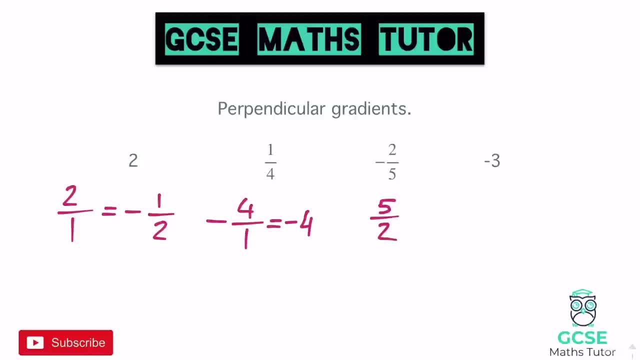 sign in front of it. but we don't have to. we'll assume it's positive if there's no negative symbol. So that'll be five over two, which we could write as a decimal as well. we could write that as 2.5.. 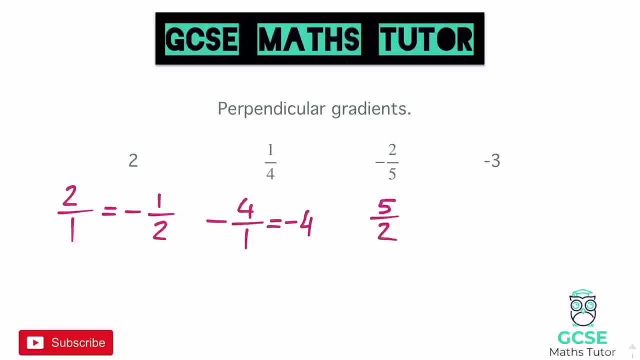 Again, remember you could actually just turn it into a mixed number. Two goes into five twice with a remainder of one, so it's two and a half or 2.5.. Absolutely fine for you to leave it in either way, just whichever you prefer. We'll have a look at when we might use different. 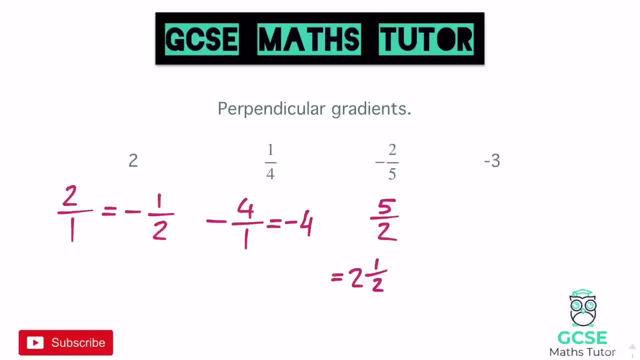 when we might use decimals or fractions later on. And the last one here: negative three. remember that currently is a fraction. I'm just going to put a one underneath up here, So it's negative. three over one. flip it over and it becomes a third. And again it's positive, so it just stays as a third. We don't. 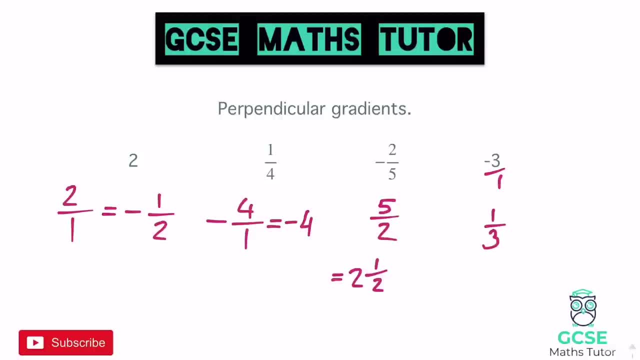 have to worry about converting that or writing it as a decimal. we can just leave it as one third. There we go. So that is the process we're going to use throughout the topic here, And there's just one extra little thing that I do tend to do when I'm writing down the gradient. So if we refer back, 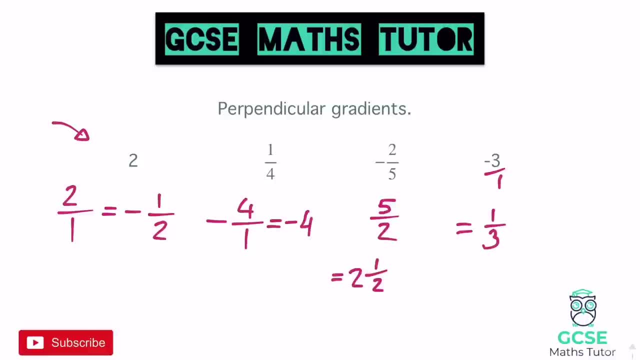 to this two over here when I'm writing down the gradient. I'm going to write down the gradient, I'm referring to the gradient. I label it as m equals two. Okay, just referring back to our equation of a line that we looked at in the last video: y equals mx plus c. the m there represents 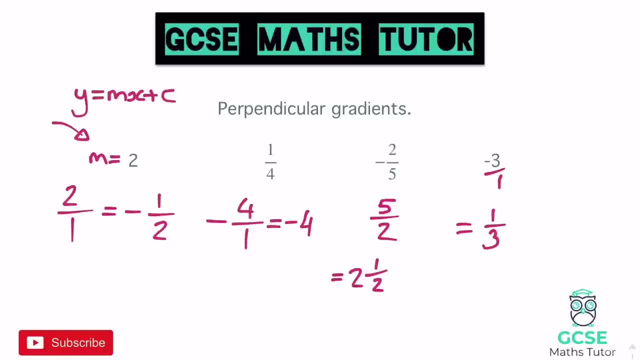 the gradient. So when I'm labeling the gradient, I say m equals two, And when I'm labeling the perpendicular gradient- which is what I've done here- negative a half, I do m again, but I put a little mini p with it, just say mp. And that is how I label the perpendicular gradient. Okay, 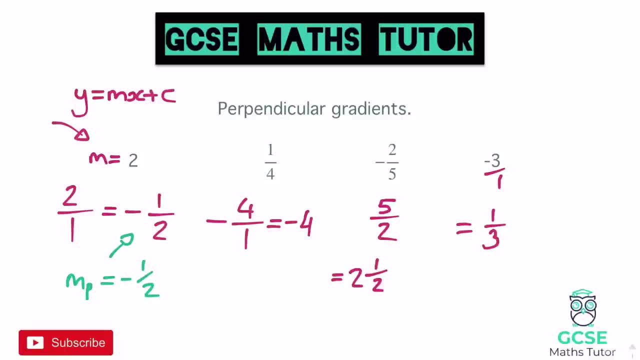 so I say mp equals negative a half, And it's a good little exam technique as well, just to show you are actually aware of what you are doing here. you're finding the perpendicular gradient, So I'm going to be using that throughout the video as well. Okay, so m equals is for the 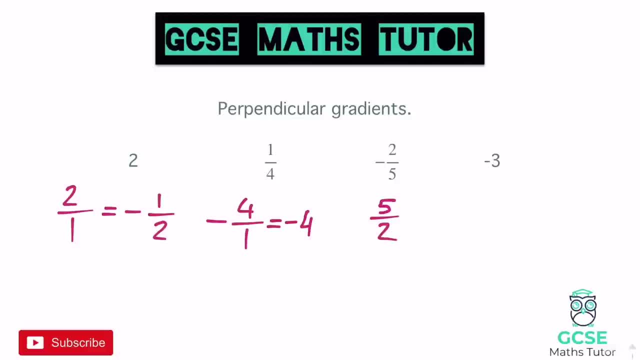 as 2.5.. Again, remember you could actually just turn it into a mixed number. Two goes into five twice with a remainder of one, So it's two and a half or 2.5.. Absolutely fine, for you to leave it. 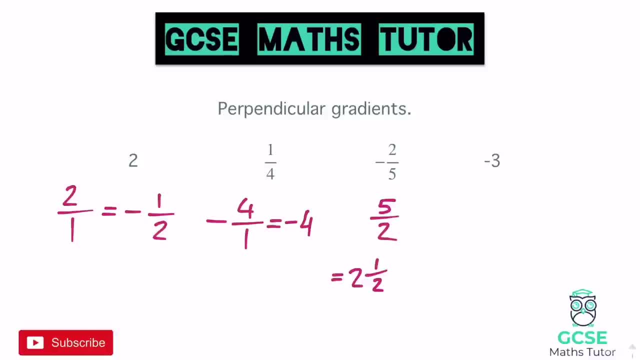 in either way, just whichever you prefer. We'll have a look at when we might use decimals or fractions later on. And the last one here, negative three. Remember that currently is a fraction. I'm just going to put a one underneath up here, So it's negative three over one. Flip it. 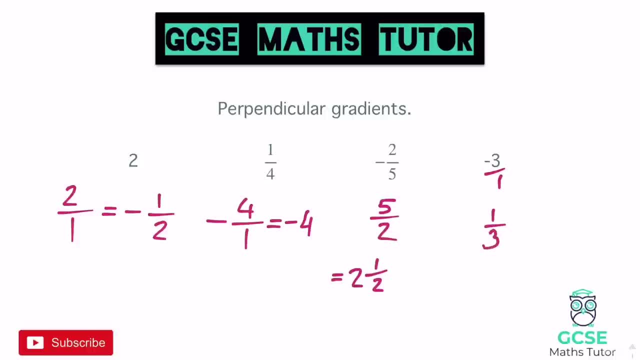 over and it becomes a third And again it's positive. so it just stays as a third. We don't have to worry about converting that or writing it as a decimal, We can just leave it as one third. There we go. So that is the process we're going to use throughout the topic here, And there's just 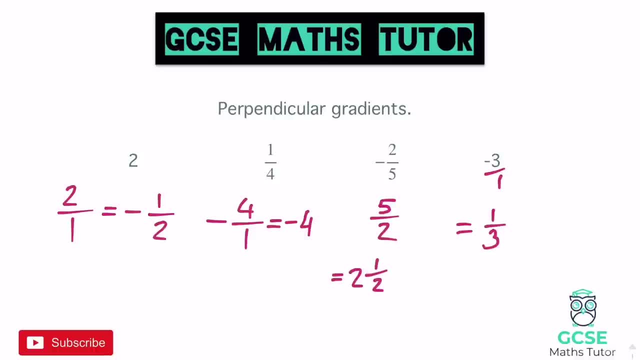 one extra little thing that I do tend to do when I'm writing down the gradient. So if we refer back to this two over here, when I'm referring to the gradient, I label it as m equals two. Just referring back to our equation of a line that we looked at in the last video: y equals mx plus c, The m there. 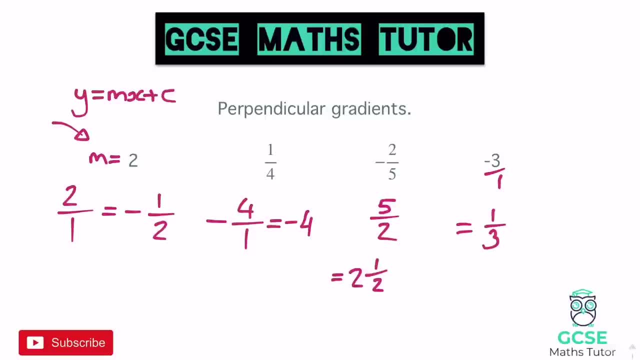 represents the gradient. So when I'm labeling the gradient I say m equals two, And when I'm labeling the perpendicular gradient- which is what I've done here- negative a half, I do m again, but I put a little mini p with it. just there say mp, And that is how I label the perpendicular. 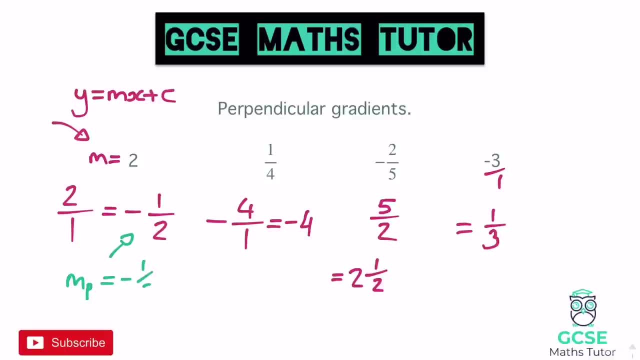 gradient. So I say mp equals negative a half, And it's a good idea to do that. So I'm going to do a little exam technique as well, just to show that you are actually aware of what you are doing here. You're finding the perpendicular gradient, So I'm going to be using that throughout the video. 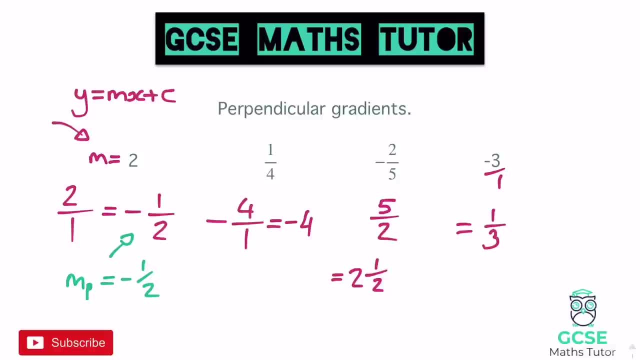 as well. So m equals is for the gradient and mp equals is going to give me my perpendicular gradient, my negative reciprocal there. Let's have a look at seeing how we can approach this in some questions. So it says: find the equation of a line perpendicular to y equals a half x minus. 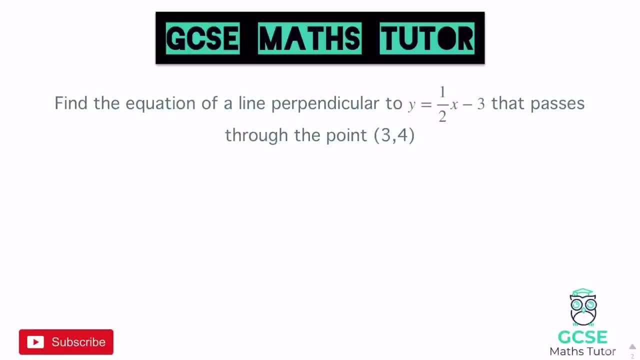 three, that passes through the point three. four: Now, first things first. I'm going to write down what the gradient is up here. So I'm going to write down what the gradient is up here. So I'm going to write down what the gradient is up here. So the gradient equals a half. there we go And I. 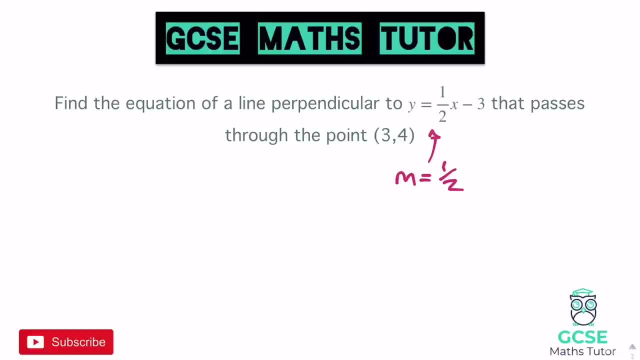 need to find a perpendicular line to this that passes through a particular point. Now, straight away, I can write down my y equals mx plus c, But I need to work out what my gradient actually is. Now, if it's a perpendicular line, I need to find the perpendicular gradient of a half. So 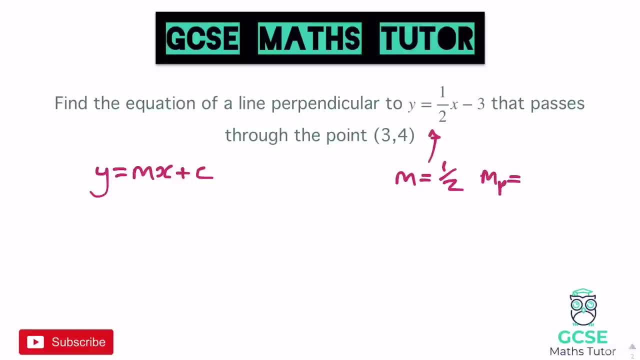 first things I'm going to do is I'm going to write that down. So mp equals. flip it over and change the sign. we get negative two over one, which is negative two, And again you can write down as negative two over one and then simplify it down to negative two if you want. But there we are. 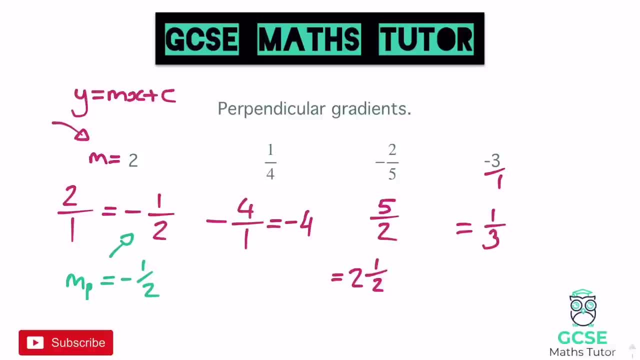 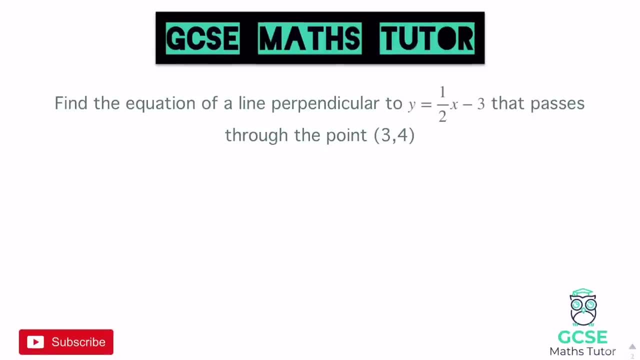 gradient and mp equals is going to give me my perpendicular gradient, my negative reciprocal. there Let's have a look at seeing how we can approach this in some questions. Okay, so it says: find the equation of a line perpendicular to y equals a half x minus three. that passes through. 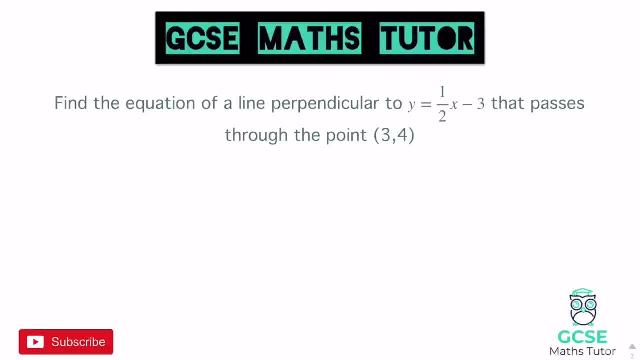 the point three. four, Now first things first. I'm going to write down what the gradient is up here. So the gradient equals a half. There we go, And I need to find a perpendicular line to this that passes through a particular 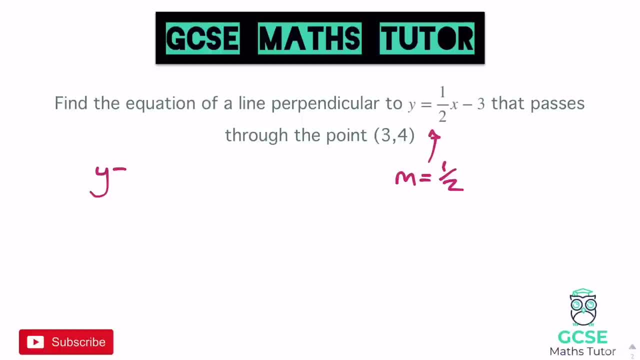 point Now straightaway. I can write down: my y equals mx plus c, But I need to work out what my gradient actually is. Now, if it's a perpendicular line, I need to find the perpendicular gradient of a half. So first things I'm going to do is I'm going to write that down So mp equals- flip it. 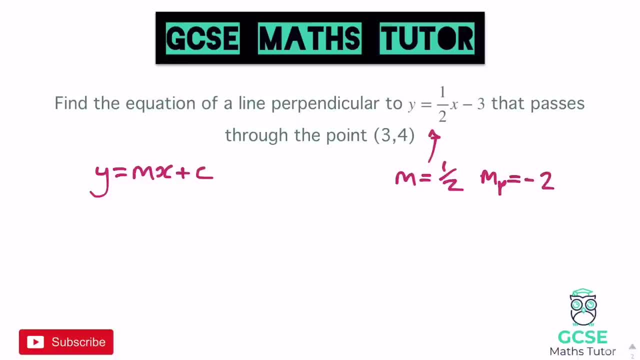 over and change the sign. we get negative two over one, which is negative two, And again you can write that down as negative two over one And then simplify it down to negative two if you want. But there we are. that's the gradient we're going to be. 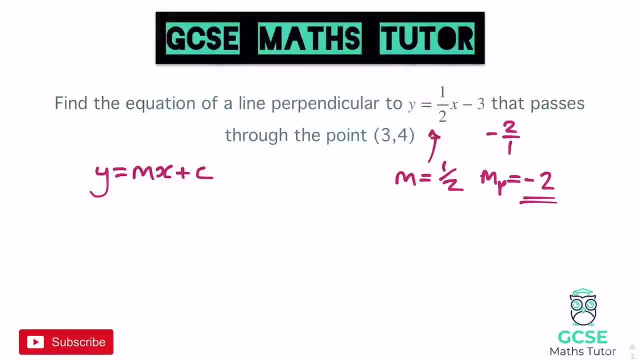 using negative two. So, just like before we've done this, put your minus two into your line equation. So y equals minus two, x plus c, And we're going to start to figure out the equation of this line. Now. we don't really need to know the fact that it has a negative three at the end. 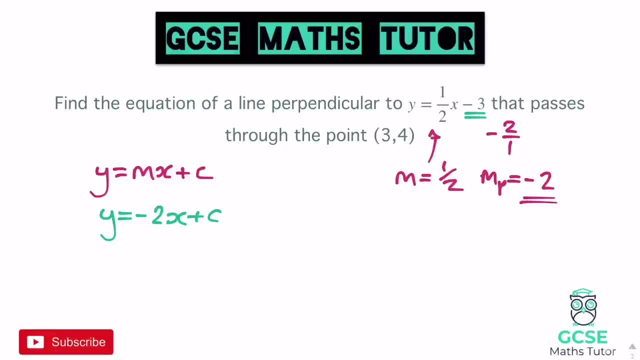 it doesn't really matter what the y-intercept of that line is. All we really need to know is what the point is, that our line is going to go through, And that's three, four. So that negative three up there doesn't really do anything for us. Okay, so we can actually just ignore the. 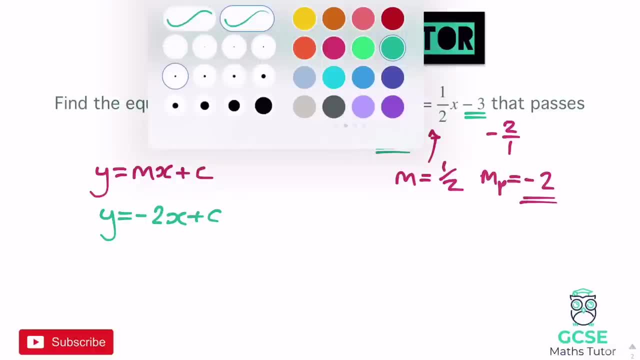 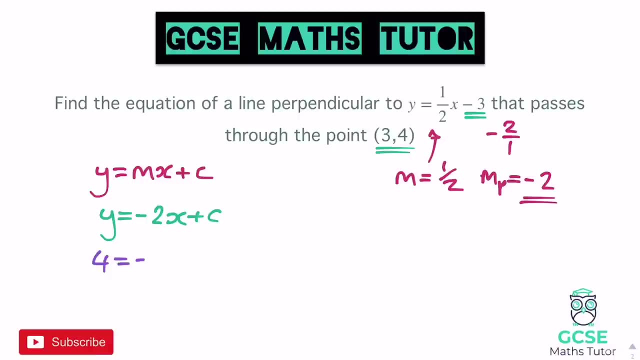 y-intercept of that line, Right. so if we stick this point in, then we've got three, four to put in. So y is four. so put four in place of y, And then three is x. So we'll sub that in. so it's negative. 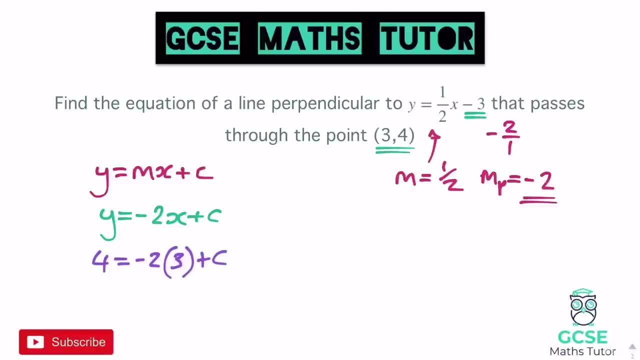 two times three plus c, And then we just need to simplify this down, get rid of that bracket there and solve this for c. So four equals negative. two times three is negative six plus c And adding six to both sides there to get c on its own. 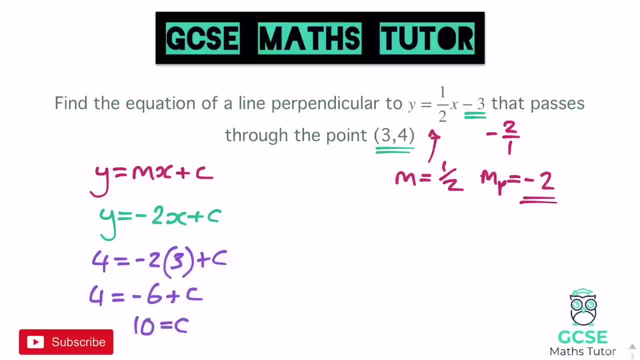 Isolate c, add six to both sides, we get 10 equals c or c equals 10.. And now we've got c. we can write our line equation just replacing this c with the number that we want, the number that we found there. 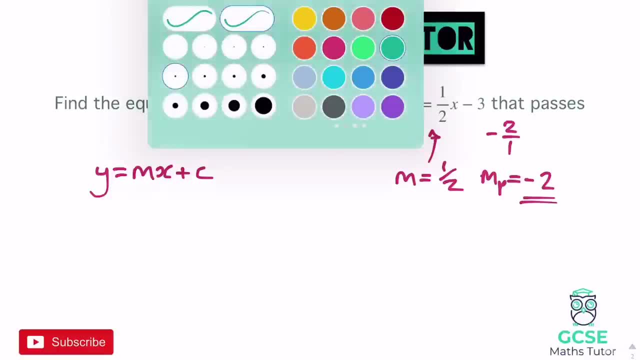 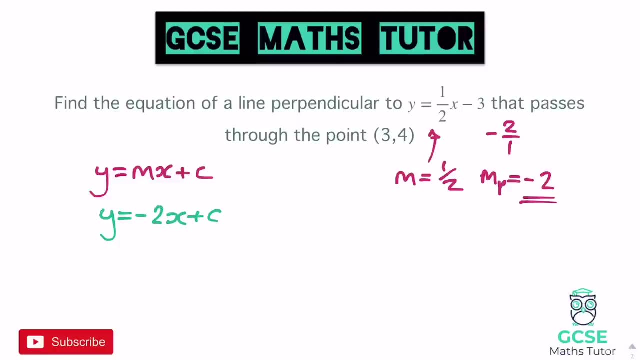 that's the gradient. we're going to be using negative two. So, just like before, when we've done this, put your minus two into your line equation. So y equals minus two, x plus c, And we're going to start to figure out the equation of this line Now. we don't really need to know. 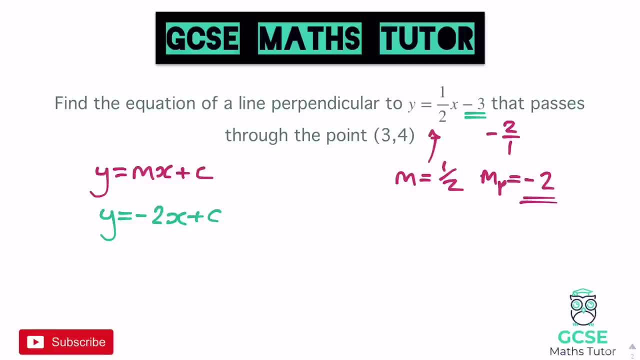 the fact that it has a negative three at the end. It doesn't really matter what the y-intercept of that line is. All we really need to know is what the point is. that our line is going to go through and that's three- four. So that negative three up there doesn't really do anything. 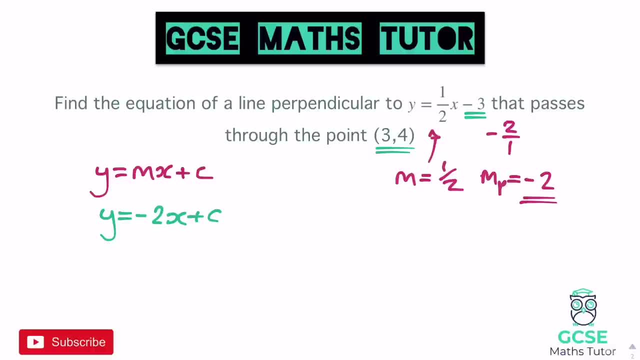 for us. okay, So we can actually just ignore the y-intercept of that line, Right? so if we stick this point in, then we've got three, four to put in. So y is four. So put four in place of y, And then three is x. So we'll sub that in. So it's negative two times three. 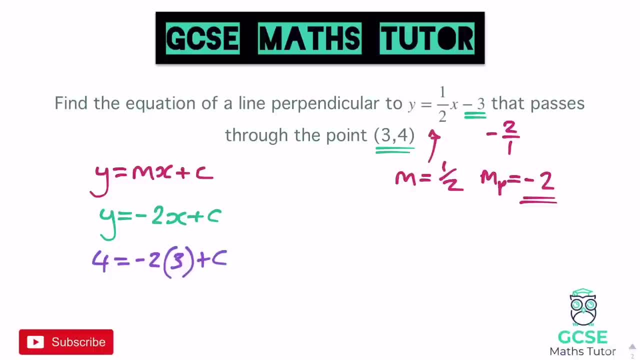 plus c. And then we just need to simplify this down, get rid of that bracket there and solve this for c. So four equals negative two times three is negative. six plus c And adding six to both sides to get c on its own to isolate c. add six to both sides, we get 10 equals c or c equals 10.. 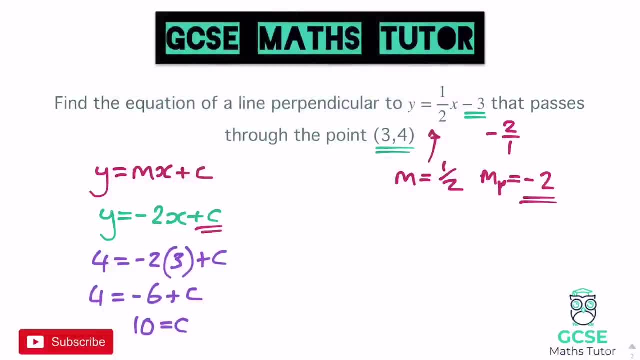 Now we've got c, we can write our line equation just replacing this c with the number that we want, the number that we found there, 10.. So we get y equals negative two x plus 10.. And obviously you could write that in a different way as well. You could write 10 minus two x and 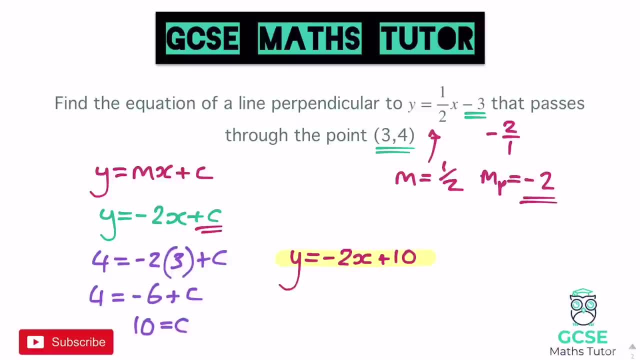 swap them around. but that's absolutely fine, just to leave your answer like that. So y equals negative two x plus 10.. Let's have a look at another one. Okay, so find the equation of a line perpendicular to the line. So we've got: y equals negative two x plus 10.. So we've got y equals. 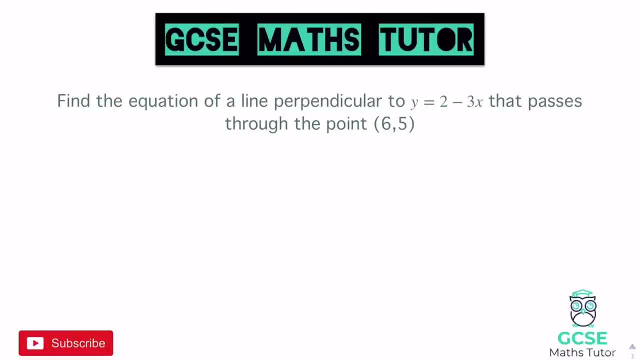 perpendicular to y equals two minus three x. that passes through the point six, five. So first things first, let's get the gradient out of this. Now it's written in a slightly different way because it's got a negative gradient, but our gradient there is negative three. the number in 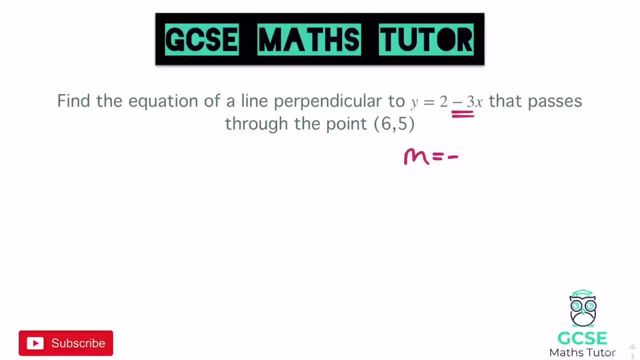 front of the x. So let's write that down. m equals negative three. Straight away we're finding a perpendicular line. So let's find the perpendicular gradient. So mp. change it to positive, flip it over and it becomes a third Right. so we just need to put a third into our line equation. 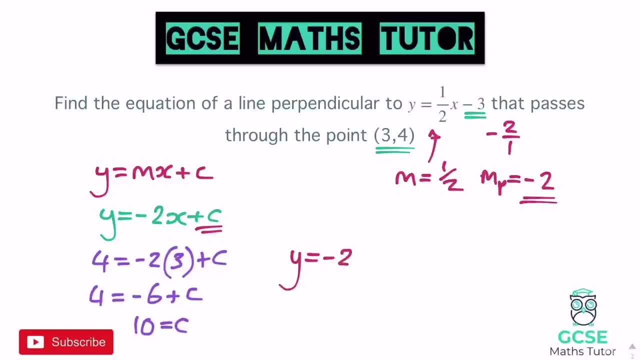 10.. So we get: y equals negative two x plus 10.. And obviously you could write that in a different way as well. You could write 10 minus two x and swap them around. but that's absolutely fine, just to leave your answer like that. So y equals negative two x plus 10.. So have a look at another. 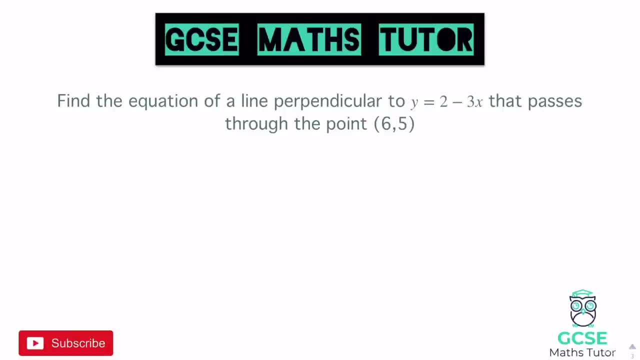 one. Okay. so find: the equation of a line perpendicular to y equals two minus three x that passes through the 0.65.. So first things first, let's get the gradient out of this. Now it's written in a slightly different way because it's got a negative gradient, but our gradient 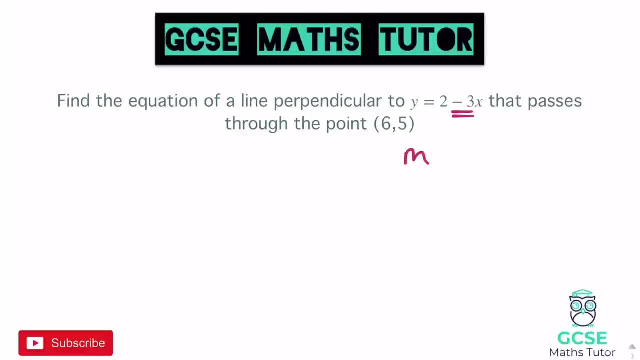 there is negative three, the number in front of the x. So let's write that down: m equals negative three. Straight away we're finding a perpendicular line, so let's find the perpendicular gradient. So mp, change it to positive, flip it over, it becomes a third Right. so we just need to put. 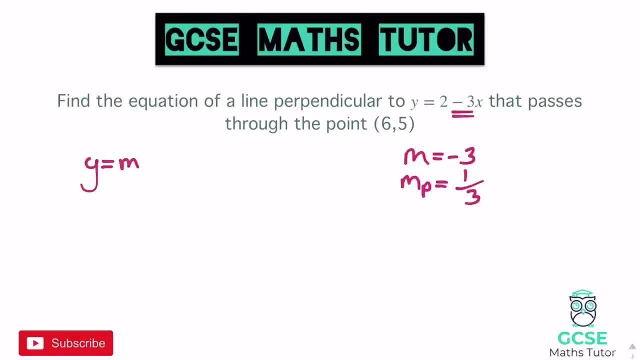 a third into our line equation. So writing down: y equals mx plus c And then let's put this gradient in So we get y equals a third x plus c, Right from there. same process again. So we're going to sub this coordinate in 6, 5, as that coordinate is on. 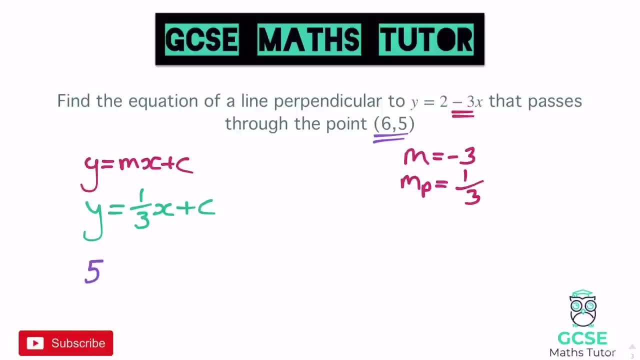 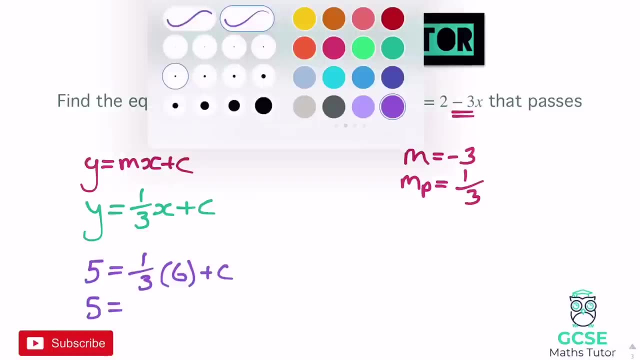 our line. So 5 equals y. So 5 equals one third times the x coordinate, which is 6 plus c. Right, let's expand that little bracket out. So we get 5 equals now one third times 6.. So you can treat this in two different ways. You can do a bit of working out. 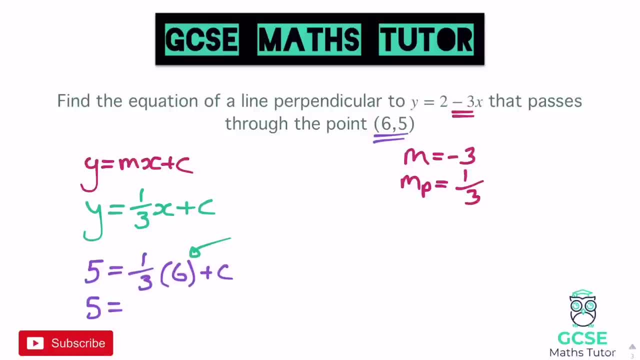 for this, if you want. If you times a third by 6, remember, 6 is 6 over 1, so you can just treat it like normal fractions- You get 6 over 3, and 6 over 3 equals 2.. And when you times a fraction, 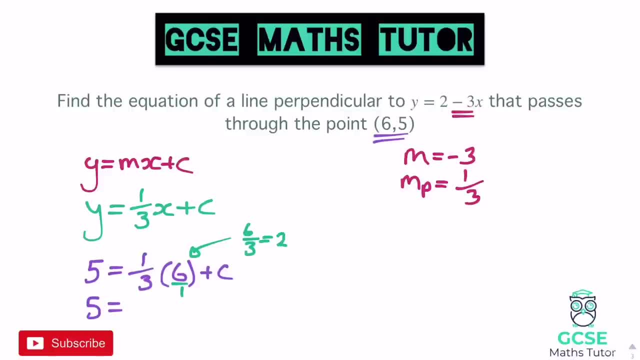 by a whole number, it just multiplies the numerator. So 6 times a third is 6 thirds, and when 6 thirds is 2.. OK, but you can also just think: when it's a fraction times 6,, if it's a nice one, a third of 6, or a third times 6, is just one third of 6.. 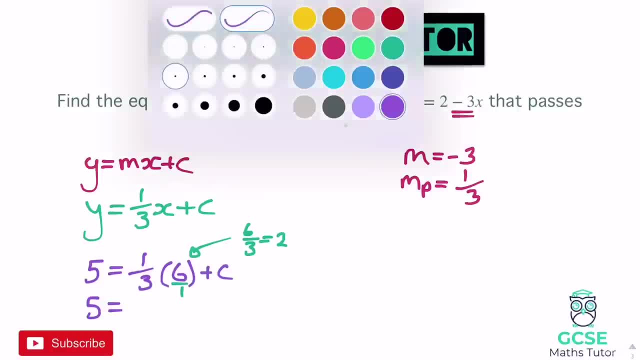 So 6 divided by 6 equals 6.. So 6 times a third is 6, and when it's a fraction times 6, by 3 equals 2.. So you can do it in two different ways there. It just depends how confident you are. 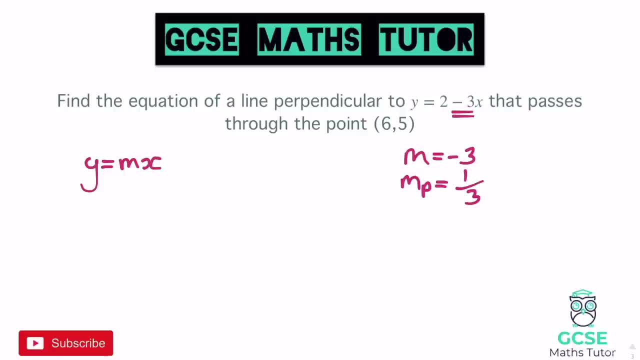 so writing down: y equals mx plus c, And then let's put this gradient in So we get y equals a third x plus c, Right from there. same process again. So we're going to sub this coordinate in six five. 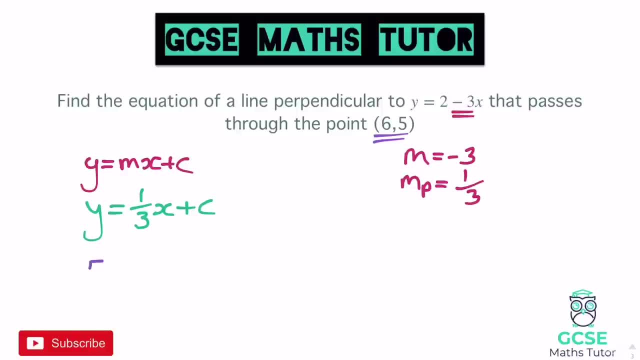 as that coordinate is on our line. So five equals y. So five equals one third times the x coordinate, which is six plus c. Right, let's expand that little bracket, So we get five equals now one third times six. So you can treat this in two different ways You. 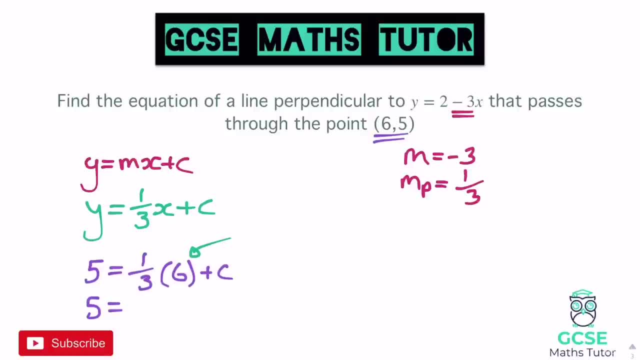 could do a bit of working out for this, if you want. If you times a third by six- remember, six is six over one, so you can just treat it like normal fractions- You get six over three, and six over three equals two, And when you times a fraction by a whole number, it just multiplies. 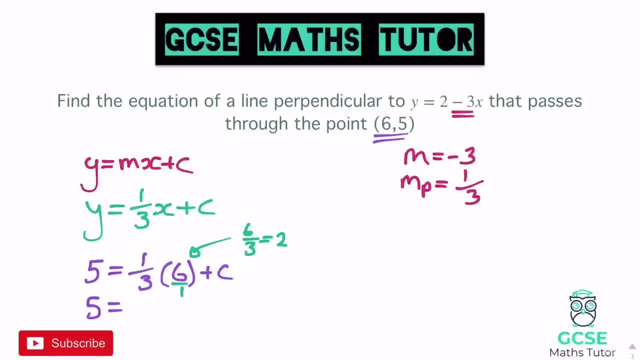 the numerator. So six times a third is six thirds, and when six thirds is two, Okay. but you can also just think: when it's a fraction times six, if it's a nice one, a third of six or a third times six. 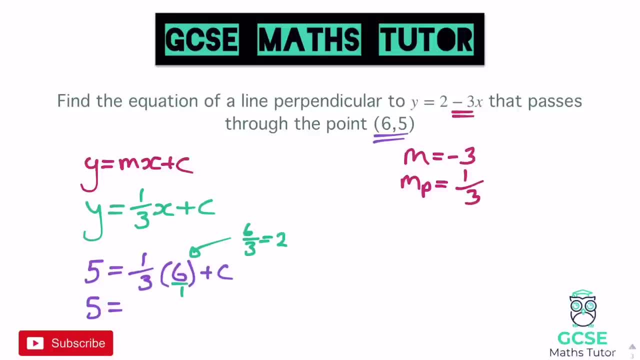 is just one third, So we get five equals now one third times six. So we get five equals now one third of six. So six divided by three equals two. So you can do it in two different ways there. It just depends how confident you are with your fractions here. But you can always just treat it in this. 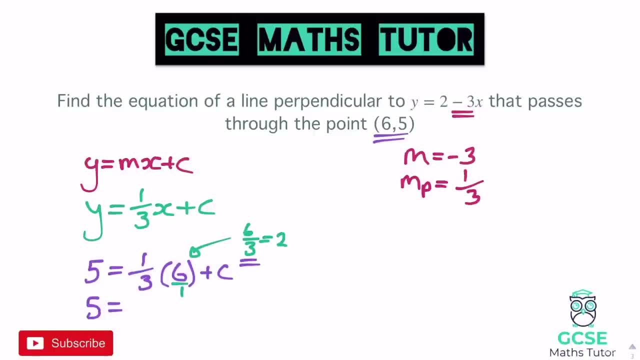 sense up here. So six times a third is six thirds, and simplify it down, And in this case it does become a whole number. So five equals two plus c. And then again, if we solve that for c, subtract two from both sides, we get three equals c, or c equals three as our value of c there. 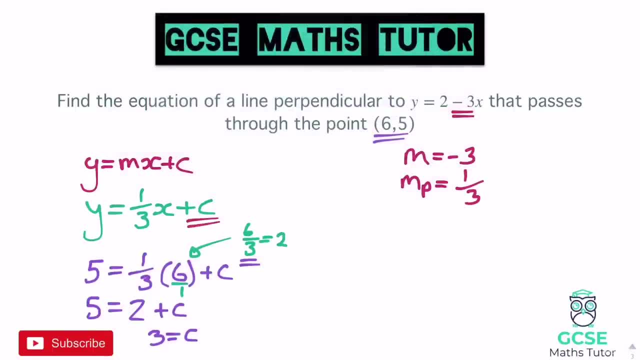 There we go. So we've got our y-intercept. now We can put it back into this line equation And we get: y equals one third x plus the three there that we've just worked out. And there's the equation of our line: one third x plus three. Okay, right, So here's some for you. 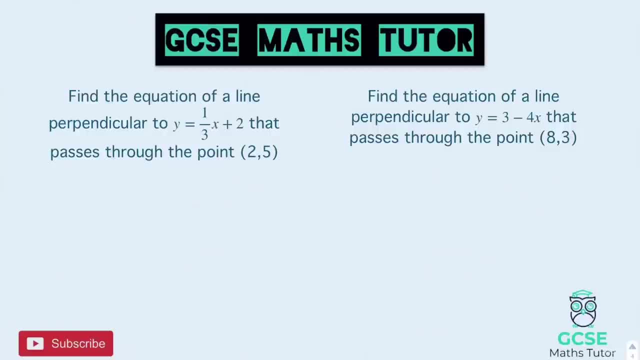 to have a go at. Okay, so there's two questions there. Have a go. Write down the gradient of the line, Write down the perpendicular gradient, Stick it into y equals mx plus c and then sub those coordinates in that are on the line there to find your line equation. So pause the video. 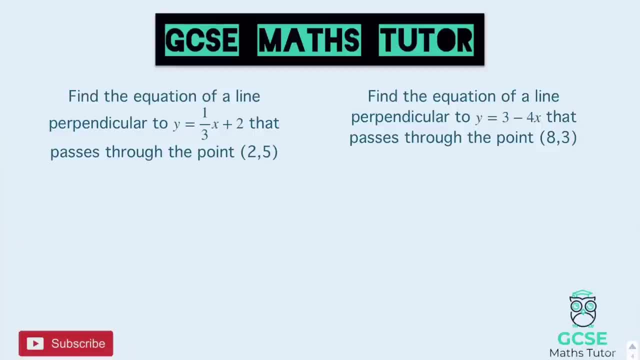 there and we'll go over that in a second. Okay, so we're going to go over that in a second. So the first one: there the gradient is currently a third, So our perpendicular gradient is going to be negative three. Putting that into our line, equation y equals minus three, x plus c, And. 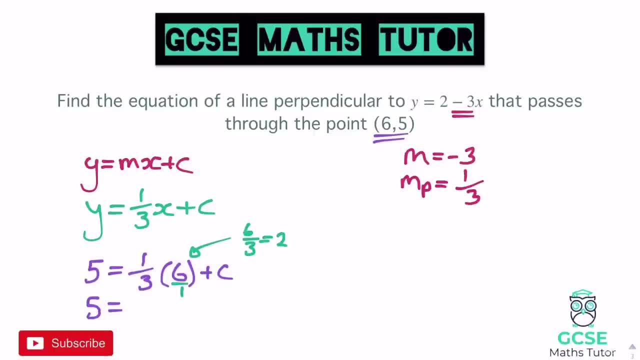 with your fractions here, But you can always just treat it in this sense up here. So 6 times a third is 6 thirds, and simplify it down, And in this case it does become a whole number. So 5 equals 2 plus c. And then again, if we solve that for c subtract 2 from both sides. 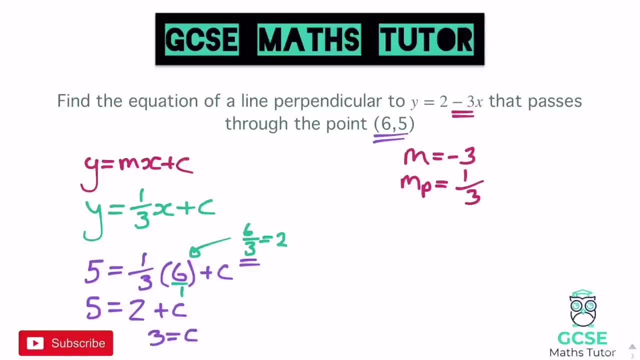 we get 3 equals c or c equals 3, as our value of c. there, There we go. So we've got our y intercept. now We can put it back into this line equation And we get y equals one third x plus the 3. there that we've just worked out, And there's the equation of our line. 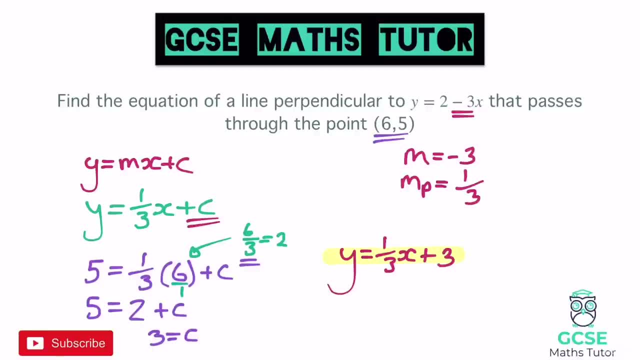 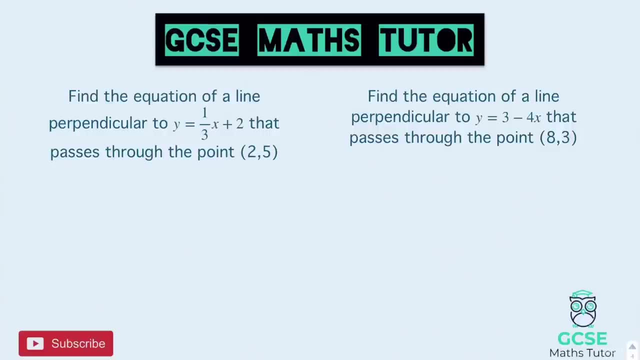 one third x plus 3.. OK, Right, so here's something for you to have a go at. OK, so there's two questions there. Have a go. Write down the gradient of the line, Write down the perpendicular gradient, Stick it into y equals mx plus c, And then sub those coordinates in. 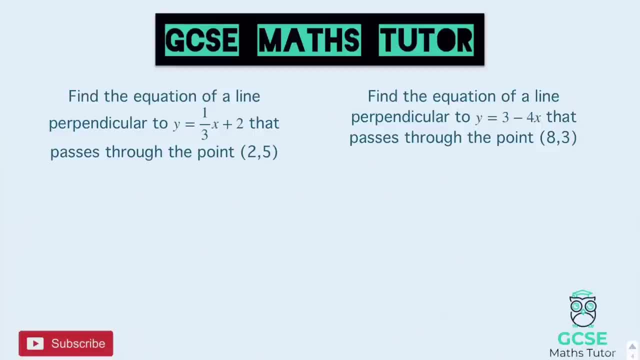 that are on the line there to find your line equation. Pause the video there and we'll go over that in a second. OK, so working these out. So the first one. there, the gradient is currently a third, So our perpendicular gradient is going to be negative. 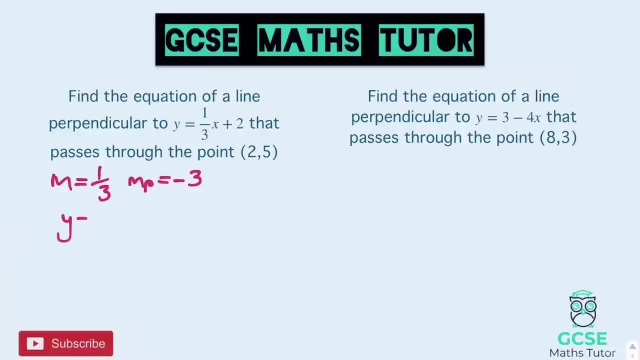 3. Putting that into our line equation: y equals minus 3x plus c, And then let's sub that coordinate into 5. So we get 5 equals negative 3 times 2 is negative 6 plus c. Add 6 to both sides. 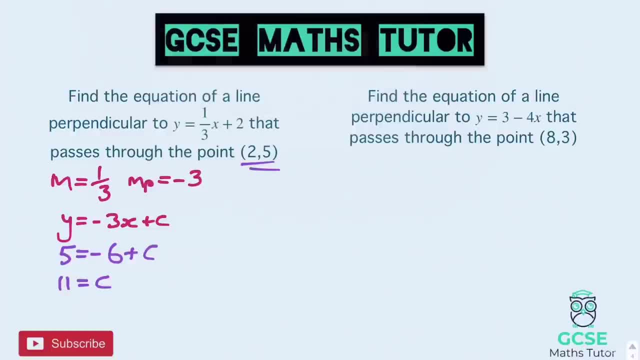 11 equals c. And then sticking that into our line equation to finish it off, y equals minus a third, sorry, minus 3x plus 11.. And there's the equation of our line for the first one. On to the second one, Our gradient for this one is negative 4, that negative 4 there in front. 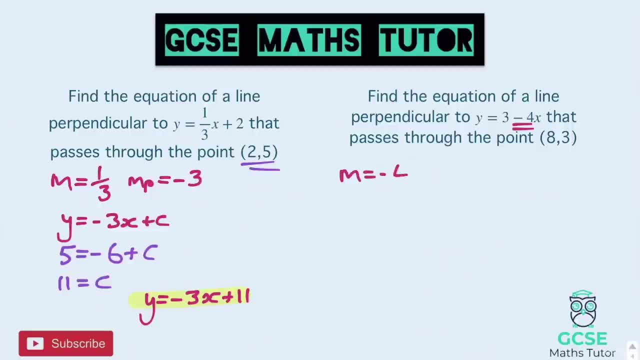 of the x, So m equals negative 4.. So our perpendicular gradient is going to be positive a quarter. There we go. So positive a quarter is our gradient. Sticking that into our line equation, y equals a quarter x plus c, And then subbing in our coordinate there, which is 8, 3 this time, So 3 equals. 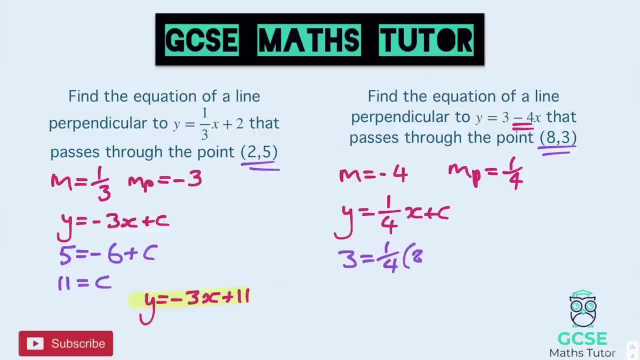 and I'm going to write the working out for this one: a quarter times 8 plus c, And we can do a quarter of 8 there or 8 quarters. We get 2.. A quarter of 8 equals 2.. 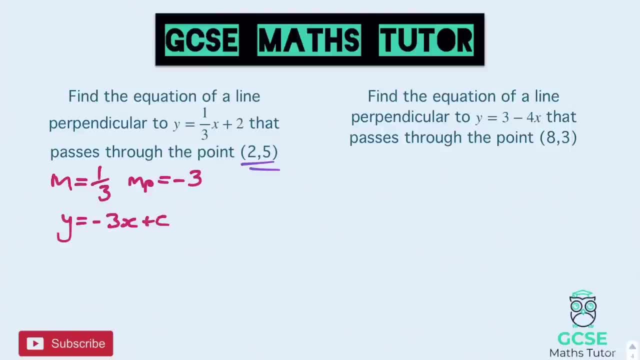 then let's sub that coordinate into five, So we get five equals negative. three times two is negative. six plus c. Add six to both sides, Eleven equals c And then stick that in there into our line equation. To finish it off: y equals minus a third, sorry, minus three, x plus 11.. 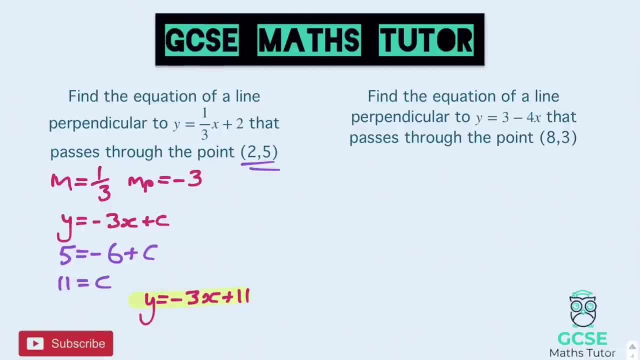 And there's the equation of our line for the first one On to the second one. Our gradient for this one is negative four, Negative four there in front of the x. So m equals negative four. So our perpendicular gradient is going to be positive a quarter. There we go. So positive a quarter is. 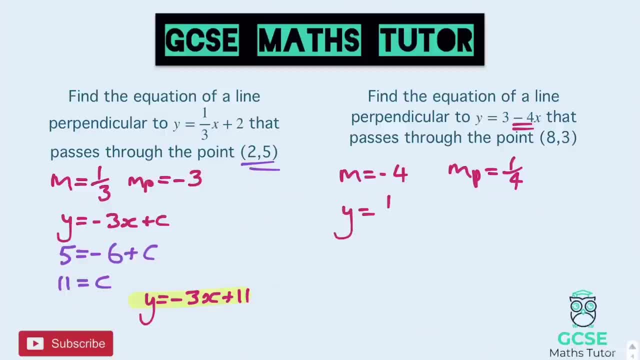 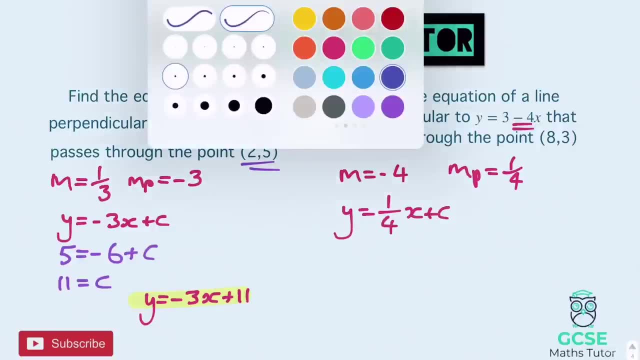 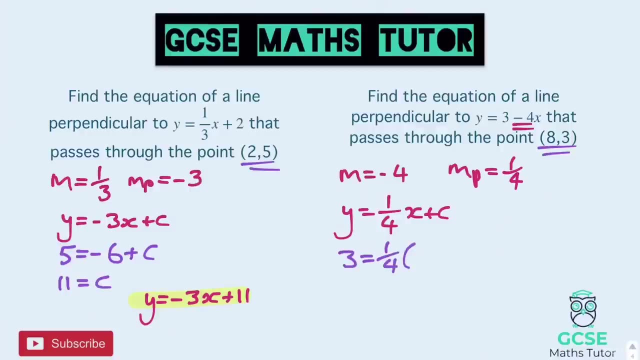 our gradient, Stick that into our line equation: Y equals a quarter x plus c, And then subbing in our coordinate there, which is eight, three this time. So three equals- and I'm going to write the working out for this: one a quarter times eight. 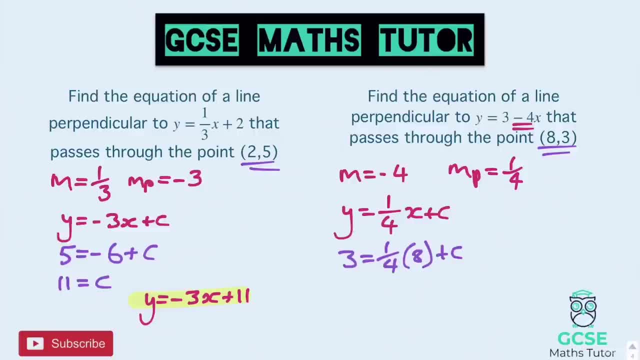 plus c, And we're going to do a quarter of eight there or eight quarters. We get two. Quarter of eight equals two. So three equals two plus c. Take away two from both sides. One equals c And then we can plug that in in place of c. there for our equation to finish it off. 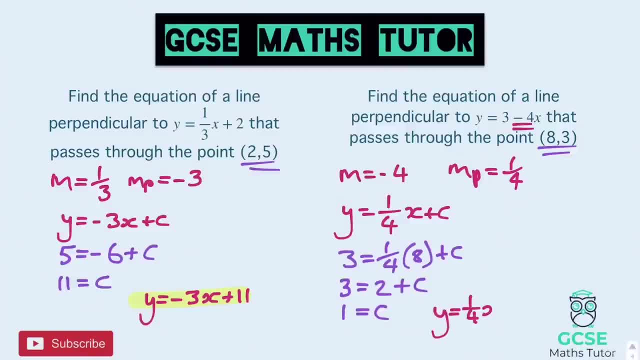 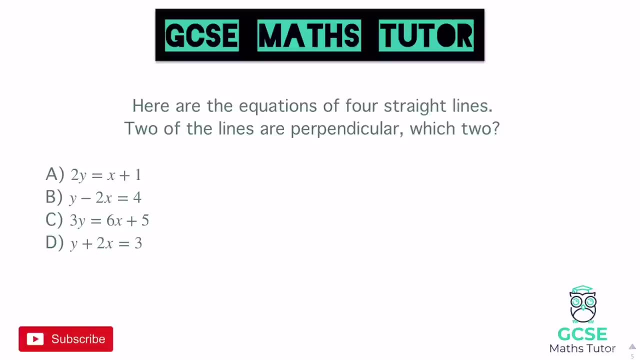 So y equals a quarter x plus one. There we go, And there's the equation of our line for that one. Right, let's have a look at something else. Okay, so what we're going to have a look at is some equations of lines where it isn't in the form. y equals mx plus c. So whenever we're looking at 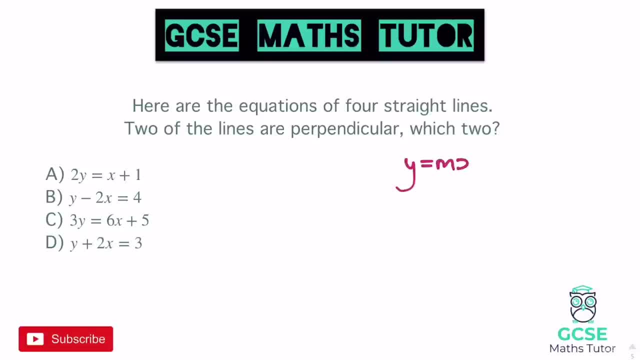 lines. we need it to be in this form here. Now it can be written in other forms, We can use them to compare them And in order to find out the gradient, it needs to be in this form here. So, looking at this question, it says: here are the equations of four straight lines. 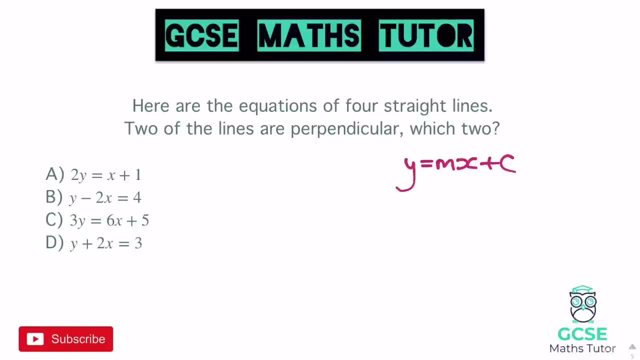 Two of the lines are perpendicular. which two? Now, if we look at this first one, it's not in the form. y equals mx plus c. Okay, it has a two in front of the y. So, in order to get it into the 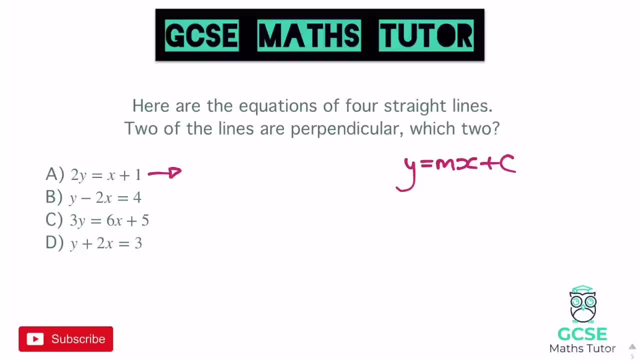 form: y equals mx plus c. we're going to have to divide everything by two. Okay, so I'm just going to write divide by two. I'm going to divide both sides by two. So two y divided by two gives us one y. 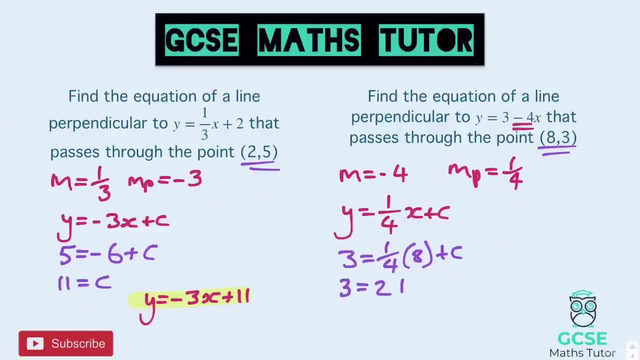 So 3 equals 2 plus c. Take away 2 from both sides, We get 1 equals c, And then we can plug that in in place of c there for our equation to finish it off. So y equals a quarter x plus 1.. 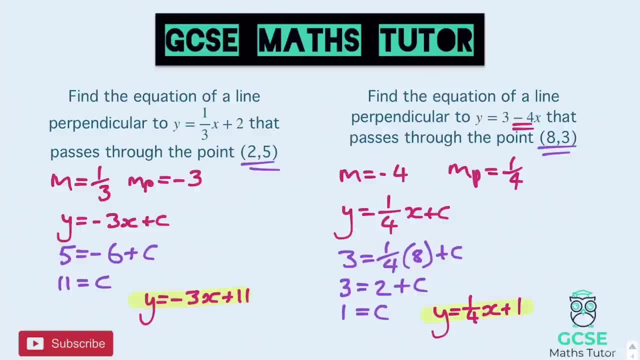 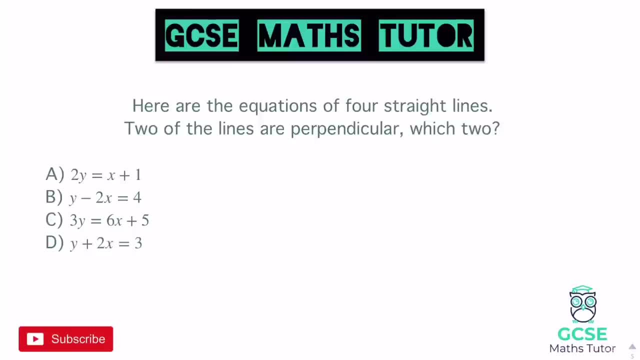 There we go, And there's the equation of our line for that one. Right, let's have a look at something else. Okay, so what we're going to have a look at is some equations of lines where it isn't in the form: y equals mx plus c. So whenever we're looking at lines, we need it to be in this. 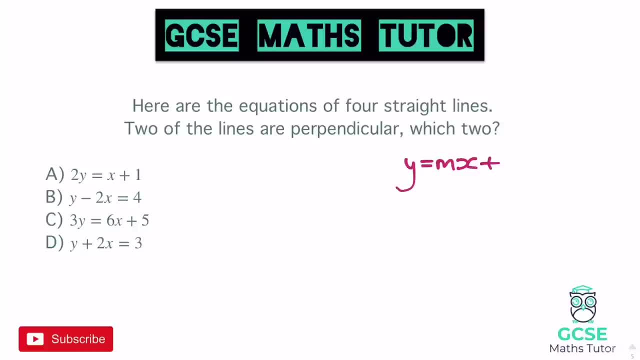 form here. Now it can be written in other forms, We can use them perfectly fine, But in order to compare them and in order to find out the gradient, we need to use them in some other forms. So in this form over here we have some stuff that we're going to have to crush together. So what we're going? 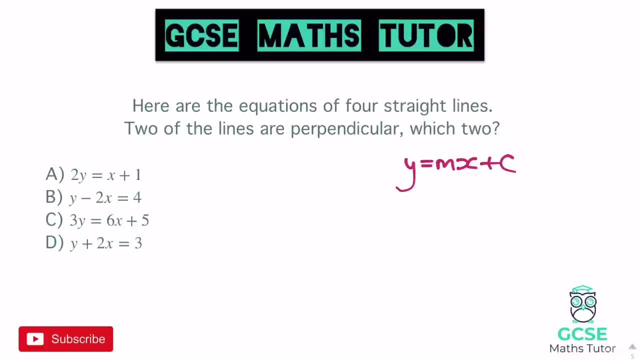 to do is add to that and we're going to add some blocks. So we have our lines and we're going to them and in order to find out the gradient, it needs to be in this form here. So, looking at this question, it says here are the equations of four straight lines. two of the lines are perpendicular. 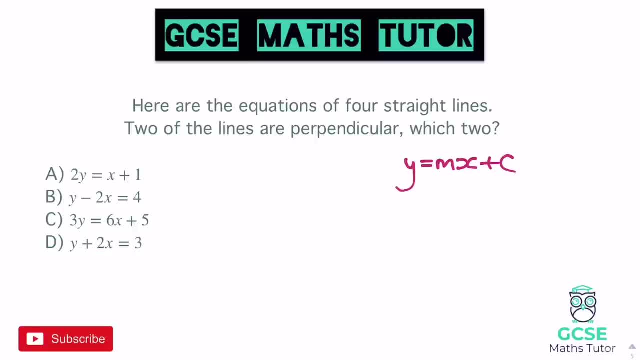 which two? Now, if we look at this first one, it's not in the form y equals mx plus c. Okay, it has a two in front of the y. so, in order to get it into the form y equals mx plus c, we're going to have 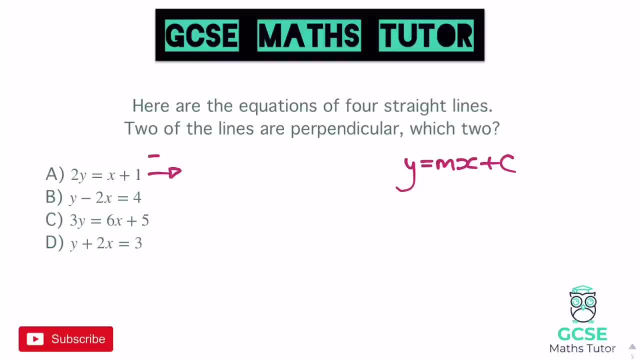 to divide everything by two. Okay, so I'm just going to write divide by two. I'm going to divide both sides by two. so 2y divided by two gives us 1y. We've got 1x there. 1 divided by two is a half. 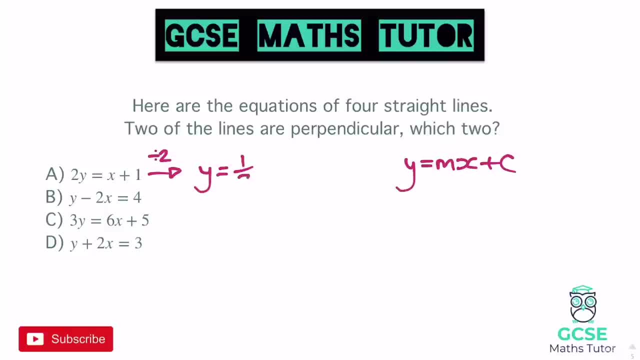 so that 1x would become a half x and the 1 divided by two at the end would become a half. so that's plus a half. There you go: half x plus a half. So there's my first one. let's have a look at the next. 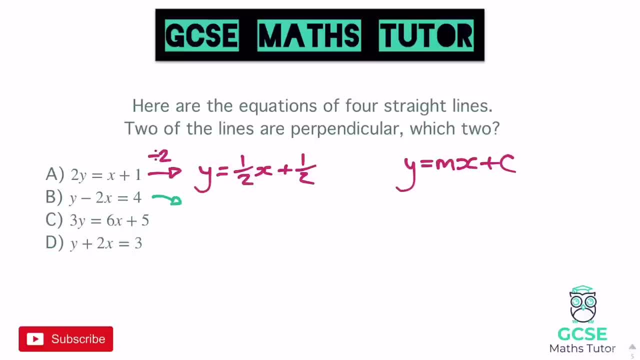 one. Now, this doesn't have anything in front of the y, but it does need rearranging. Look, the x there is on the left hand side of the equal sign. So if we add or plus 2x to both sides, we would get y equals. and just to keep it so that the x 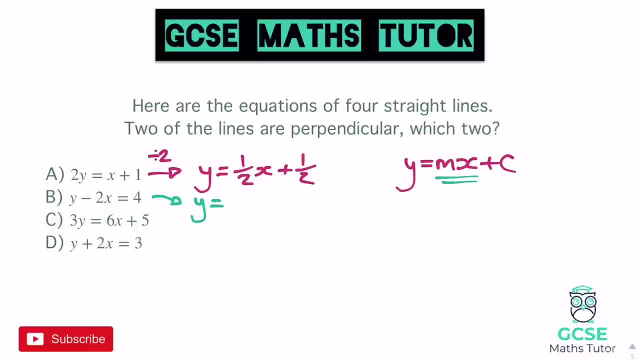 part's here. although I don't have to, I'm going to stick it in front of the 4.. So y equals positive 2x. so as it's in front of the 4, I don't have to put the plus sign. There we go, we get 2x, and then 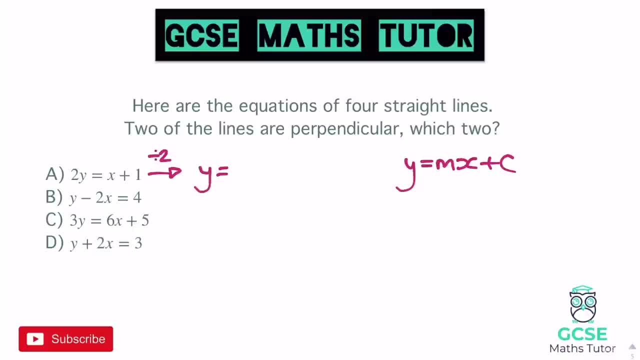 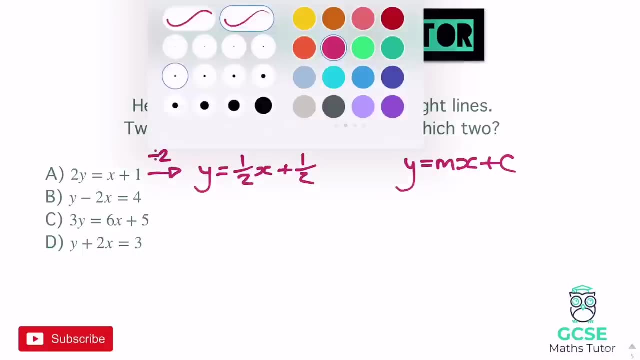 We've got one x there. One divided by two is a half, So that one x would become a half x, And the one divided by two at the end would become a half. So that's plus a half. There you go: Half x plus a half. So there's my first one. Let's have a look at the next one. 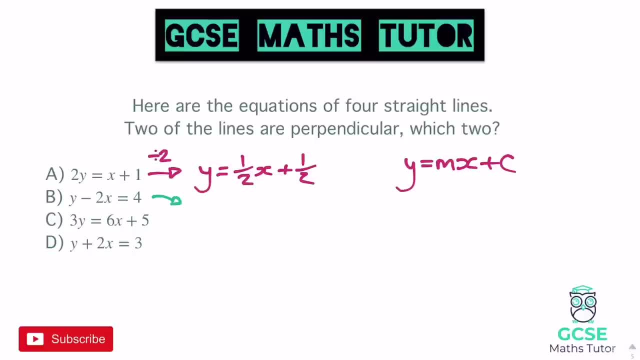 Now this doesn't have anything in front of the y, but it does need rearranging. Look, the x there is on the left hand side of the equal sign. So if we add a plus two x to both sides, we would get y equals mx plus c. So we've got one x there. One divided by two is a half, So that's. 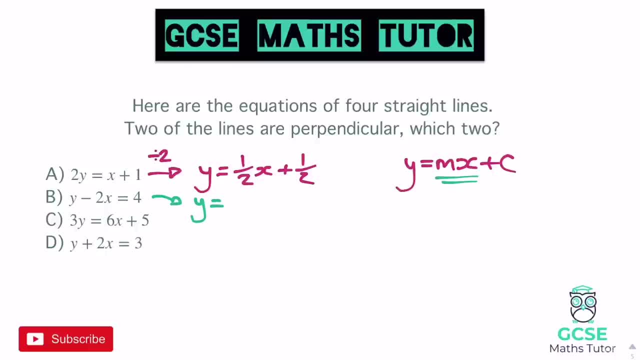 just to keep it so that the x part's here. although I don't have to, I'm going to stick it in front of the four. So y equals positive two x. So as it's in front of the four, I don't have to. 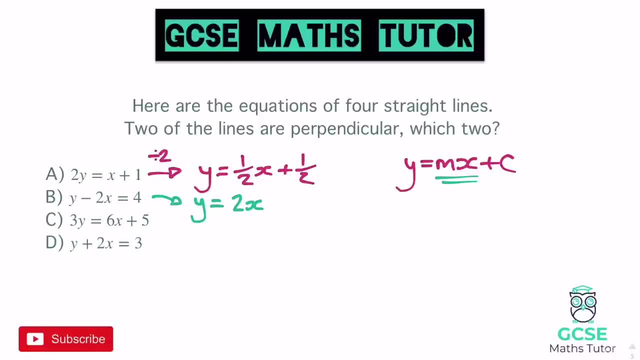 put the plus sign. There we go. We get two x, And then we do have to introduce the plus sign for the four there. So plus four, as it is positive four. There we go, Two x plus four, And that's my. 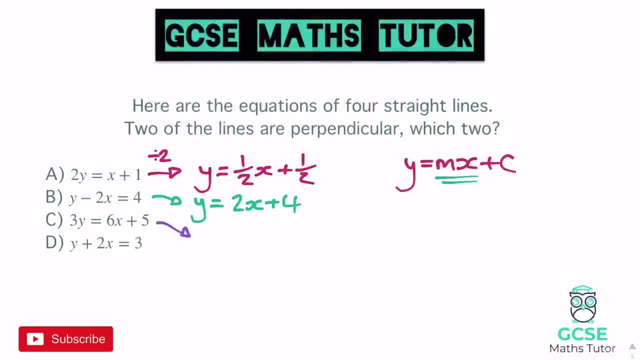 second one. Let's have a look at the third one, What we're going to do for this one. Okay, so we've got a three in front of the y, So we need to divide everything by three so that it says y equals. Don't have to rearrange it at all. 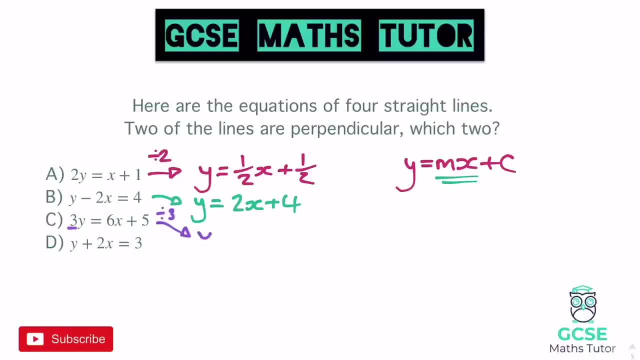 by three. So dividing that by three we get y equals six divided by three is two. So two x, six. x divided by three is two x. And then add five and five divided by three. Let's leave that as a fraction. five over three, That just means five divided by three there. 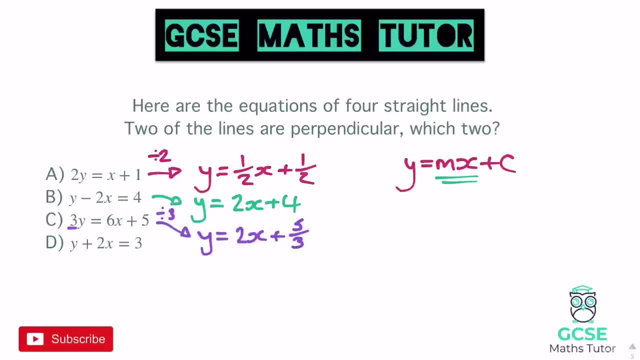 rather than trying to actually work that out. So five over three is fine. as we are also looking at the gradients here to decide which two are perpendicular, because that's what we're going to have a look at- which one's a perpendicular, We don't really need to worry about the y intercept. 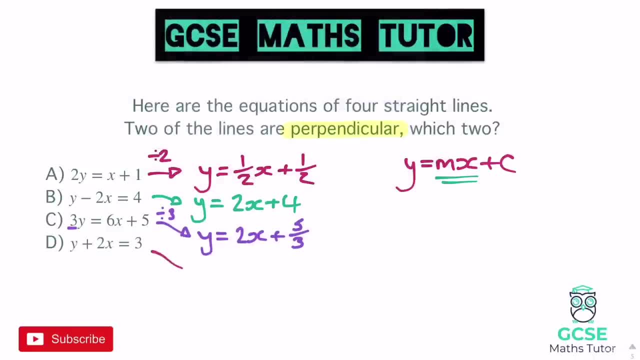 there. Okay, There we go. Let's have a look at this last one. Okay, So nothing in front of the y, but the two x is in the way here, So we need to minus two x from both sides to get that out. 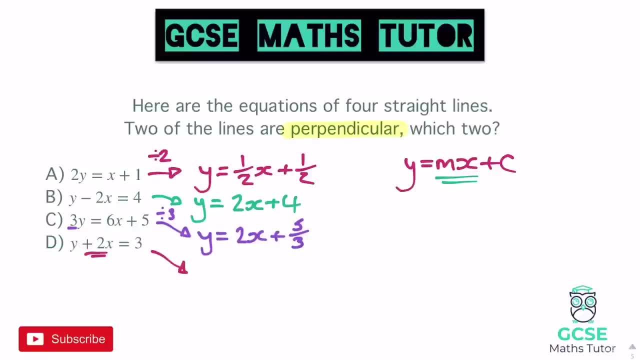 of the way, And again, just like before, I'm going to put it in front of the three. So y equals we're subtracting two x, so minus two x. There we go, And then that is positive three again. so plus three, Right? So we need to have a look at which ones of these are. 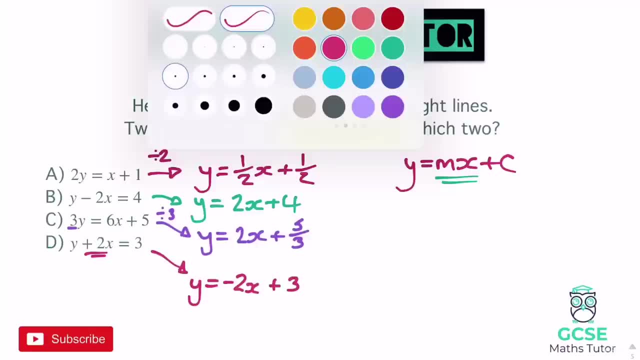 perpendicular. Now, as we've got- and let's see if we can highlight this- we've got a two x and a two x here. So those are two x and a two x. So those are two x and a two x. 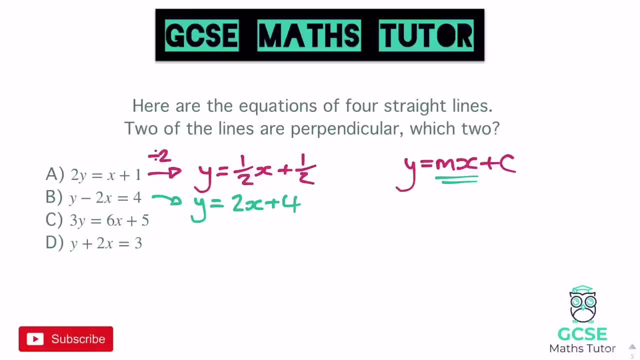 we do have to introduce the plus sign for the 4 there. so plus 4, as it is positive 4.. There we go, 2x plus 4, and that's my second one. Let's have a look at the third one, what we're going to do for. 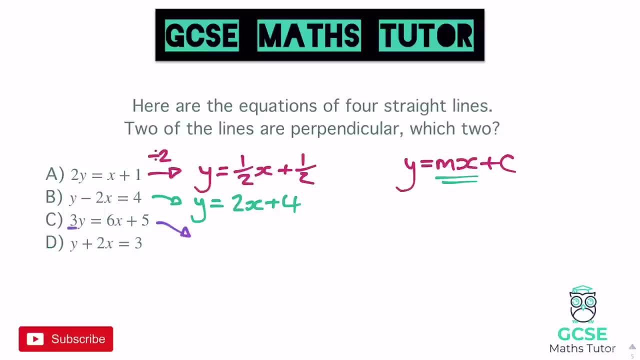 this one. Okay. so we've got a 3 in front of the y, so we need to divide everything by 3 so that it says y equals- Don't have to rearrange it at all, but dividing everything by 3.. So dividing that by 3, we get y equals. 6 divided by 3 is 2, so 2x, 6x divided by 3. 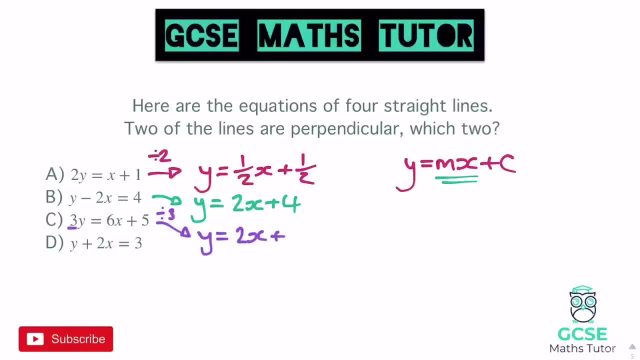 is 2x and then add 5 and 5 divided by 3. let's leave that as a fraction: 5 over 3.. That just means 5 divided by 3 there, rather than trying to actually work that out. So 5 over 3 is fine. 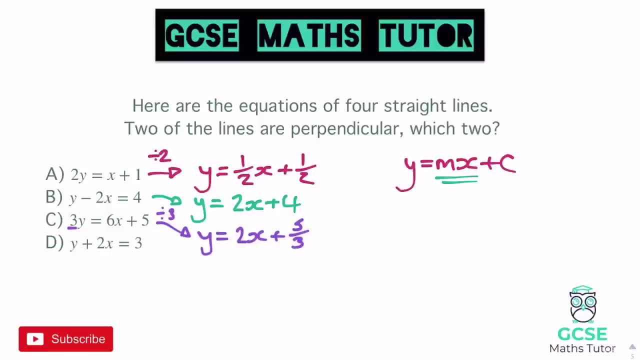 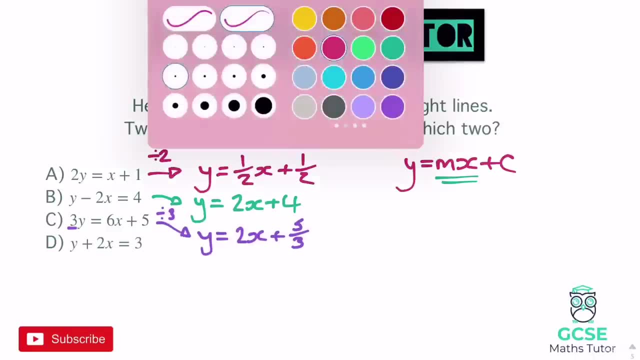 as we are also looking at the gradients here to decide which two are perpendicular, because that's going to have a look at which one's a perpendicular. We don't really need to worry about the y intercept there. Okay, but there we go. let's have a look at this last one. Okay, so nothing in front. 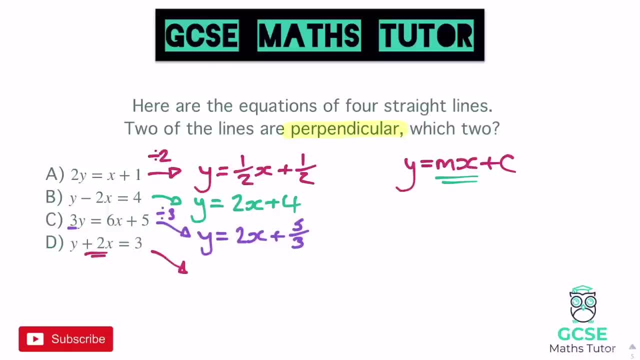 of the y, but the 2x is in the way here, so we need to minus 2x from both sides to get that out of the way, and again, just like before, I'm going to put it in front of the 3.. So y equals we're. 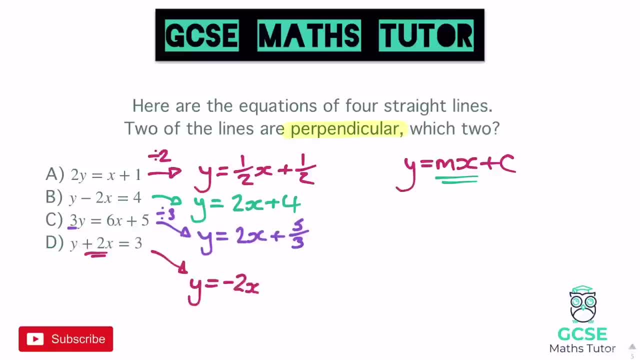 subtracting 2x, so minus 2x. there we go, and then that is positive 3 again, so plus 3.. Right, so we need to have a look at which ones of these are perpendicular. Now, as we've got- and let's see if we can highlight this- we've got a 2x and a 2x here, so those two 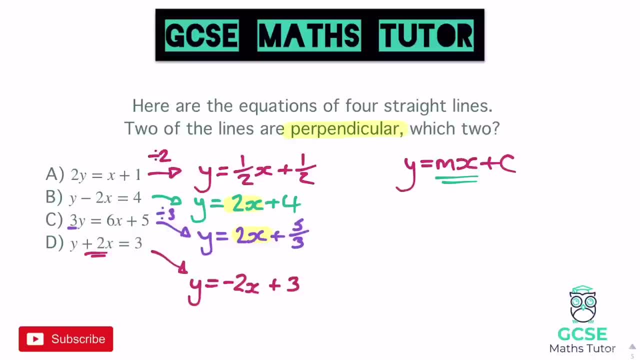 lines there are parallel. I'm not asking for which ones are parallel, but they have the same gradient, so we could say that those two are parallel. So let's have a look at the other two. So we've got these two here. So the gradient of the one at the top, so the gradient of a, is a half and the 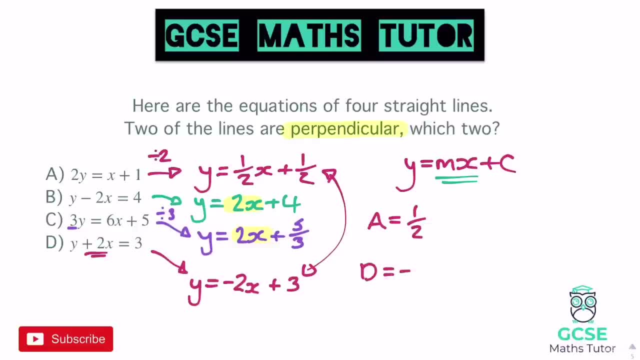 gradient of d down the bottom, there is negative 2. and if we think about this, how do I, if I, if half my negative reciprocal would be negative 2, wouldn't it? you'd flip it over, it'd be negative 2 over 1, which is negative 2, so therefore those two lines must be perpendicular. Okay, so it's just something. 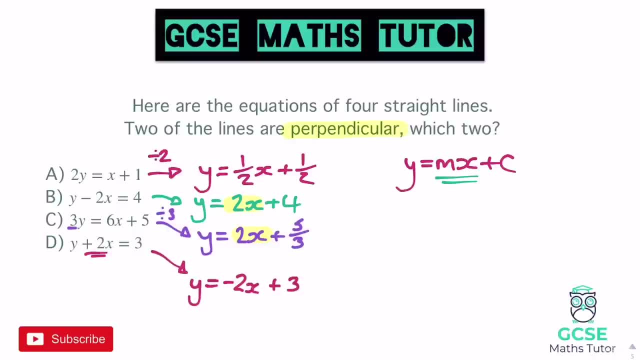 Those two lines there are parallel. Not asking for which ones are parallel, but they have the same gradient. So we could say that those two are parallel. So let's have a look at the other two. So we've got these two here. So the gradient of the one at the top. so 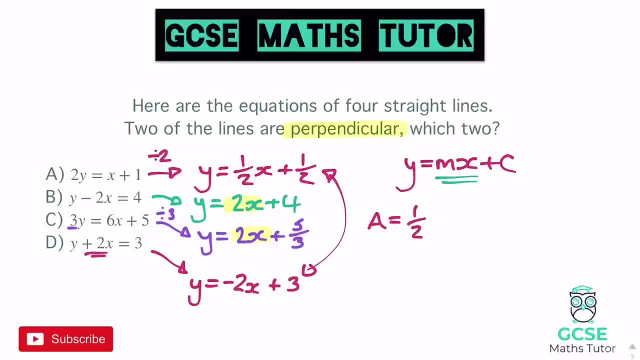 the gradient of A is a half and the gradient of D down the bottom, there is negative two. And if we think about this, how do I? if half is my gradient, my negative reciprocal would be negative two, wouldn't it? You'd flip it over, It'd be negative two over one. So 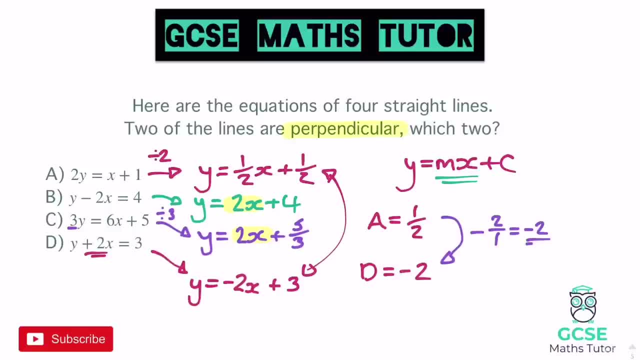 it's negative two over one which is negative two. So therefore, those two lines must be perpendicular. Okay, So it's just something to be thinking about in terms of different line equations, what they can look like in the way we want to have them. We want to have. 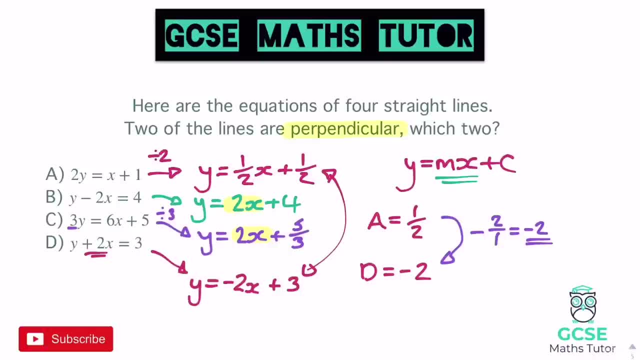 them as y equals. We don't want any numbers in front of the y. If we do, we're never going to divide it, And if there's anything next to the y, we just want to move it over to the other side. Okay, But they're A and D there and my two lines are perpendicular. 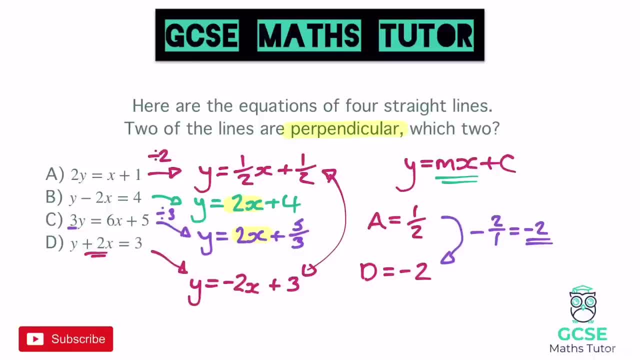 But we're going to be having a look at some line equations next, where they might not necessarily already be in the form: y equals mx plus c, And that just hints at some of the ST that you do have to change them first. Let's have a look at one, though, so you can. 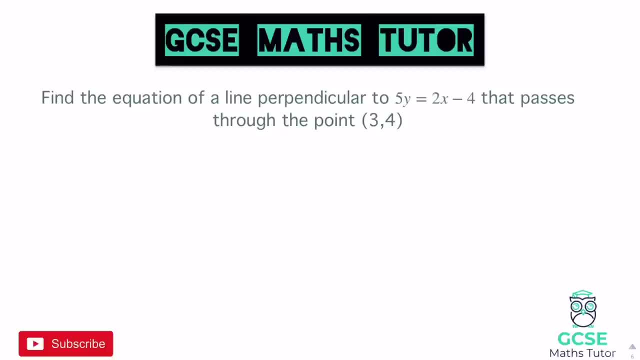 have a go, Okay. So this question says: find the equation of a line perpendicular to 5y equals 2x minus 4, and that passes through the point 3, 4.. Okay, So here's our line equation. 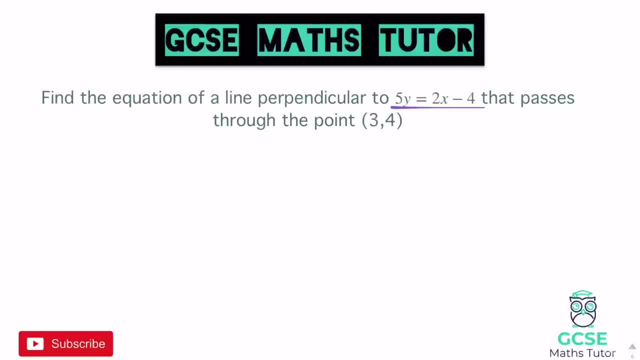 5y equals 2x minus 4.. So to eliminate that 5y there, just to make sure we've got a 1y, we're going to divide everything by 5. And let's see what we get when we do that We. 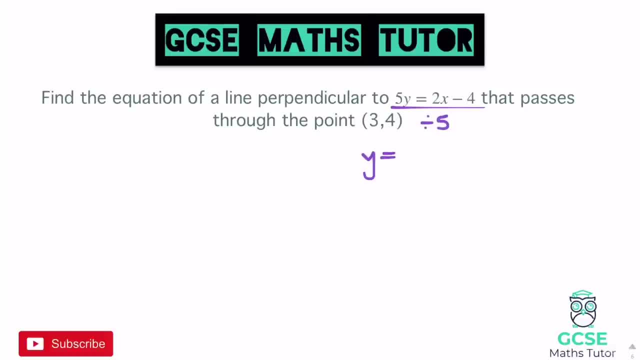 definitely get. our y equals 2 divided by 5 isn't very nice. We could write that as a decimal if you want, but I'm just going to leave it as a fraction. And the reason I tend to leave it as a fraction, particularly to start with, is it's a lot. 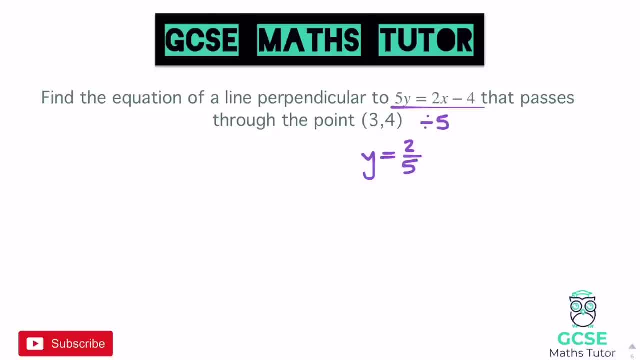 easier to do negative reciprocal of a fraction than it is as a decimal. In fact, if I did have it as a decimal, I'd actually convert it back to a fraction so that I could do my negative reciprocal there. But we get 2 fifths x minus and not that we're going to need. 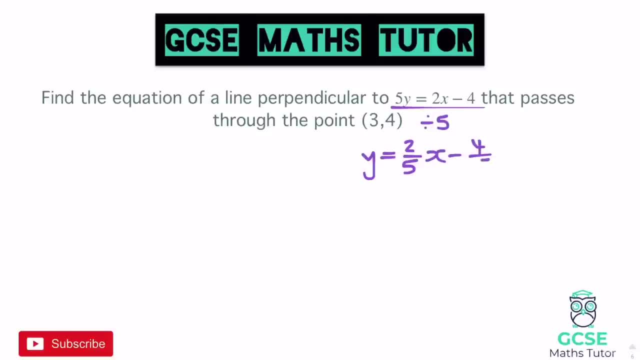 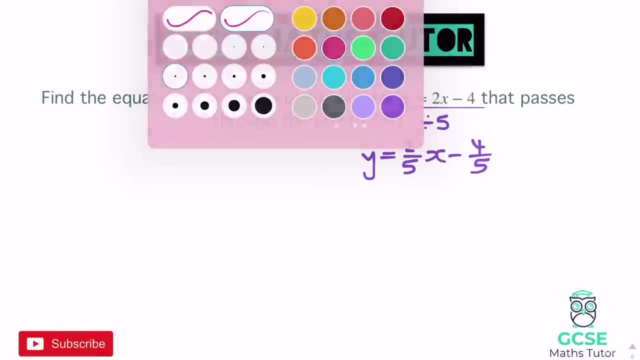 the y intercept. but let's get it right 4 over 5 as well, just dividing it by 5.. So that is the equation of the line that we want, because we can now do our gradient negative reciprocal here. So our gradient at the moment is 2 fifths our number. 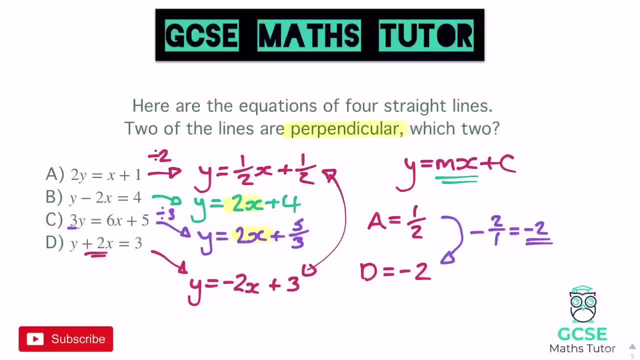 to be thinking about in terms of different line equations, what they can look like in the way we want to have them. We want to have them as y equals. we don't want any numbers in front of the y. if we do, we're never going to divide it, and if there's anything next to the y, we just want to move it. 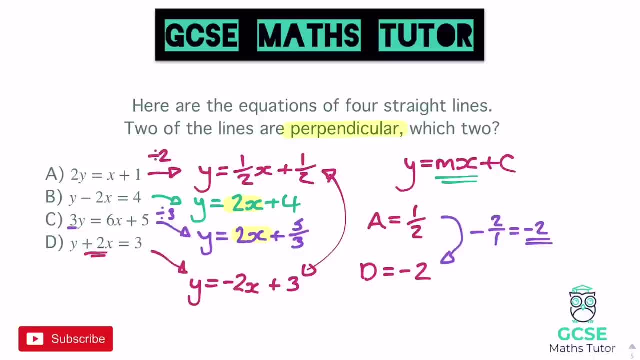 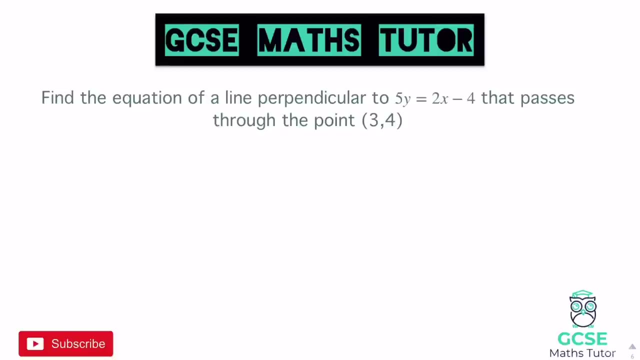 over to the other side. Okay, but they're a and d. there are my two lines that perpendicular, but they're a and d. there are my two lines next, where they might not necessarily already be in the form. y equals mx plus c, and that just hints to you that you do have to change them first. Let's have a look at one, though, so you can have a go. Okay, so this question says: find the equation of a line perpendicular to 5y equals 2x minus 4, and that passes through the point 3, 4.. Okay, so here's our line equation: 5y equals 2x minus 4.. So to eliminate that 5y there, just to make sure we've got a 1y, we're going to divide everything by 5 and let's see what we get when we do that. 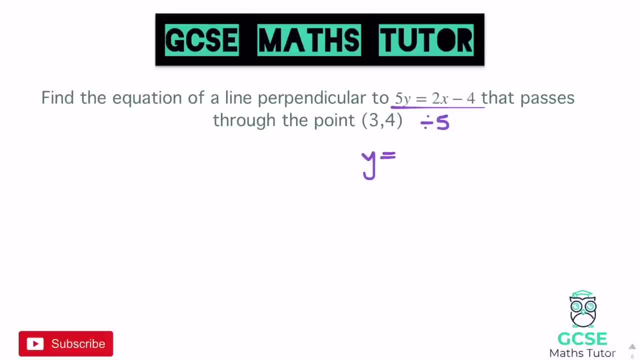 We definitely get our y equals. 2 divided by 5 isn't very nice. we could write that as a decimal if you want, but I'm just going to leave it as a fraction. and the reason I tend to leave it as a fraction, particularly to start with, is it's a lot easier to do negative reciprocal of a fraction than it is as a decimal. In fact, if I did have it as a decimal, I'd actually convert it back to a fraction so that I could do my negative reciprocal there. But we get 2 fifths x minus, and not that we're going to need the y intercept. but let's get it right 4 over 5 as well, just dividing it by 5.. 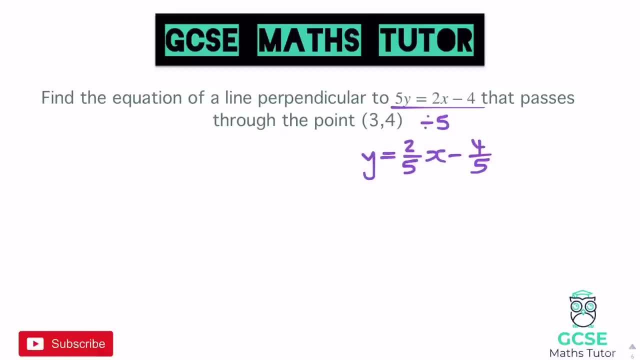 So that is the equation of the line that we want, because we can now do our gradient negative reciprocal here. So our gradient at the moment is 2 fifths our number in front of x there and our negative reciprocal of that. if we flip it over and change the symbol, we get minus 5 over 2.. There we go, which we could also write as minus 2 and a half or 2.5 and convert it if you want, but I'm just going to leave it as 5 over 2 for the moment. 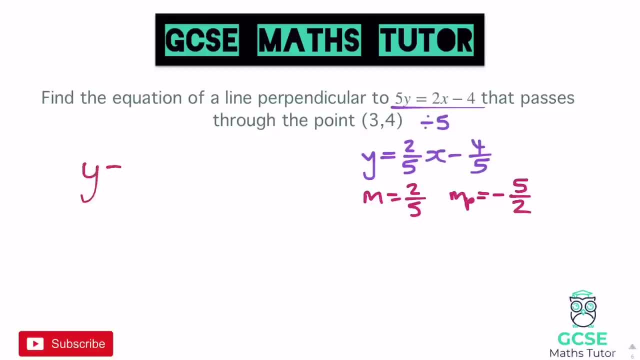 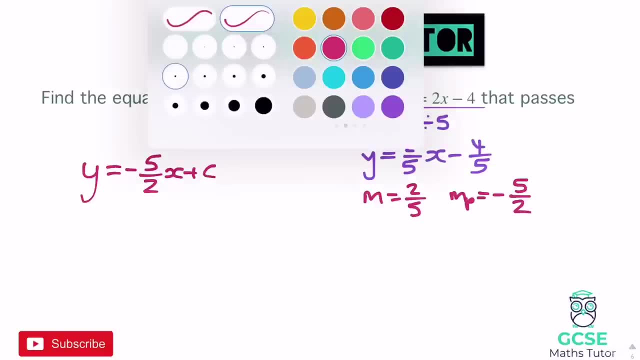 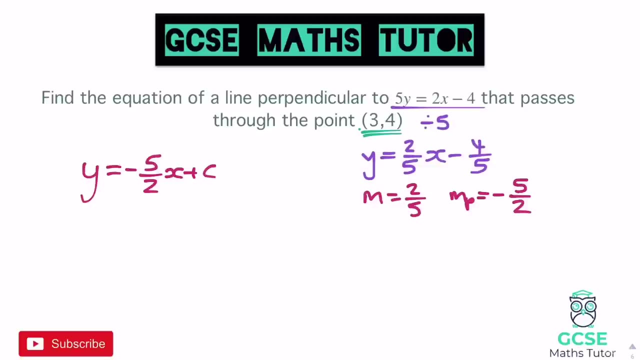 Alright, let's put that into our line equation then. So y equals minus 5 over 2, x plus c, So same as before. we're going to sub this point in, use that to help us find c, but we've not got a nice gradient for this one. we've got minus 5, halves, or 5 over 2 or 2.5, if you want to convert it. 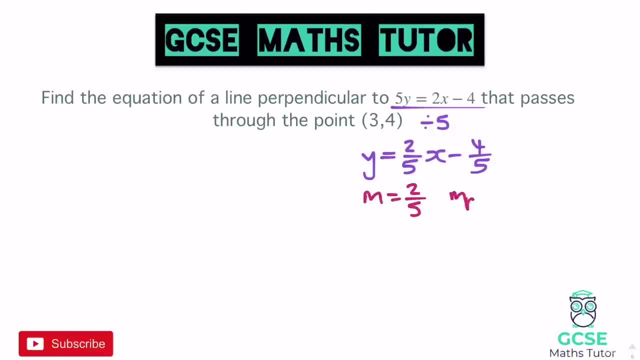 in front of x there and our negative reciprocal of that. if we flip it over and change the symbol, we get minus 5 over 2.. There we go, which we could also write as minus 2 and a half or 2.5, and convert it if you want, but I'm just going to leave it as 5 over 2 for. 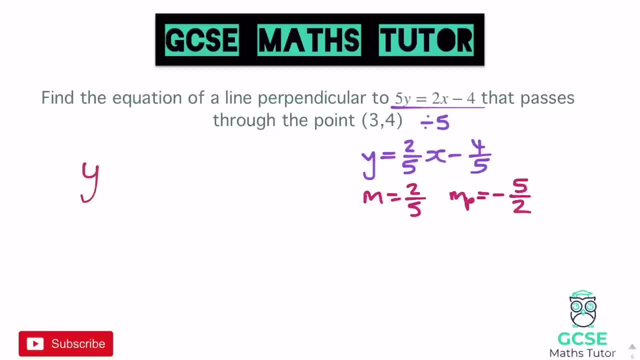 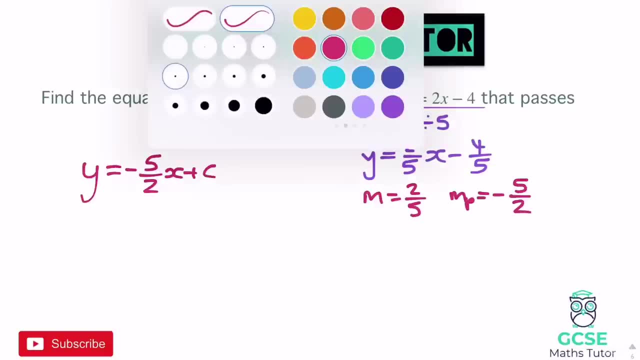 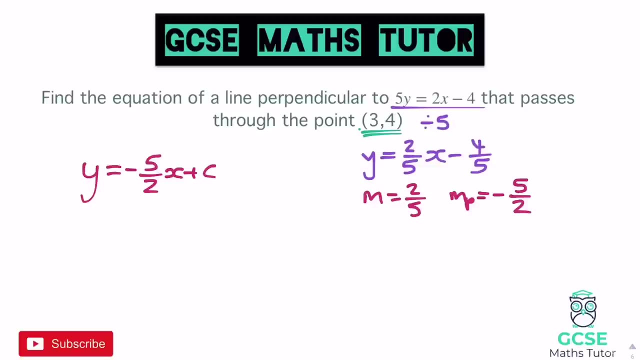 the moment. All right, let's put that into our line equation then. So y equals minus 5 over 2.. Plus c: So same as before. we're going to sub this point in. use that to help us find c, but we've not got a nice gradient for this one. We've got minus 5 halves, or 5 over 2,. 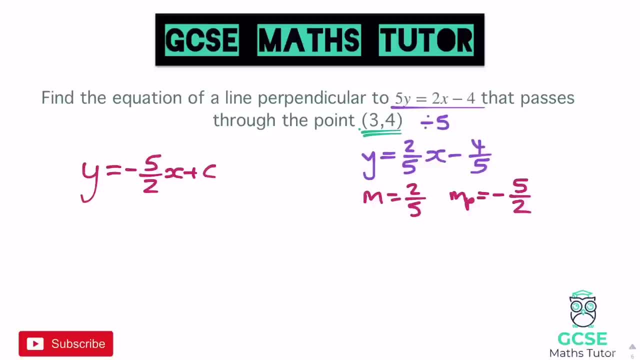 or 2.5. if you want to convert it, I'm just going to leave it as it is, So sticking our coordinates in: y is 4, so 4 equals negative 5 over 2 times 3, so subbing in 3, plus c. 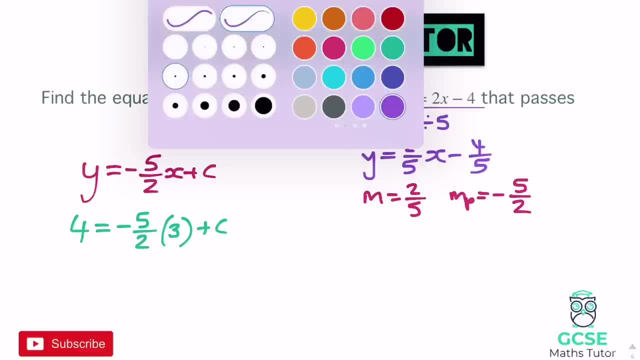 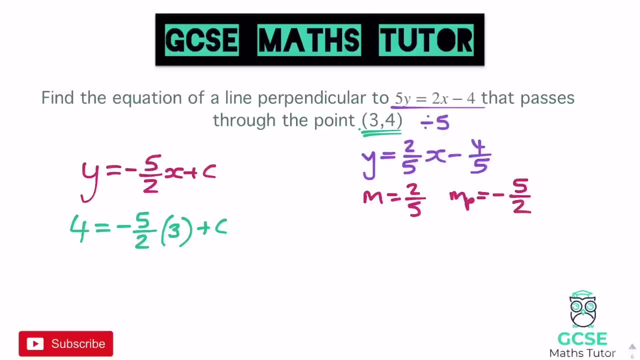 Now you might make the case here that it might be easier as a decimal, but if it's not this 2.5 or it's something else, you're going to want to leave it as a fraction. So you might think at this point: okay, well, I'll probably just do 2.5 times 3,, which is quite nice, and 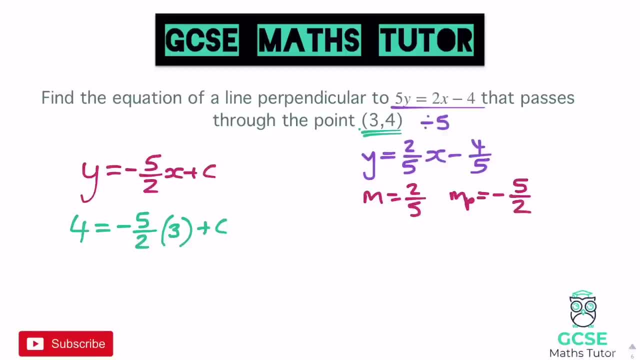 easy to do. I'm actually going to avoid doing that for the moment. I'm just going to leave it in fractional form. It just makes it a bit easier with some of the harder questions where maybe the decimals aren't as nice if it's thirds or if it's sevenths or something. 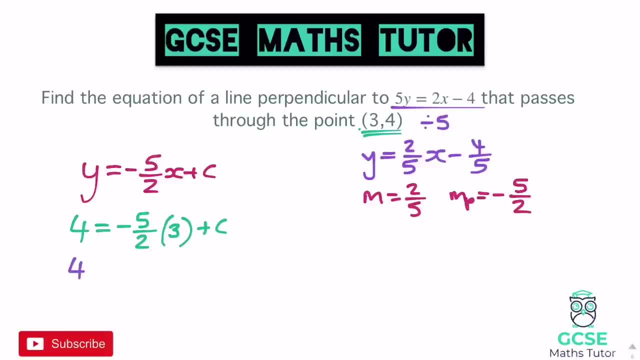 like that, Right, so let's work it out. So 4 equals negative 5 over 2 times 3.. We'll just always just imagine this as a fraction times the top, times the bottom, So we've got negative 5.. 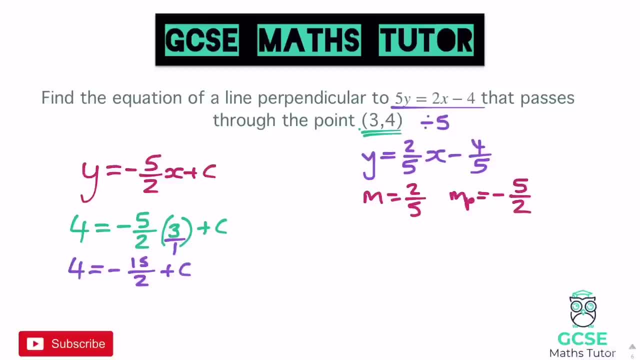 15 over 2 plus c. There we go: Minus 15 over 2.. Obviously, if it's not a nice decimal here, you can actually just convert that into a mixed number. Okay, so minus 15 over 2 is the same as minus 7.5.. 2 goes into 15 seven times, with a remainder of 1.. So let's just 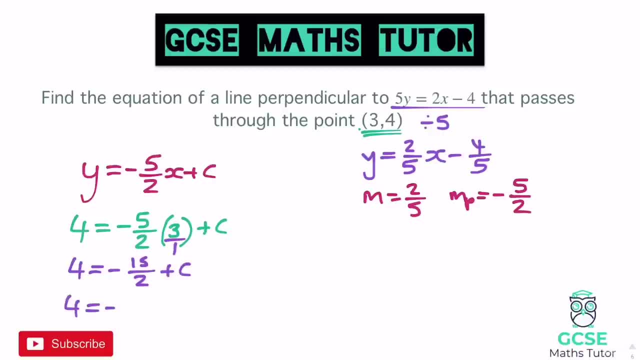 rewrite that. So 4 equals minus 7.5 plus c, And that's just quite nice and easy now to add to 4,, isn't it? So we can add 7 to 4. Which is 11.. Add the extra half, which is 11.5.. So if we add 7.5 to both sides, we get 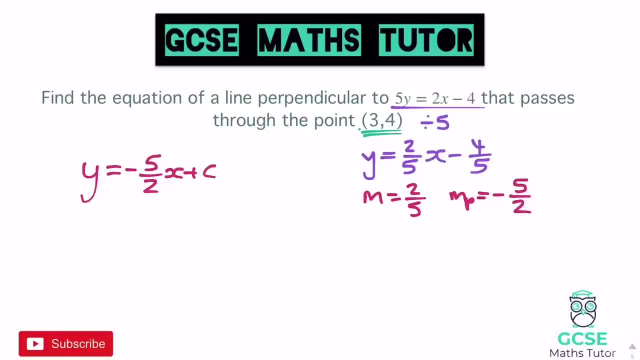 I'm just going to leave it as it is. So sticking our coordinates in y is 4, so 4 equals negative 5 over 2 times 3, so subbing in 3 plus c. Now you might make the case here that it might be easier as a decimal, but if it's not this kind of fraction here, where it is 2.5 or it's something else, you're going to want to leave it as a fraction. so you might think at this point: okay, well, I'll probably just do 2.5 times 3, which is quite nice and easy to do. 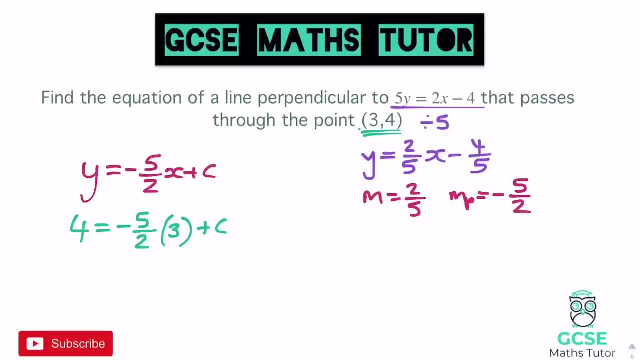 I'm actually going to avoid doing that for the moment, though I'm just going to leave it in fractional form just makes it a bit easier with some of the harder questions, where maybe the decimals aren't as nice if it's thirds or if it's sevenths or something like that. 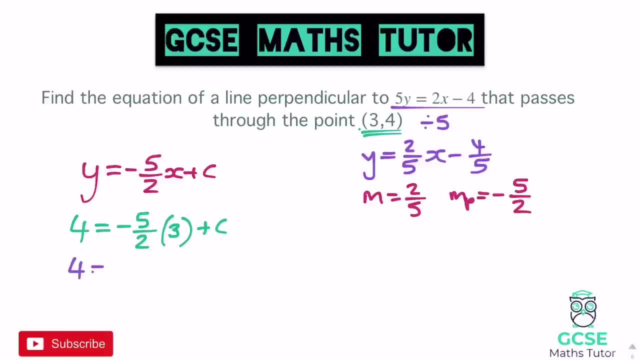 Right, so let's work it out. So 4 equals negative 5 over 2 times 3.. Well, just always, Just imagine this as a fraction times the top, times the bottom. so we've got negative 15 over 2, plus c. 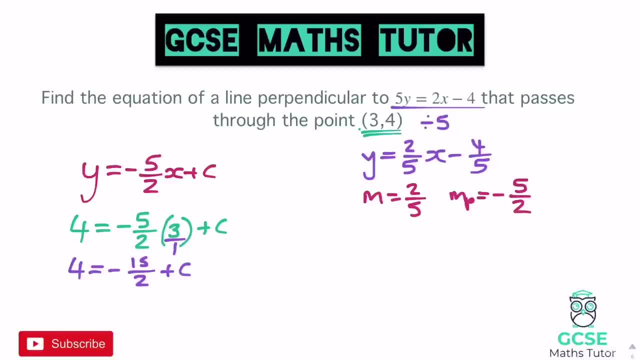 There we go: Minus 15 over 2.. Obviously, if it's not a nice decimal here, you can actually just convert that into a mixed number. Okay, so minus 15 over 2 is the same as minus 7 and 1 half. 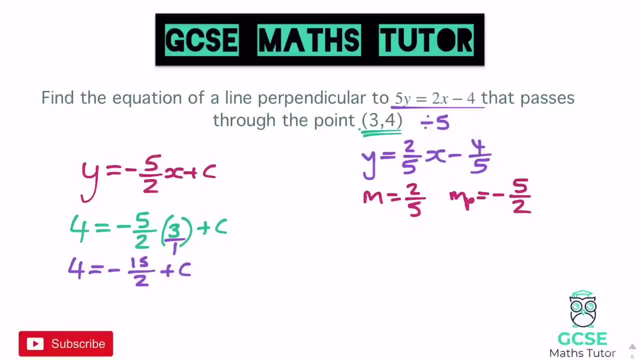 2 goes into 15, 7 times, with a remainder of 1.. So let's just rewrite that. So 4 equals minus 7 and a half Plus c, And that's just quite nice and easy now to add to 4, isn't it? 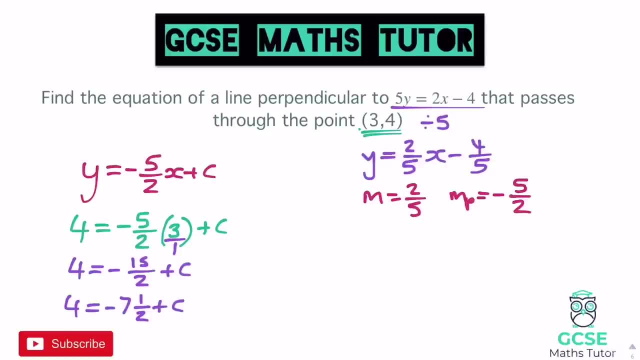 So we can add 7 to 4, which is 11.. Add the extra half, which is 11 and a half. So if we add 7 and a half to both sides, we get c equals 11 and a half, Which again you could write as 11.5.. 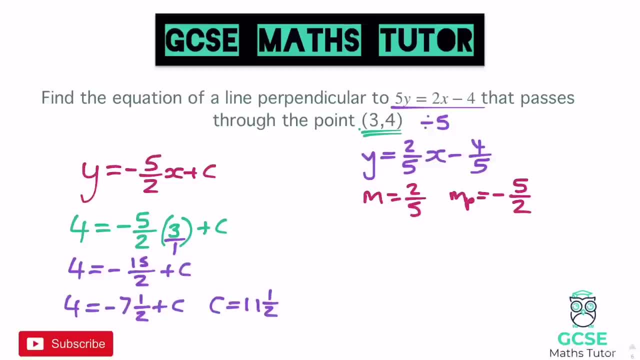 But just for the case of some of the harder questions, I'm going to leave it as a fraction Right. so plugging that in in place of c, We get y equals minus 5 over 2x, Plus 11 and a half. 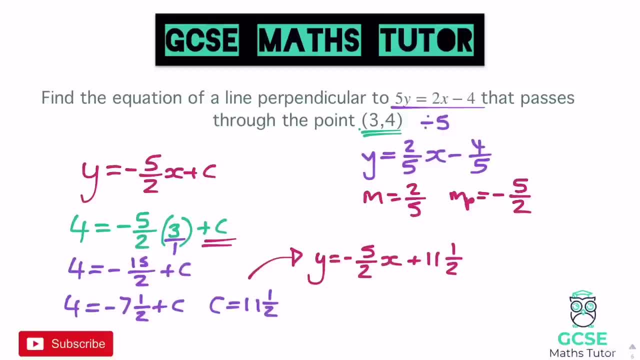 There we go, And there's our final answer. A little bit weird there actually to have it as mixed numbers and improper fractions there, So I probably would change that. I'd probably put: y equals negative 2 and a half, x Plus 11 and a half. 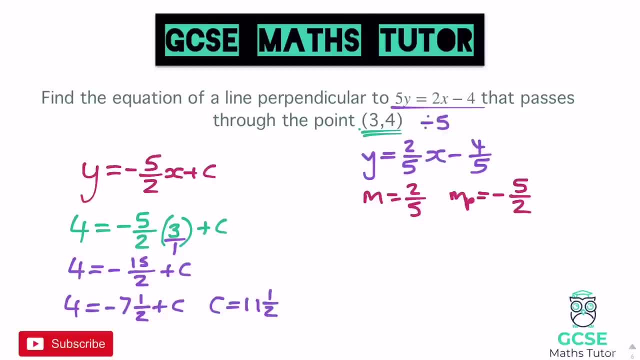 c equals 11.5, which again you could write as 11.5.. But just for the case of some of the harder questions, I'm going to leave it as a fraction Right. so, plugging that in in place of c, we get y equals minus 5 over 2x plus 11.5.. There we go, And there's our. 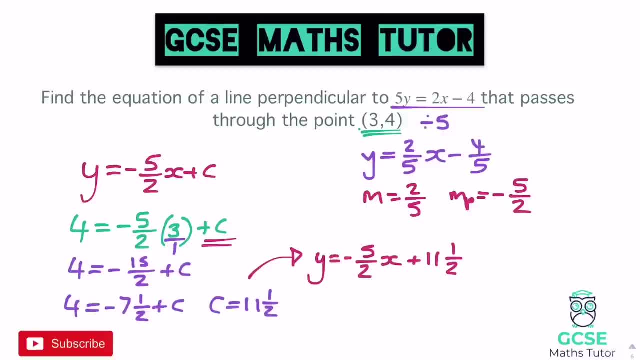 final answer. So I figured there actually to have it as mixed numbers and improper fractions there. So I probably would change that. I'd probably put: y equals negative 2.5x plus 11.5.. There we go. It wouldn't actually be wrong to leave it how I already had, but I just don't really. 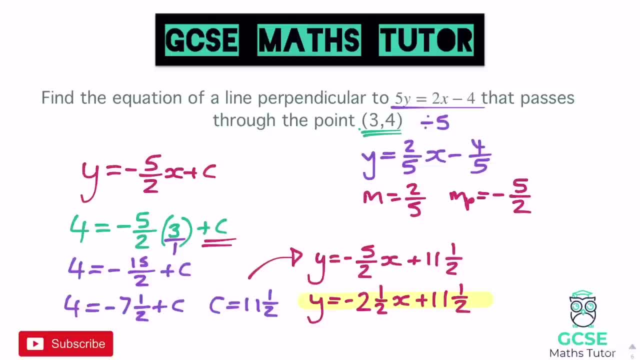 like to have improper fractions and mixed numbers in the same question. There we go. So y equals negative 2.5x plus 11.5.. Of course, again, you could write it as minus 2.5x plus 11.5.. Absolutely fine to write. 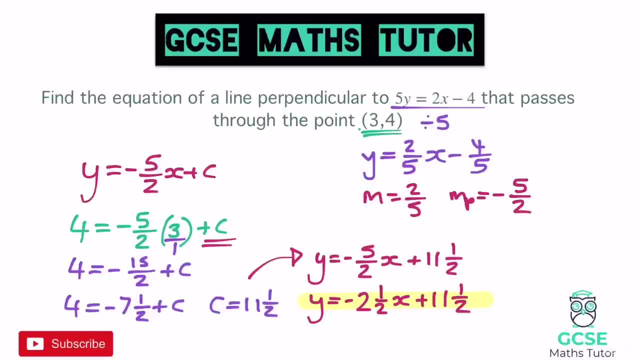 Final answer is a decimal Right. So just a little bit, little bits to be thinking about there. Obviously, when you do get- and I'm just going to highlight it down here- when you do get this scenario going on, do just leave it as a fraction, Okay, And then convert. 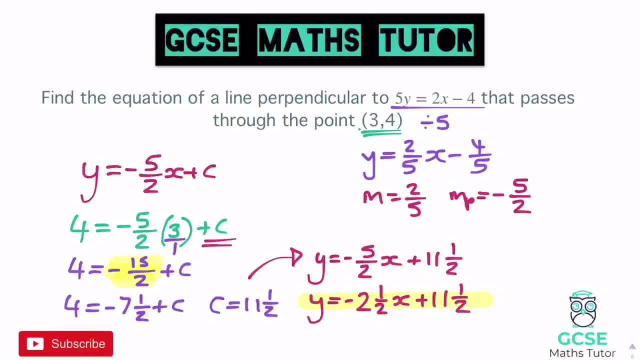 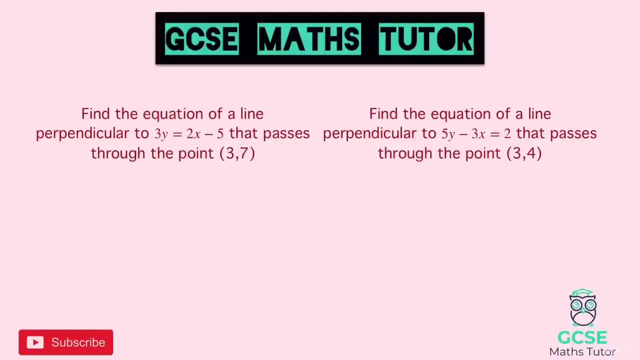 it back to a mixed number so that you can add it and find your c if that scenario does arise. I've got one here where it does arrive, So you can have a go at it now. So I'll flick to that, Okay, So there's two questions here. Have a go. Pause the video there and we'll. 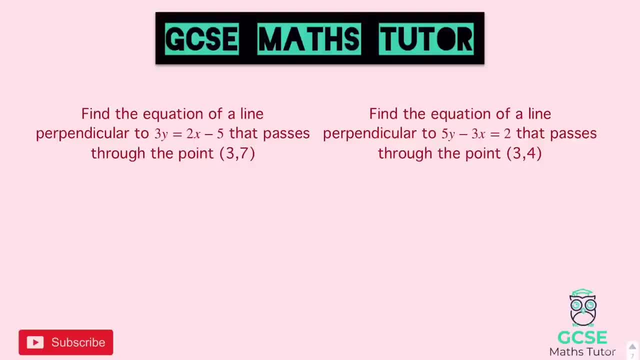 go over the answers in a sec, Right, Okay, So let's have a look at these. So the first one: find the equation of this perpendicular line to this one And it goes through this point here. So first of all we need to divide it by three, So y equals. 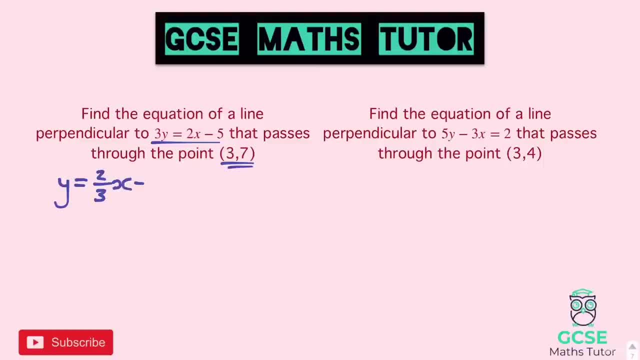 two divided by three is two thirds, And five divided by three is five over three. There we go. So our gradient there at the moment is two thirds And our perpendicular gradient will be negative three over two. Flipping it over, Putting that into our line equation: 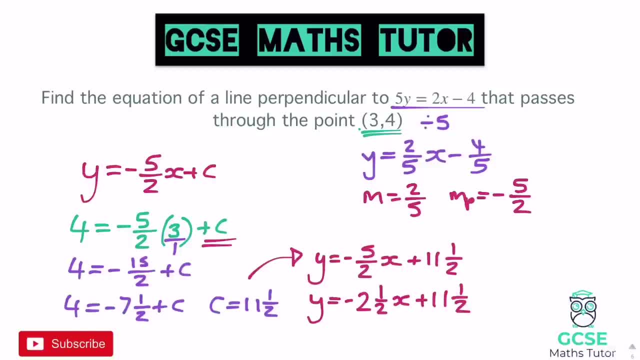 There we go. It wouldn't actually be wrong to leave it how I already had, But I just don't really like to have improper fractions and mixed numbers in the same question. There we go. So y equals negative 2 and a half x. 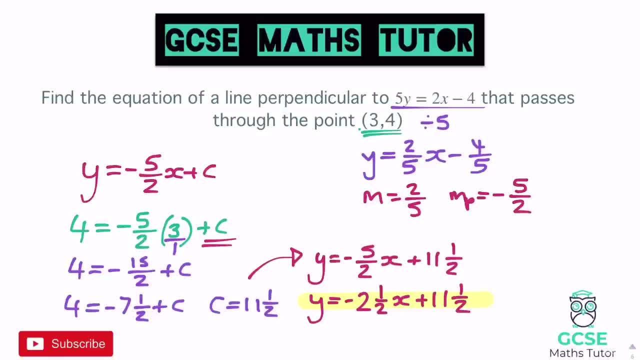 Plus 11 and a half. Of course, again you could write it as minus 2.5x plus 11.5.. Absolutely fine to write your final answer as a decimal Right. So just a little bits to be thinking about there. 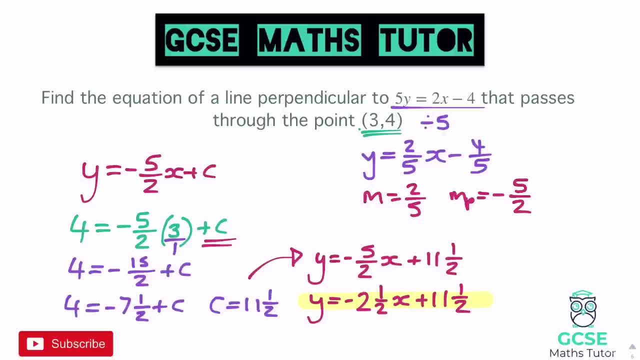 Obviously, when you do get- I'm just going to highlight it down here- When you do get this scenario going on, Do just leave it as a fraction, Okay, and then convert it back to a mixed number So that you can add it and find your c if that scenario does arise. 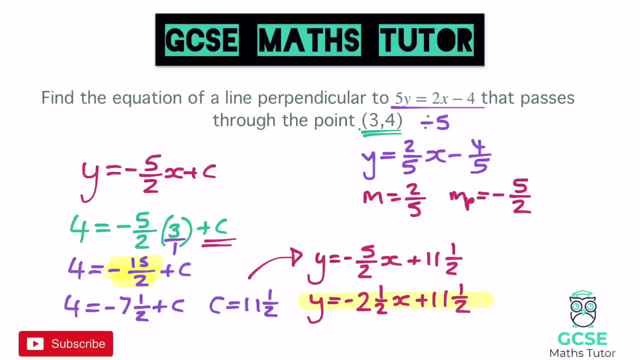 I've got one here, where it does arrive, So you're going to have a go at it now, So I'll flick to that. Okay, so there's two questions here. Have a go. Pause the video there And we'll go over the answers in a sec. 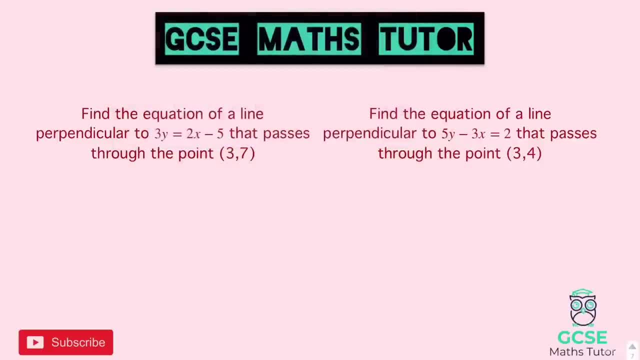 Right, okay, So let's have a look at these. So the first one Find the equation of this perpendicular line to this one And it goes through this point here. So first of all, we need to divide it by 3.. So y equals 2. divided by 3 is 2 thirds. 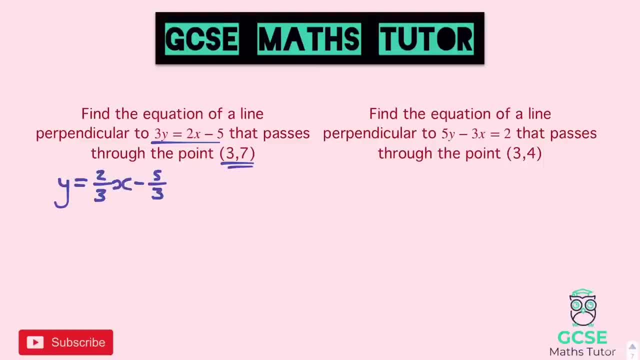 And 5 divided by 3 is 5 over 3.. There we go. So our gradient there at the moment is 2 thirds And our perpendicular gradient will be negative 3.. 3 over 2. Flipping it over. 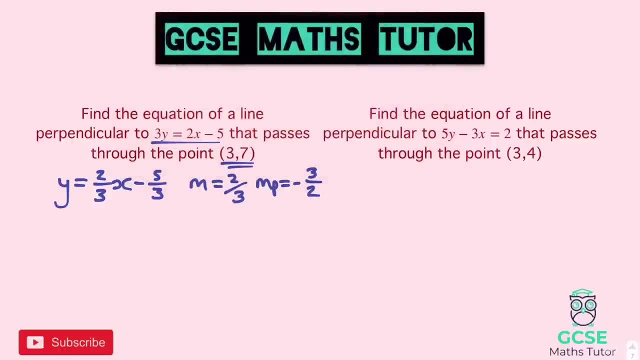 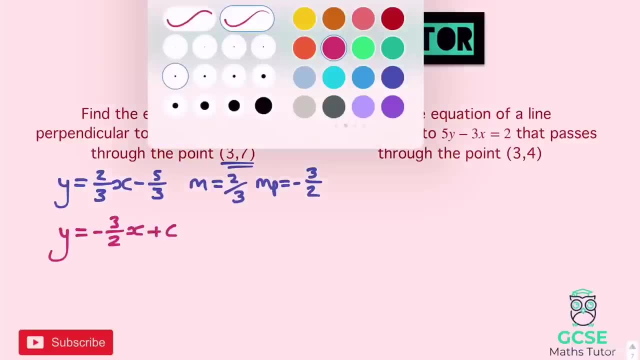 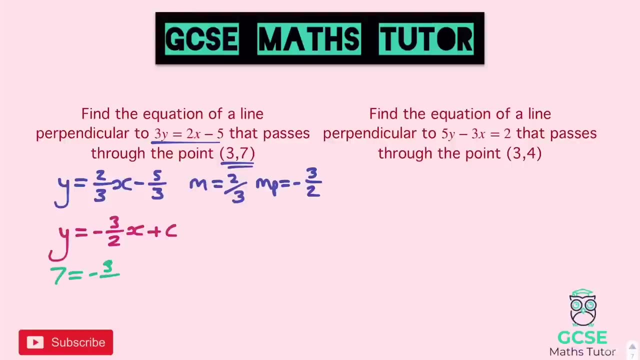 Putting that into our line equation. Let's have a look and see what we get here. So y equals negative 3 over 2x plus c, And now we can substitute that point in 3 and 7. So 7 equals negative 3 over 2 times 3 plus c. 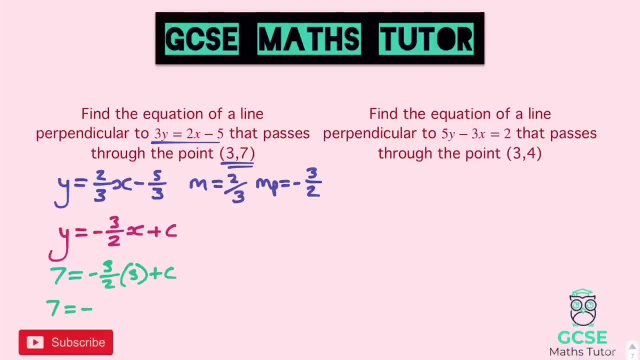 Times that out, We get 7 equals minus 3 times 3 over 2, is minus 9 over 2.. Plus c And that's 4 and a half or 4.5.. So if we add 4.5 or 4 and a half over to 7. 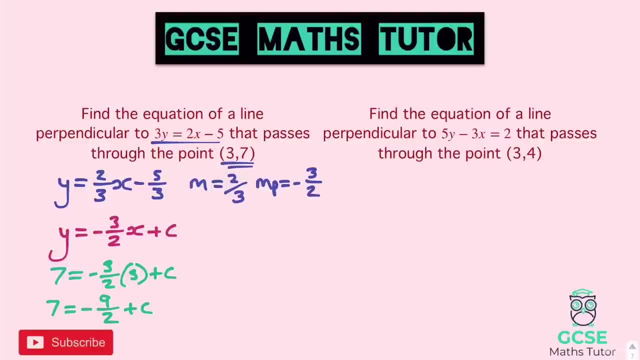 7 plus 4 is 11.. Plus the extra half is 11 and a half. So 11 and a half, or 11.5, equals c, And now we can plug that in place of the c up here Again, you can write it as you mix them with your decimals. 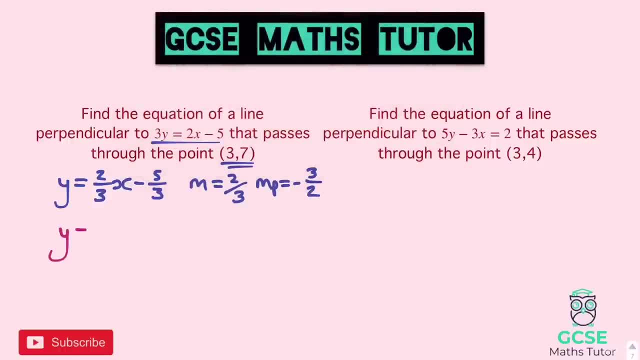 Let's have a look and see what we get here. So y equals negative three over two, x plus c. And now we can substitute that point in three and seven. So seven equals negative three over two times three plus c. Times that out, We get seven equals minus three times three over two is minus nine over two plus. 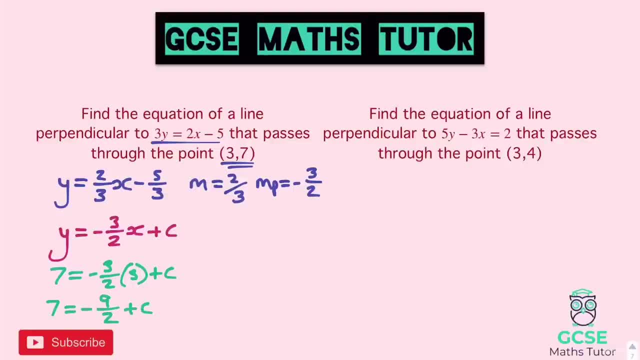 c, And that's four and a half or 4.5.. So if we add 4.5 or four and a half over to seven, seven plus four is 11 plus the extra half is 11 and a half. So 11 and a half or 11.5 equals c, And now we can plug that in. 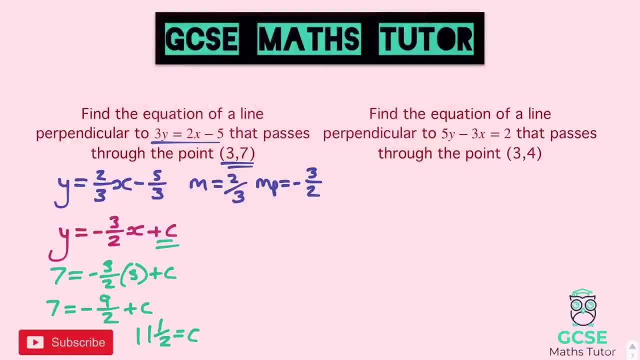 place of the c up here Again, you can write it as your mixed number, your decimals, Or you could have kept it top heavy if you'd have wanted, But let's write it all in. So: y equals minus one and a half, or three over two, Doesn't actually matter, Just personal. 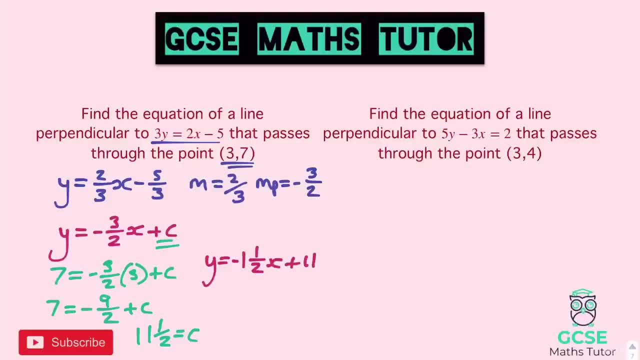 preference here And then plus the 11 and a half. There you go. So you could have written minus three over two x, Or you could have written minus 1.5 and 11.5 there. As long as it's the same numbers, it doesn't. 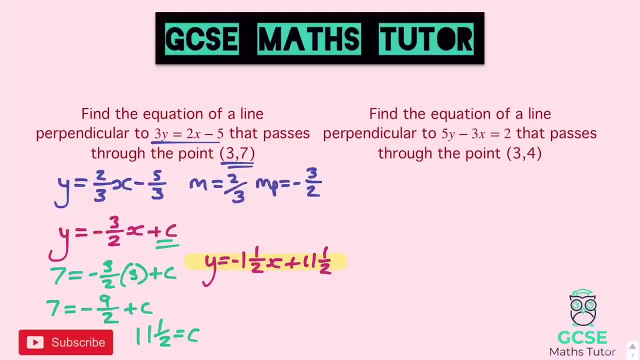 really matter how you write them. There we go And there's the equation of that line On to the next one. So at the moment it's not in the format we want. We need to add the three x over as well. So if we add that over, we get five. y equals three x plus two. 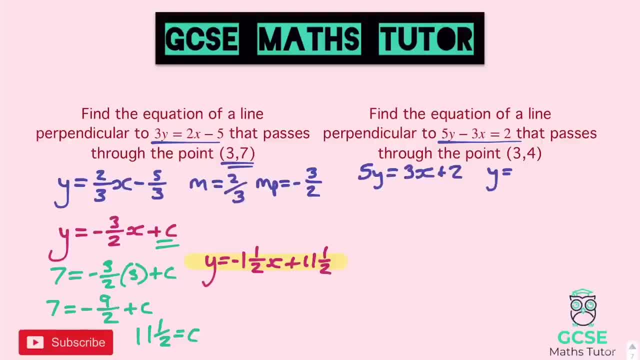 Divide everything by five, We get y equals three fifths, x, Three divided by five plus two fifths. We need that one at the end, But there we go And then we can write our gradient. So at the moment the gradient is three over five And our perpendicular gradient, if 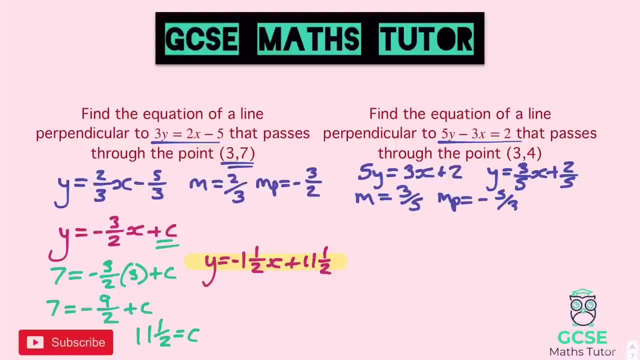 we flip that over, we get minus five thirds. So minus five thirds. Right, Let's put it in place. See what we get. So y equals minus five and a half. We get minus one and a half. So what we're going to do is write that one over to the other side And then we're going. 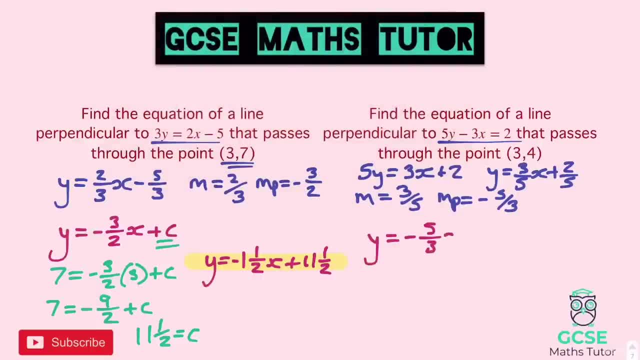 to add our gradient. So if we do that over, we get minus one and a half. So we get minus one and a half minus 5 thirds x plus c, and now let's sub in that coordinate there 3, 4.. So 4 equals. 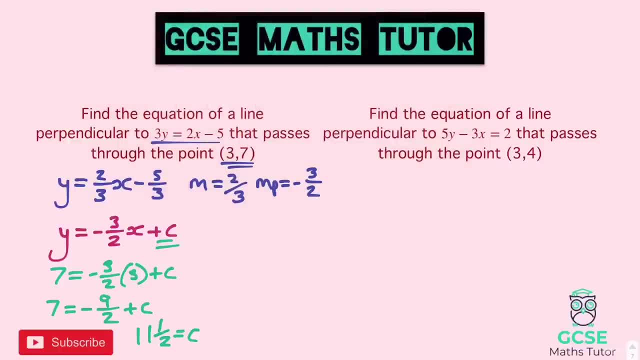 Or you could have kept it top heavy if you'd have wanted. But let's write it all in. So y equals minus 1 and a half or 3 over 2. Doesn't actually matter, Just personal preference here. And then plus the 11 and a half. 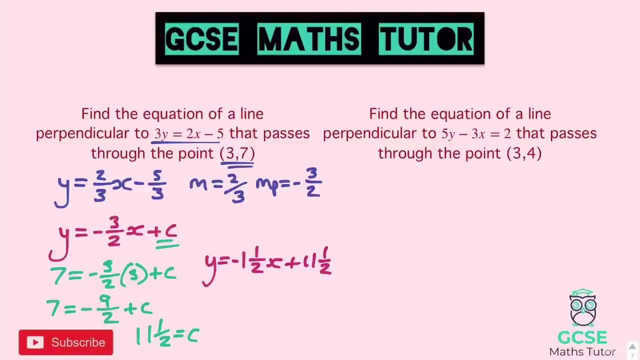 There you go. So you could have written minus 3 over 2x, Or you could have written minus 1.5 and 11.5 there. As long as it's the same numbers, Doesn't really matter how you write them. 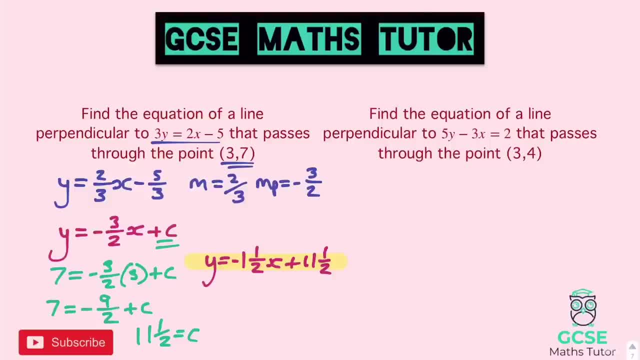 There we go, And there's the equation of that line On to the next one. So at the moment it's not in the format we want. We need to add the 3x over as well. So if we add that over, we get 5y. 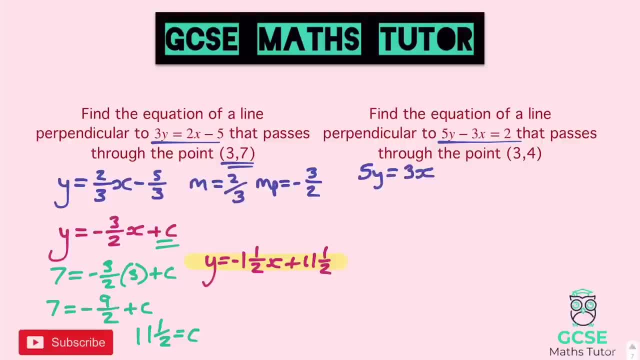 Y equals 3x plus 2.. Divide everything by 5. We get y equals 3 fifths x 3 divided by 5 plus 2 fifths. Not that we need that one at the end, But there we go. 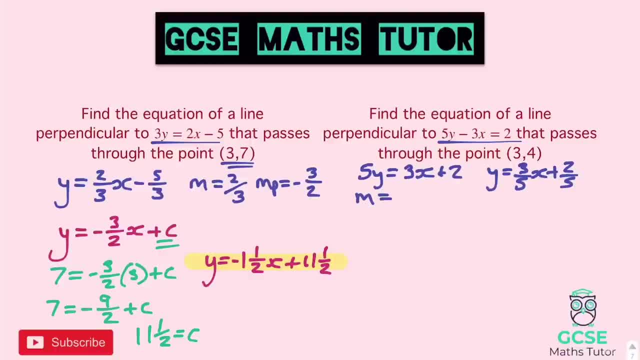 And then we can write our gradient. So at the moment the gradient is 3 over 5.. And our perpendicular gradient? If we flip that over, we get minus 5 thirds. So minus 5 thirds, Right, Let's put it in place and see what we get. 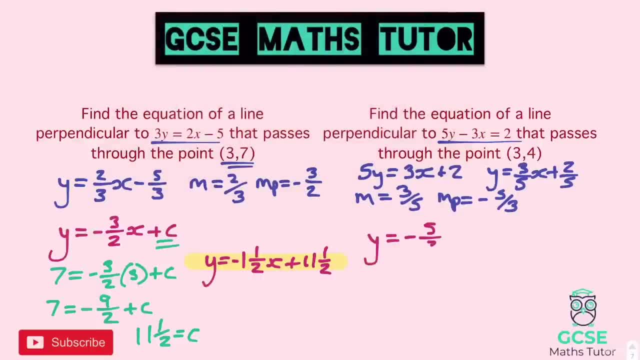 So y equals minus 5 thirds x plus c. And now let's sub in that coordinate there 3, 4.. So 4 equals minus 5 thirds times the x coordinate there, Which is 3 plus c. Let's times that out. 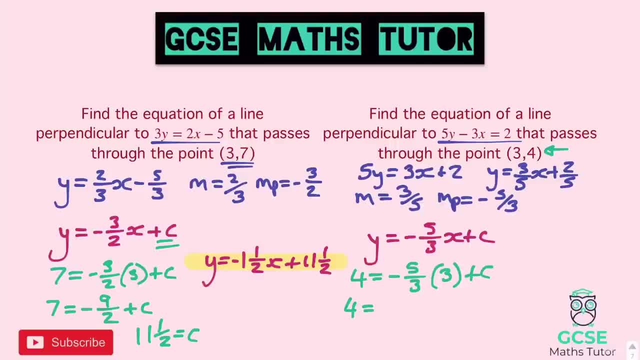 So 4 equals 3 times 5 on the top there, Remembering it's 3 over 1. So minus 15 over 3, plus c, 15 does actually divide by 3. So 15 over 3 becomes 5.. 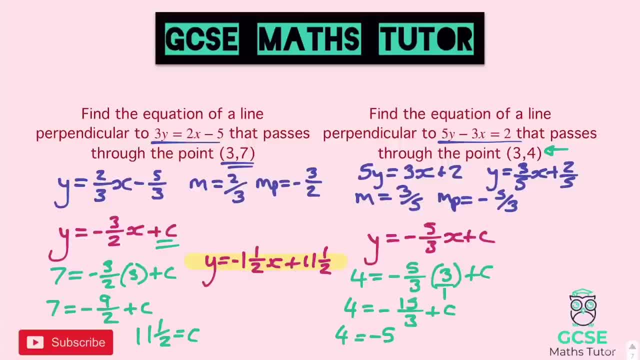 So we have 4 equals negative, 5 plus c, And adding 5 to both sides there we get 9 equals c Or c equals 9. And then again we can put that in place of c in our line equation. So what do we get? 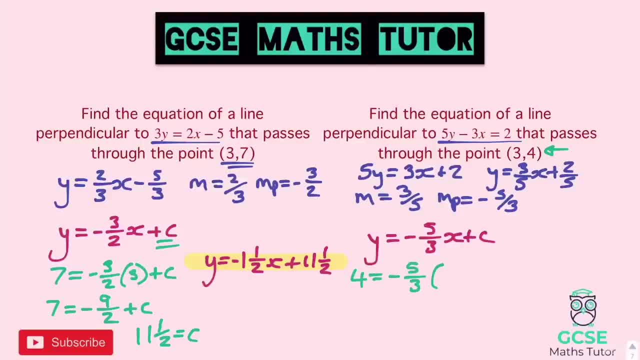 minus 5 thirds times the x coordinate there, which is 3, plus c. Let's times that out. So 4 equals 3 times 5, on the top there, remembering it's 3 over 1, so minus 15 over 3,. 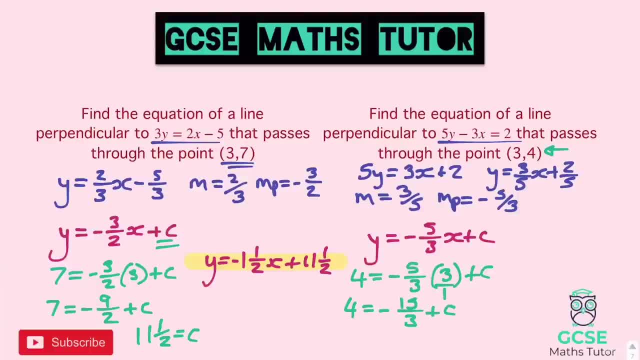 plus c. 15 does actually divide by 3, so 15 over 3 becomes 5, so we have 4 equals negative 5 plus c, and adding 5 to both sides there, we get 9 equals c, or c equals 9, and then again we can. 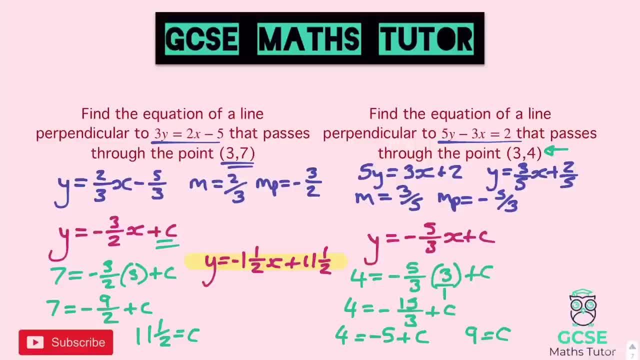 put that in place of c in our line equation. So what do we get? We get- let's write this up here- we get: y equals minus 5 thirds x plus 9, there we go, and that is our line equation. And again you could write negative. 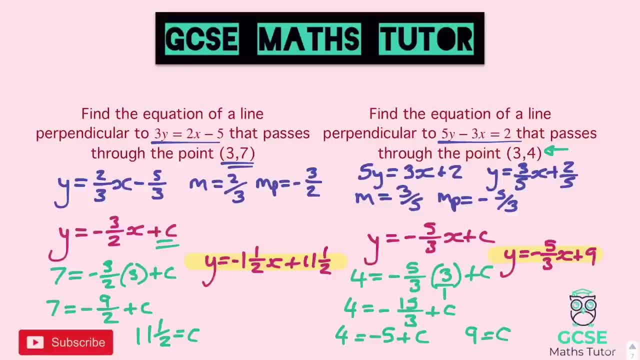 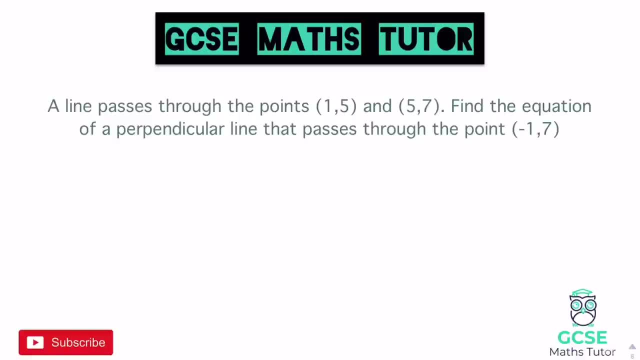 5 thirds as negative. 1 and 2 thirds- you could write that in another format if you wanted to there, but absolutely fine, just leave that as a fraction, Right? so there's those two. Let's have a look at something slightly different. Okay, so a line passes through the points 1,. 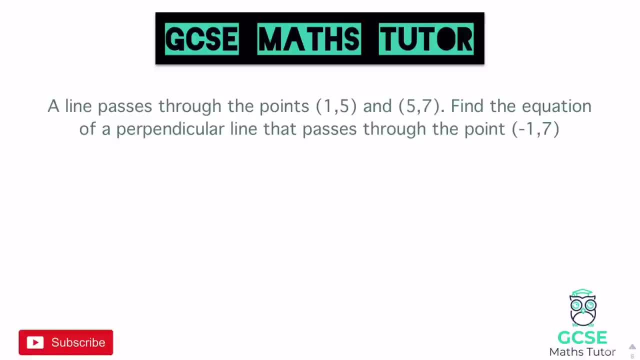 5, and 5, 7.. Find the equation of a perpendicular line that passes through the point negative 1, 7.. Now, this doesn't give us a line equation, which means we don't have a line equation, have a gradient, which means we're going to have to work one out. So we have been given this. 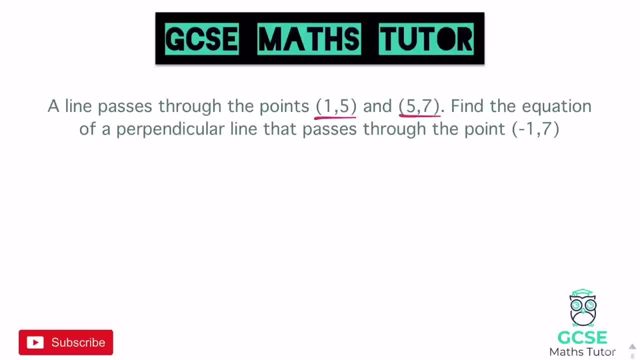 information that a line passes through these two points. Obviously, if you remember from the last video, we can have a look at the change in y over the change in x to get the gradient. so we don't even need the line equation, Because we've got these two points. we can find it ourselves. So 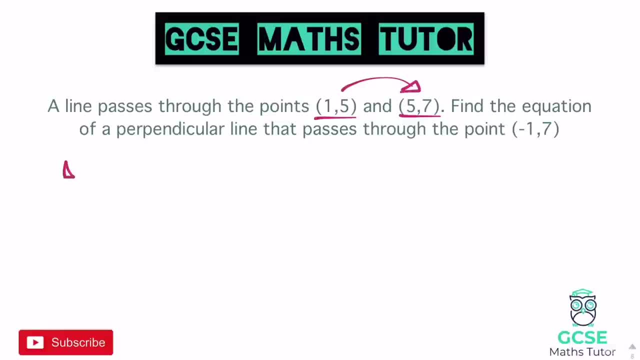 going from one point to the other, the change in y, which we're going to do over the change in x, but the change in y goes from 5 to 7, which is a change of positive 2, and the change in x goes. 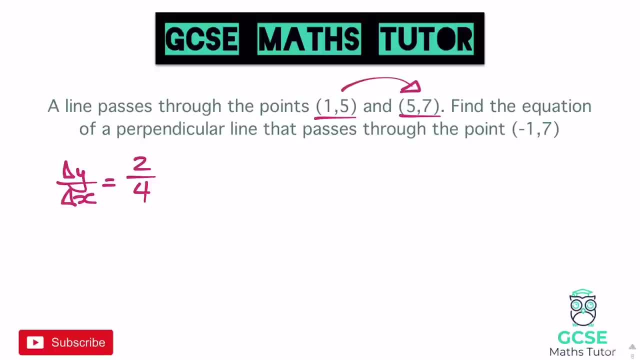 from 1 to 5,, which is positive 2, and the change in x goes from 1 to 5,, which is positive 2.. So if we simplify that down we get a half. So our gradient at the moment is 1 half. So if I want 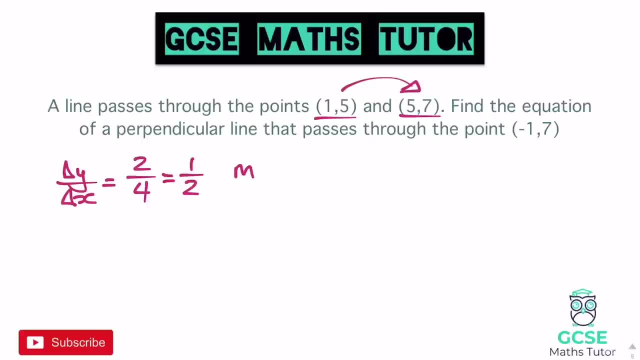 the perpendicular gradient which we do. for this, because we're looking for a perpendicular line- we'll do the negative reciprocal, So negative 2 over 1, which is negative 2.. Right, there we go, And now we can put that into our line equation. So y equals negative 2x plus c, And then again: 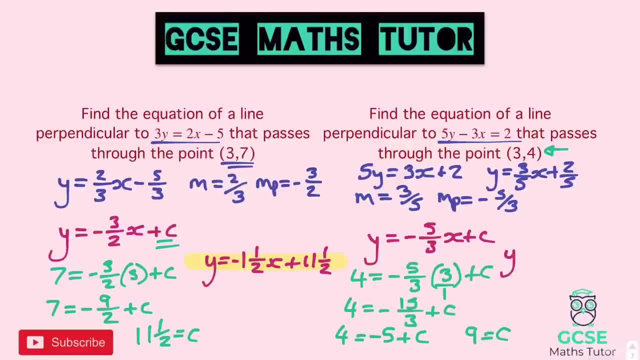 We get- Let's write this up here: We get y equals Y equals minus 5 thirds, x plus 9.. There we go, And that is our line equation. And again you could write negative 5 thirds as negative 1 and 2 thirds. 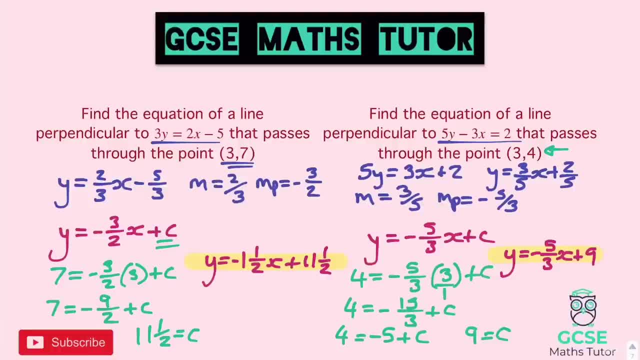 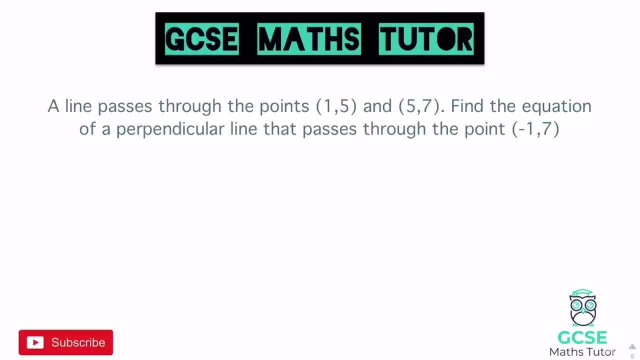 You could write that in another format if you wanted to there. But absolutely fine, Just leave that as a fraction, Right? So there's those two. Let's have a look at something slightly different. Okay, So a line passes through the points 1, 5 and 5, 7.. 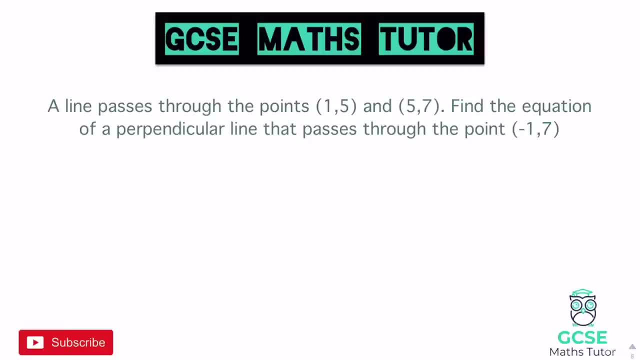 Find the equation of a perpendicular line And that passes through the point negative 1, 7.. Now, this doesn't give us a line equation, Which means we don't have a gradient, Which means we're going to have to work one out. 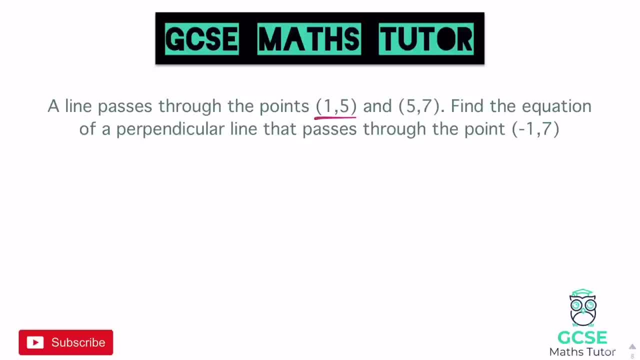 So we have been given this information That a line passes through these two points. Obviously, if you remember from the last video, We can have a look at the change in y over the change in x To get the gradient. So we don't even need the line equation. 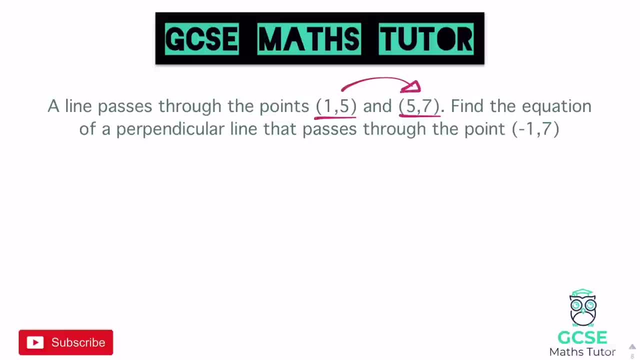 Because we've got these two points, we can find it ourselves. So, going from one point to the other, The change in y, Which we're going to do over the change in x, But the change in y goes from 5 to 7.. 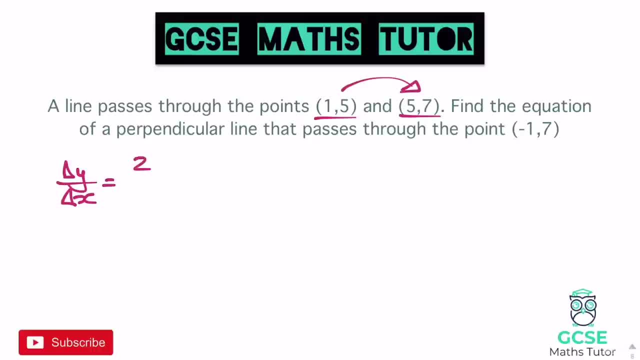 Which is a Change of positive 2. And the change in x goes from 1 to 5. Which is positive 4 or 2 quarters. So if we simplify that down We get a half. So our gradient at the moment is 1 half. 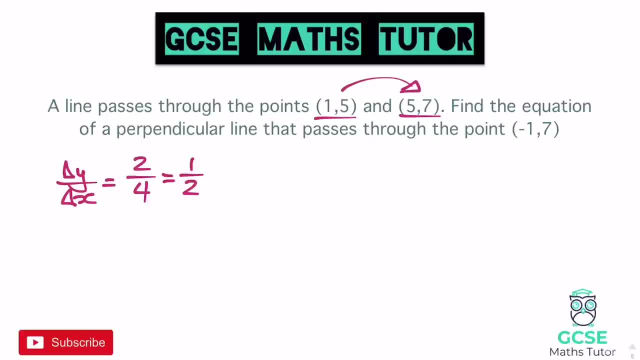 So if I want the perpendicular gradient- Which we do for this, Because we're looking for a perpendicular line- We'll do the negative reciprocal, So negative 2 over 1.. Which is negative 2.. Right, there we go, And now we can put that into our line equation. 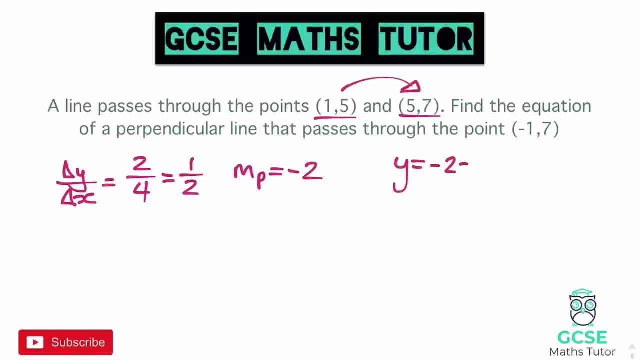 So y equals negative 2x, Which is negative 1 plus c. And then again, just like before, We're going to sub in our coordinate. So 7 is the y coordinate, Which equals negative 2 times x, Which is negative 1 plus c. 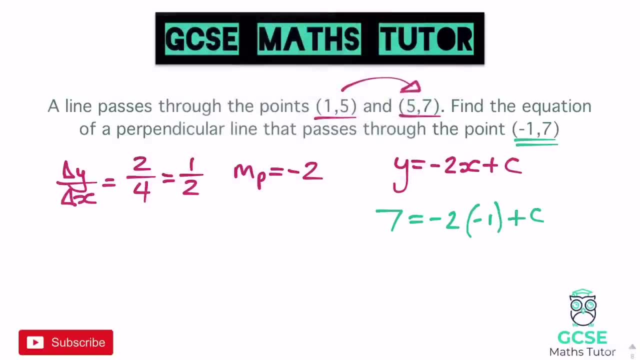 Negative 2 times negative. 1. Is positive. 2. Those negatives cancel each other out. So 7 equals 2 plus c. Solving that, Take away 2 from both sides To get c on its own, We get 5 equals c. 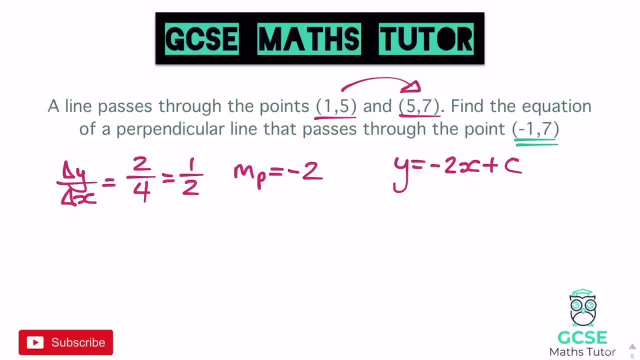 just like before, we can sub in our coordinate. So 7 is the y coordinate, which equals negative 2 times x, which is negative 1, plus c- Negative 2 times negative, 1 is positive 2.. Those negatives cancel each other out, So 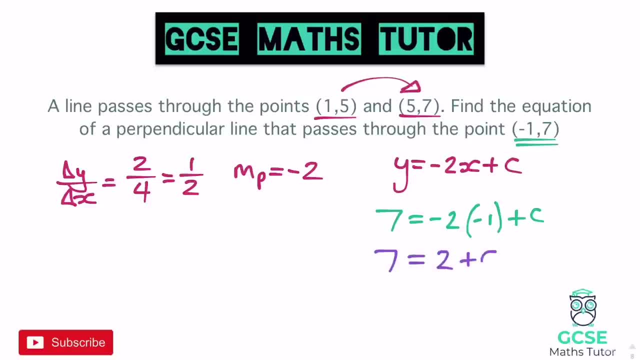 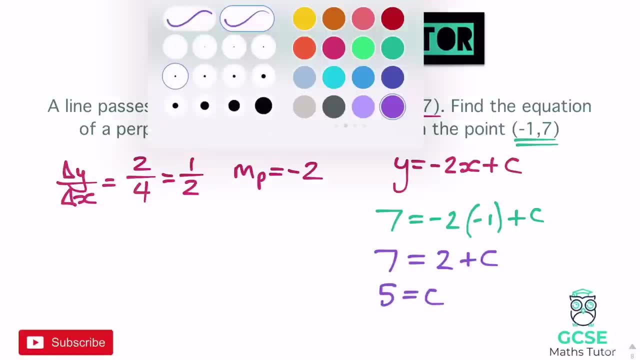 7 equals 2 plus c. Solving that, take away 2 from both sides to get c on its own, We get 5 equals c or c equals 5, and we can put that back in place of c up here. So y equals negative 2x. 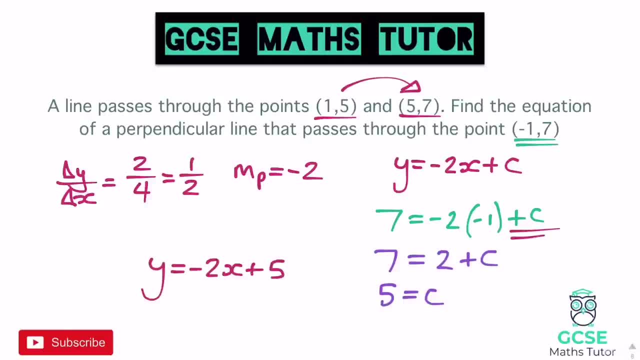 plus the 5 there. There we go plus 5.. And there's the equation of our line. OK, so for this question it's all the same process, but you're just going to have to find the gradient first. So I've got one for you to have a go at. Don't forget you change in y over. 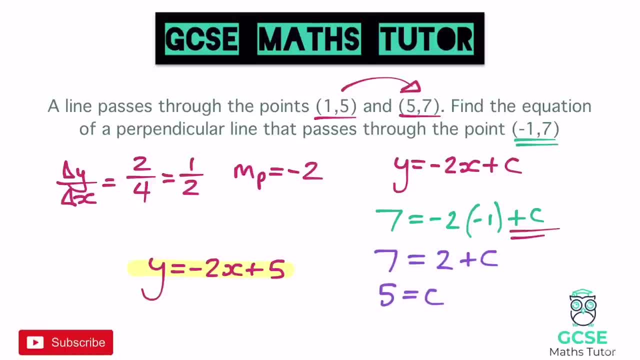 change in x. Don't forget, if you're going from one coordinate to the other, to keep that consistent with the x and the y. But here we go. Here's one for you to have a go at. OK, so here's a question. 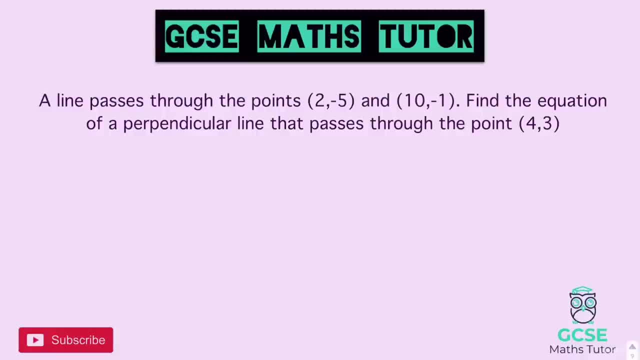 for you to have a go at. It's a pause video there. Have a go and we'll go over the answers in a sec. OK, so a line passes through these two points. So let's start off by finding the gradient. So, 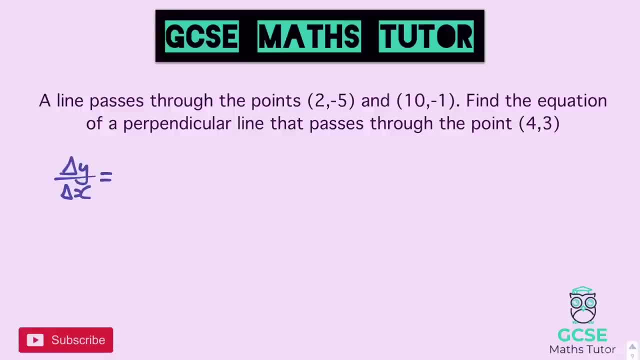 change in y over the change in x. So the change in y goes from negative 5 to negative 1. And that is a positive 4.. It's going up 4 from negative 5 to negative 1. Then from 2 to 10 for the x. 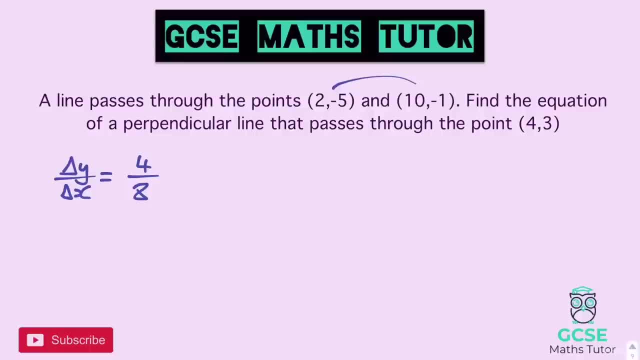 coordinate, that is 8. There we go, 4 over 8. And if you simplify that down you get 1 over 2. So you get a half again for this one. So our perpendicular gradient, flip it over, put it. 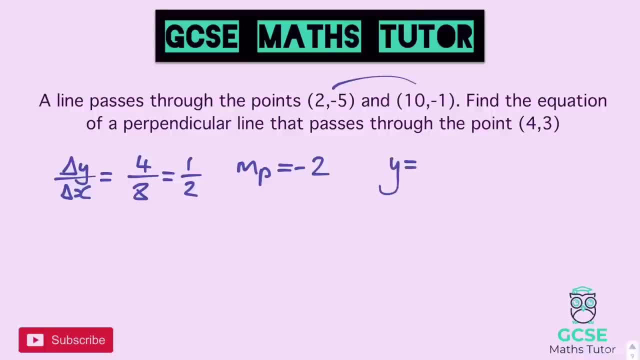 in And we can actually put this now into our line equation. So y equals negative 2x plus c. Now we can put in our coordinates there. So we've got 4, 3 to stick in, So 3 in place of y, So 3 equals. 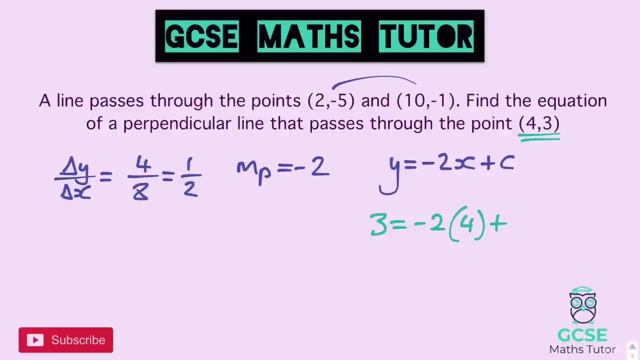 negative, 2 times 4 plus c. Expand that out, So 3 equals negative, 8 plus c. And then, solving that for c, add 8 to both sides. We'll get 11 equals c, or c equals 11.. And then, finishing it off, 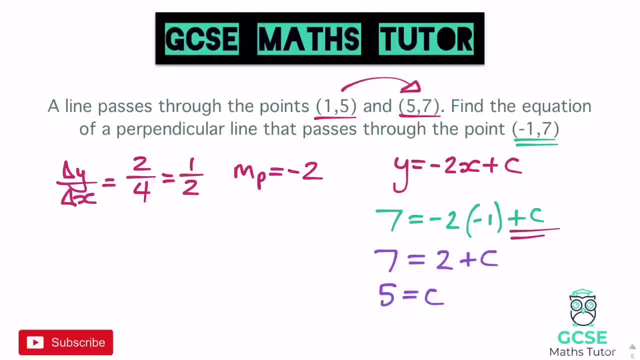 Or c equals 5.. Taking place of c up here. So y equals negative 2x Plus the 5. there, There we go, Plus 5. And there's the equation of our line. Okay, so for this question It's all the same process. 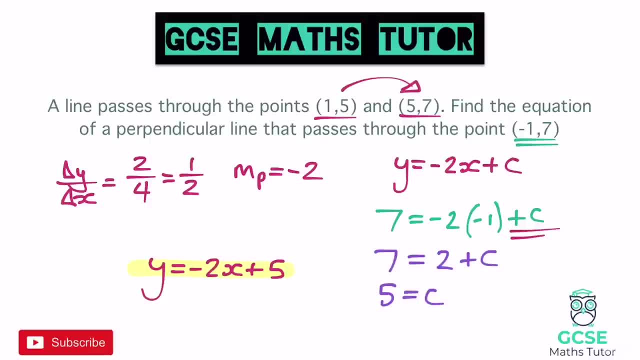 But you're just going to have to find the gradient first. So I've got one for you to have a go at. Don't forget you're changing y over changing x. Don't forget if you're going from one coordinate to the other. 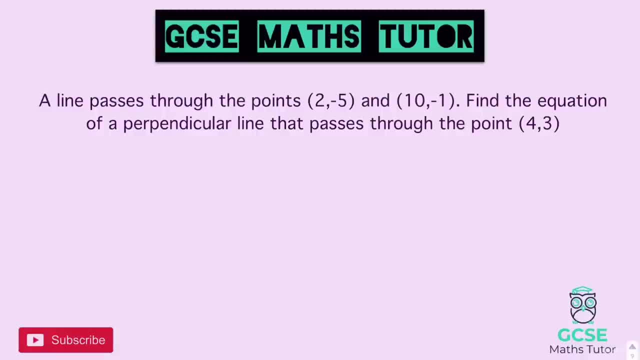 To keep that consistent with the x and the y. But here we go. Here's one for you to have a go at. Okay, so here's a question for you to have a go at. We'll go with the answer in a sec. 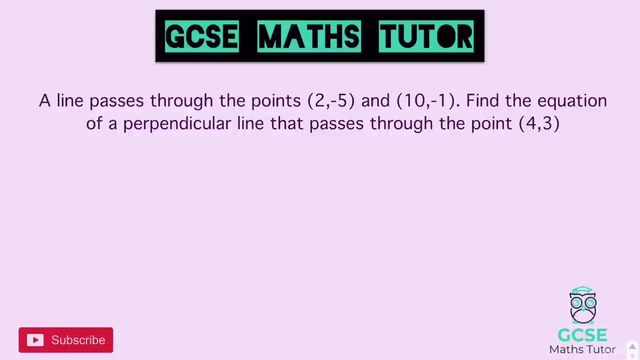 Okay, so a line passes through these two points. So let's start off by finding the gradient. So changing y Over the change in x, So the change in y Goes from negative 5 to negative 1.. And that is a positive 4.. 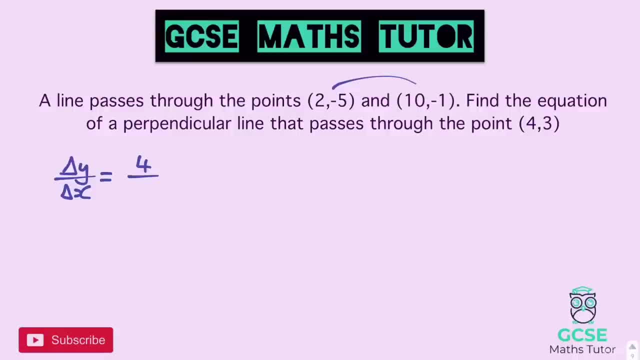 It's going up 4 from negative 5 to negative 1.. Then from 2 to 10 for the x coordinate, That is 8.. There we go, 4 over 8. And if you simplify that down, You get 1 over 2.. 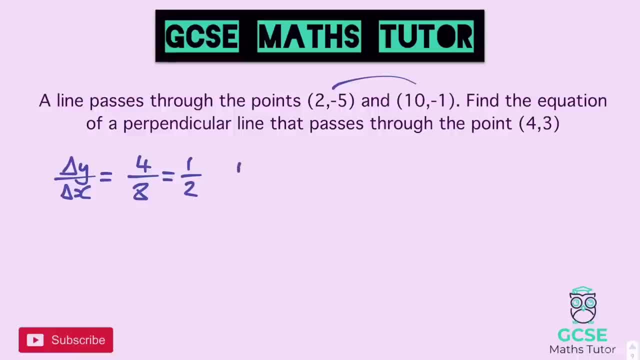 So you get a half again for this. So our perpendicular gradient: Flip it over, Put it with a negative, Negative 2. And we can actually put this now into our line equation. So y equals negative 2x Plus c. 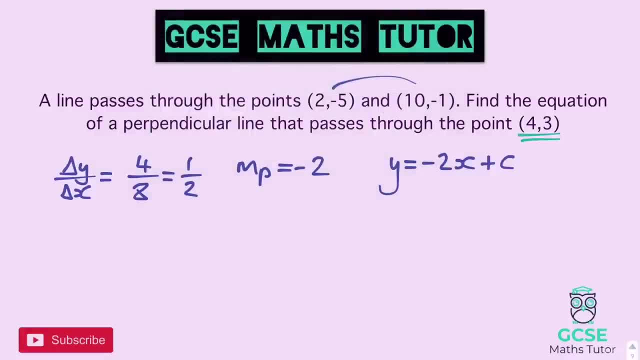 Now we can put in our coordinates there. So we've got 4, 3 to stick in. So 3 in place of y. So 3 equals negative 2 times 4.. Plus c. Expand that out. So 3 equals negative 8 plus c. 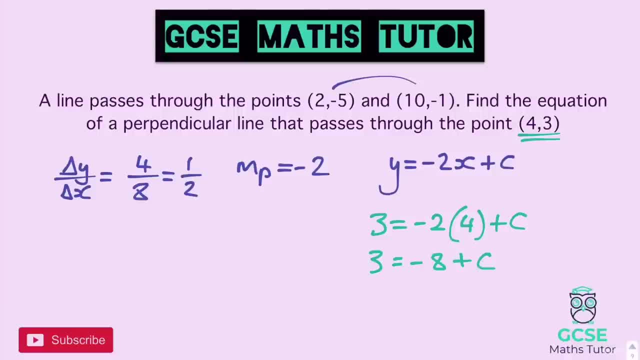 Expand that out And then, solving that for c, Add 8 to both sides, We get 11 equals c, Or c equals 11.. And then, finishing it off Just like before, Putting it in place of c, there, We get y equals negative 2x. 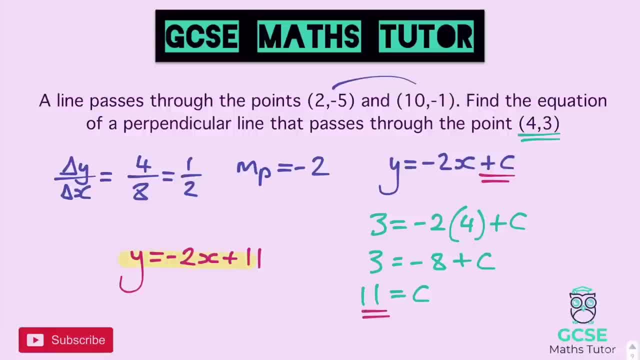 Plus this 11 here. Right, there we go, And there's the equation of the line Right, I've got one more question for you to have a go at before we finish, Just sort of putting all this together and seeing what you can do. 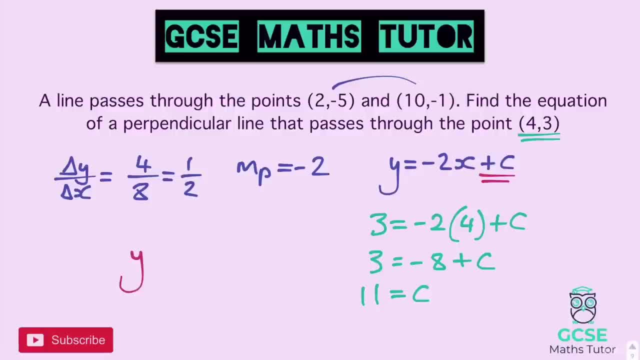 just like before putting it in place of c. there we'll get y equals negative 2x plus this 11 here. Right, there we go, And there's the equation of the line. Right? I've got one more question for. 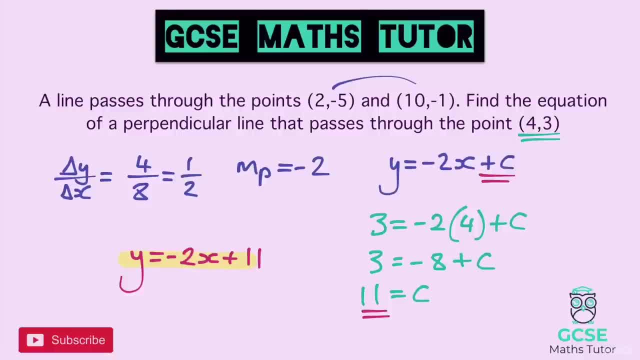 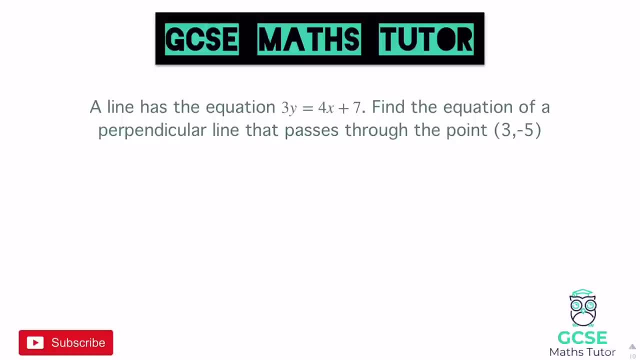 you to have a go at before we finish, Just sort of putting all this together and seeing what you can do. Let's have a look at it. Okay, so this is the last question here. There's nothing that we've not done throughout the video to actually be able to answer this, But it might be a good. 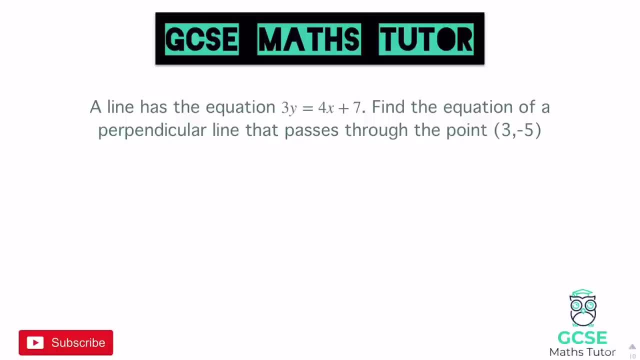 idea for you to just pause the video there. have a go see what you get and we'll go over the answers in a sec. Okay, so hopefully you've had a go at that question there. Let's have a look. It says: 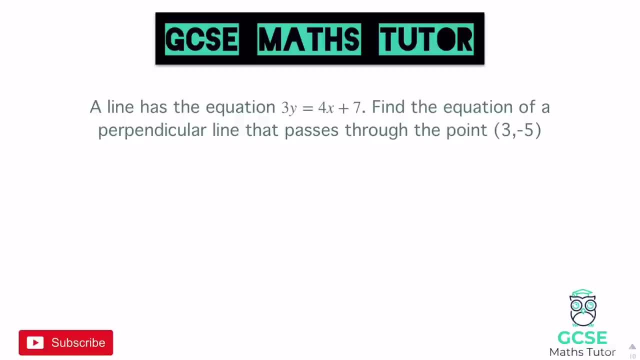 here's the line equation: Find the equation of a perpendicular line that passes through the point 3, negative 5.. So we've got the line up here. 3y equals 4x plus 7.. So we're going to have to get. 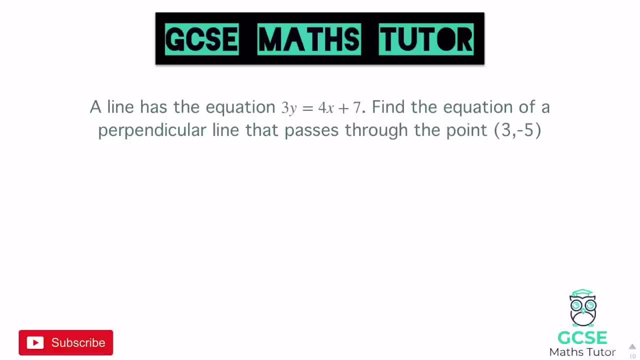 that in the form y equals. So let's divide everything by 3, okay, So that's the first step. Divide by 3.. So if we do that, we get y equals 4 thirds and we divide that by 3, x plus 7 thirds. 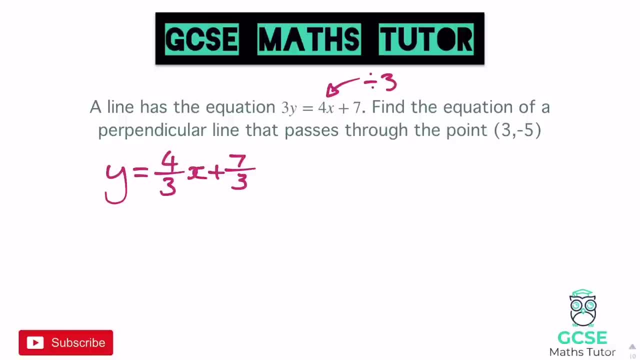 dividing everything by 3.. So that's the first step. So we've got the line up here, So we've got the, I think, by 3 there, And then we've got our gradient. So our gradient of that line is 4 thirds. Now we can find the perpendicular gradient. So flip it over with a negative. 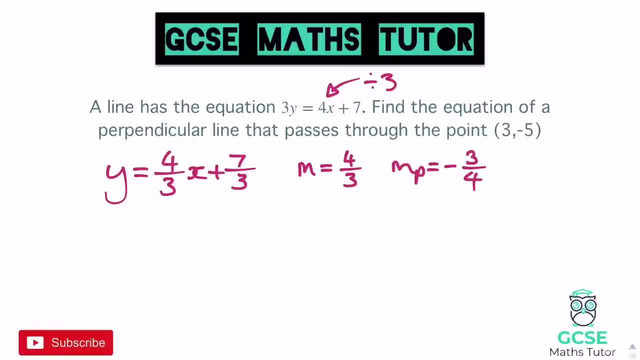 negative 3 quarters. And now we can just take that same approach that we have on all the previous questions. So sticking our gradient into our line equation, we get y equals negative 3 quarters, x plus c, And then we can put our coordinate in, and our coordinate there is: 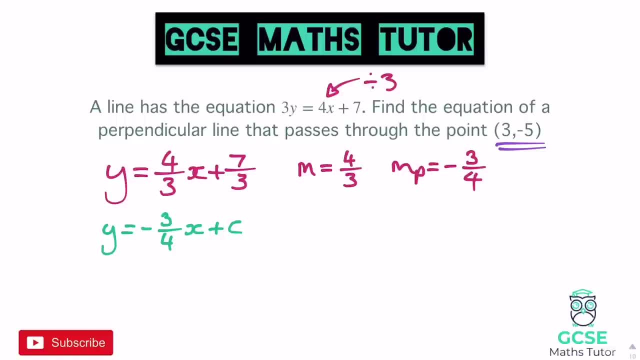 3, negative 5.. So minus 5 in place of y. So minus 5 equals negative 3 quarters times 3 plus c. Expand that out: So minus 5 equals 3 over 1 times 3 quarters, is negative 9 quarters. 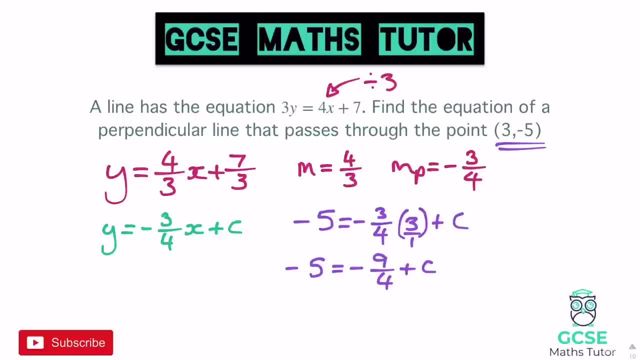 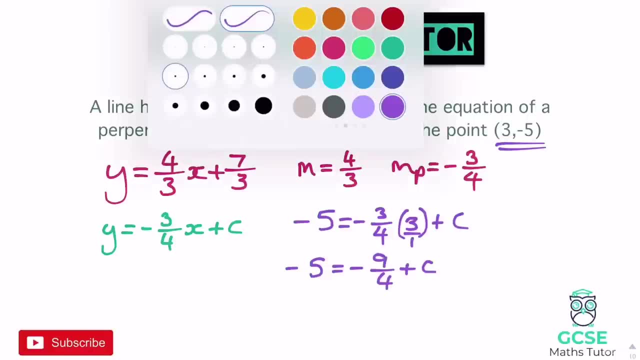 plus c, And then we need to add 9 quarters to the other side. Again, this is one of those scenarios where I would look at this as a mixed number. So if we convert that into a mixed number, let's do that to the side, Minus 9 quarters. 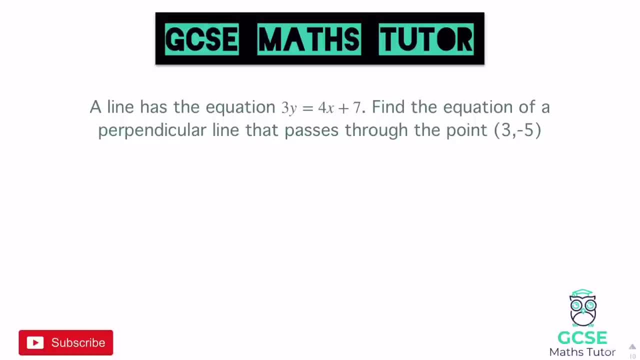 Let's have a look at it, Something that we've not done throughout the video To actually be able to answer this, But it might be a good idea for you to just pause the video there. Have a go, See what you get. 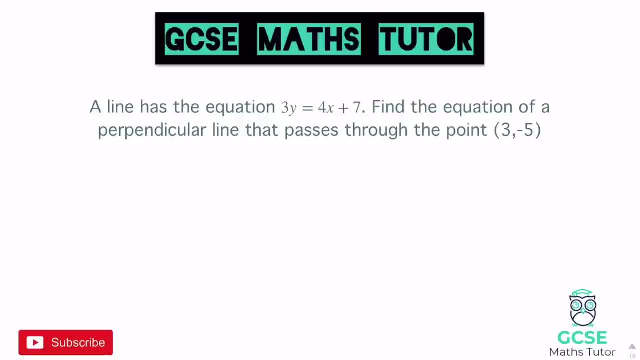 And we'll go over the answers in a sec. Okay, so hopefully you've had a go at that question there. Let's have a look. It says: here's the line equation: Find the equation of a perpendicular line that passes through the point. 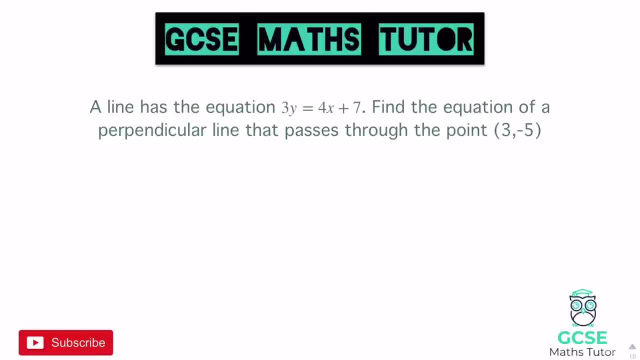 So we've got the line up here: 3y equals 4x plus 7.. So we're going to have to get that in the form y equals, So let's divide everything by 3.. Okay, So that's the first step. 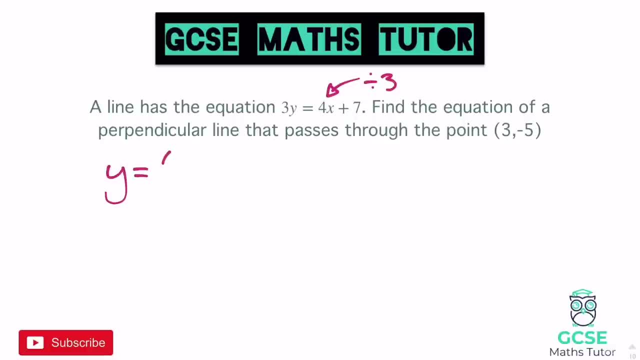 So if we do that, We get y equals 4 thirds And we divide that by 3.. x plus 7 thirds, Dividing everything by 3 there, And then we've got our gradient. So our gradient of that line. 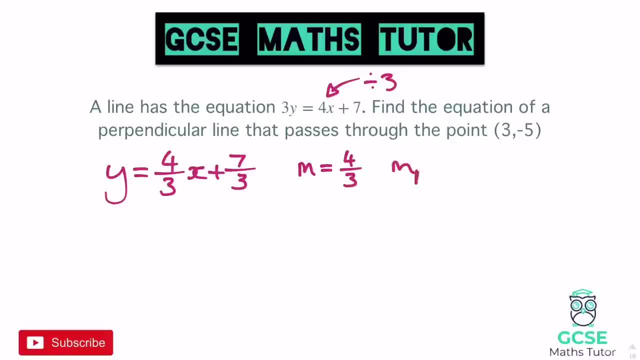 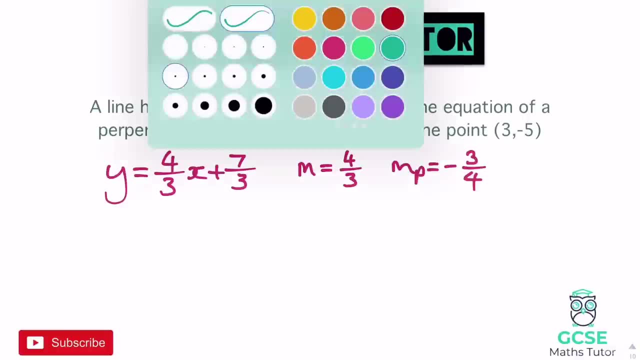 Is 4 thirds. Now we can find the perpendicular gradient. So flip it over with a negative, Negative 3 quarters, And now we can just take that same approach that we have on all the previous questions, So sticking our gradient into our line equation. 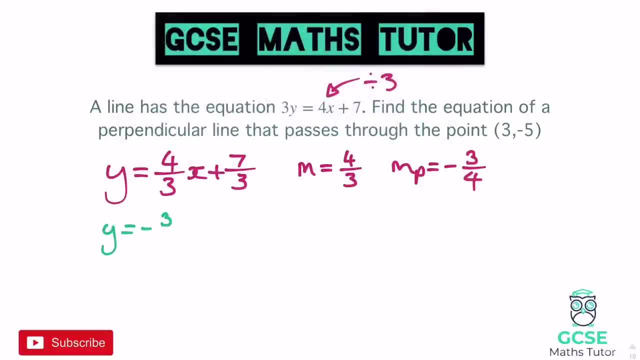 We get y equals Negative 3 quarters x plus c, And then we can put our coordinate in And our coordinate there is 3 negative 5.. So minus 5 in place of y. So minus 5.. Equals Negative 3 quarters. 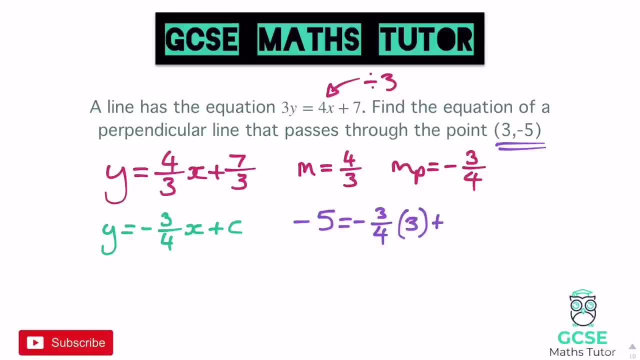 Times 3. Plus c. Expand that out. So minus 5 equals 3 over. 1 times 3 quarters Is negative. 9 quarters Plus c. And then we need to add 9 quarters to the other side. 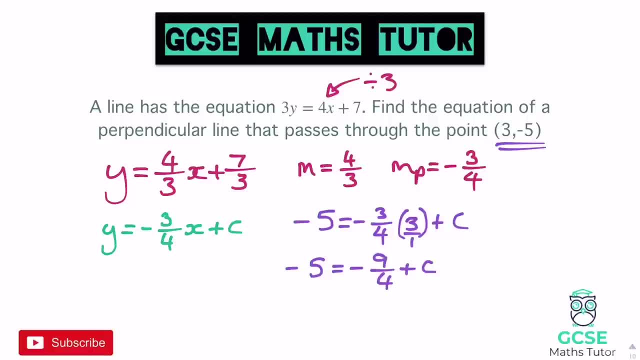 Again, this is one of those scenarios where I would Look at this as a mixed number. So if we convert that into a mixed number, Let's do that to the side. Minus 9 quarters Is the same as Minus 2 and a quarter. 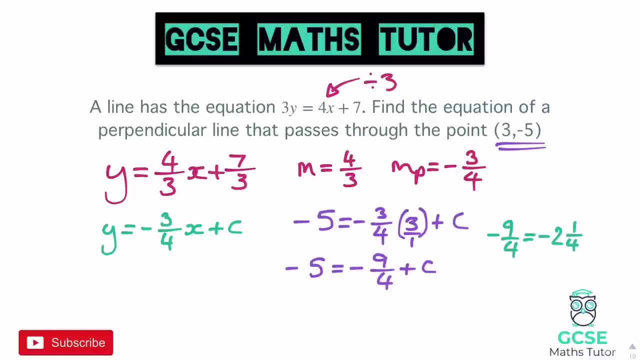 4 goes into 9 twice. So minus 2 and a quarter. So if we add 2 and a quarter over to negative 5.. We need to just be able to work that out there. So if we add 2 to negative 5..